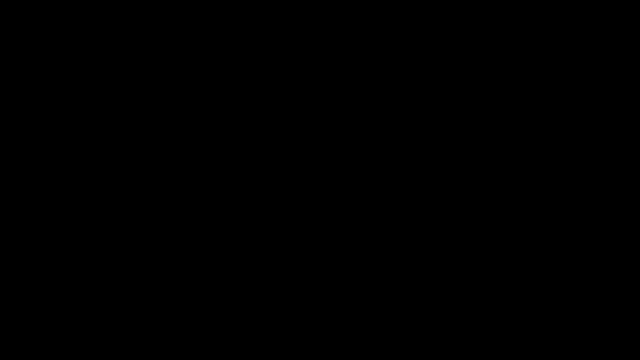 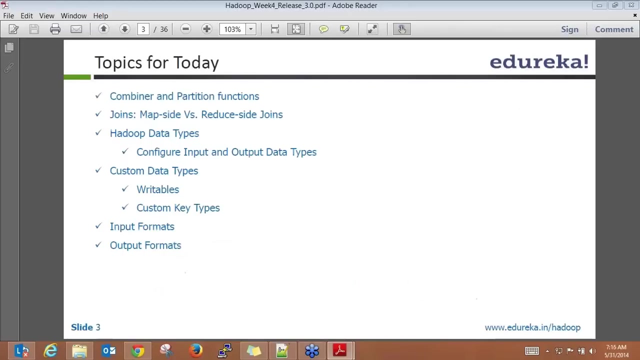 Today we are going to start with the advanced MapReduce concept, and these are the topics for today. So today what we are going to do is we are going to build on whatever the concept we learned in the previous class and along with that, we will learn some of the common. 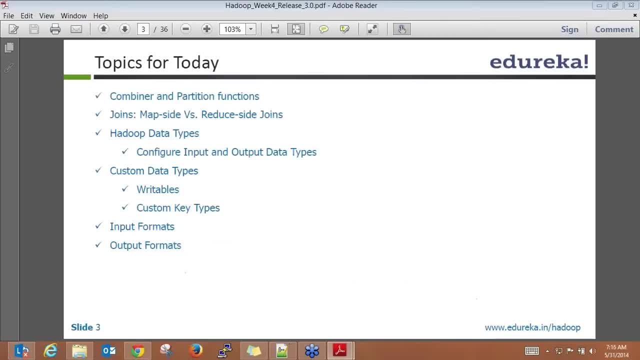 thing which, as a developer, you have to be aware in terms of the MapReduce developer, So few of the common scenario, like in the previous class. also, people have the question like how to redirect your output, like the reducer, how the reducer works, kind of things. 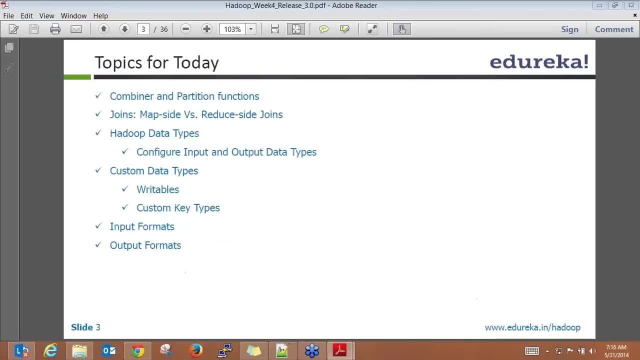 And then, like one of the critical thing, when you will go for this data processing by using the Hadoop framework, it will be like how to do the join. So we are going to see about, like in MapReduce, if you have to do the join, if you compare to SQL, you just write a join. 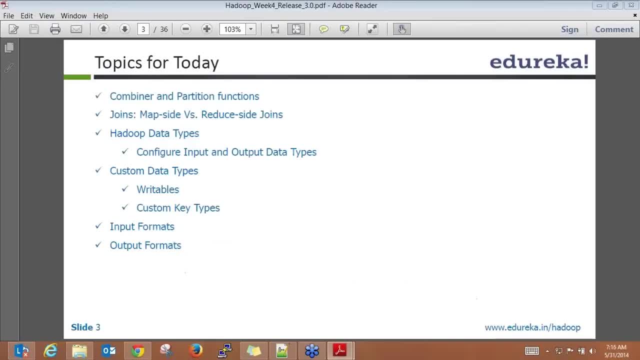 statement and you are able to do that. But when it comes to the MapReduce it is more involved kind of the join, where you as a programmer need to take care of all the aspects of the join, like how you read data, how you face the column and all those things. So let's 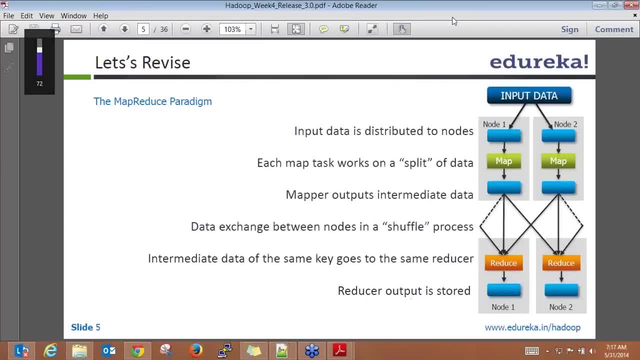 get it started, guys. So how the MapReduce framework work, guys, is you have the input data and whenever you want to run MapReduce code, then that first thing, what you will do, is you will bring that data inside the HDFS. and that's the two main components we have in the whole Hadoop learning or whatever. 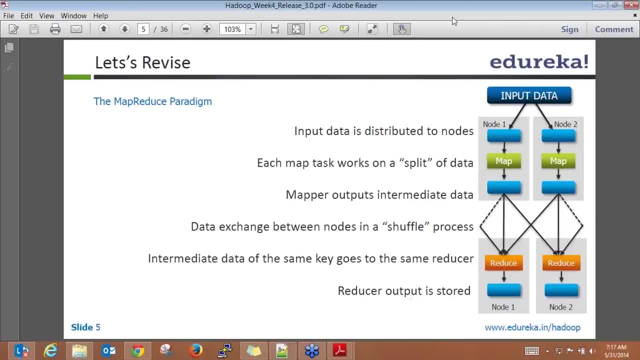 we are discussing about the Hadoop framework. One is Hadoop file system and then the MapReduce, which you run on top of the HDFS. So now to run the MapReduce, what you have to do is you. you have to first bring the data inside the Hadoop. so whenever you bring any data inside, 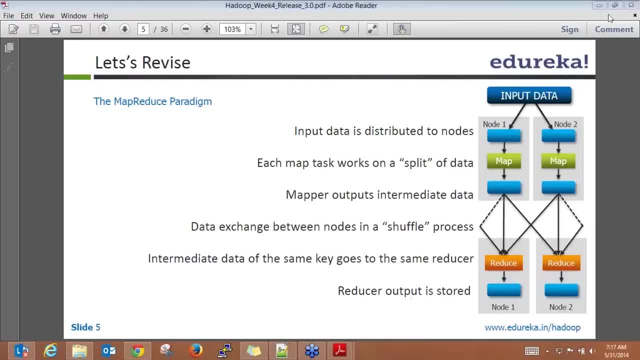 the Hadoop, the data gets distributed across multiple nodes. and once the data is distributed across the multiple nodes, what happens is, like you know, the data gets divided on the level of the block. so you have a block size configuration, if you guys remember the configuration. 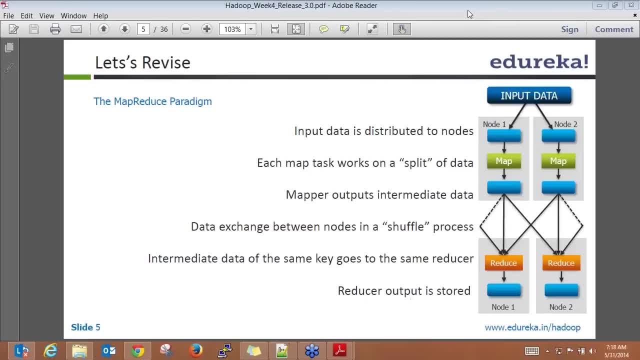 files. we see right where, in the hdfs-sitexml, you can specify what is the block size- so generally 64 MB or 128 MB- and based on that, your data will get divided across multiple machines and each of the block will be replicated across multiple copies in the cluster based. 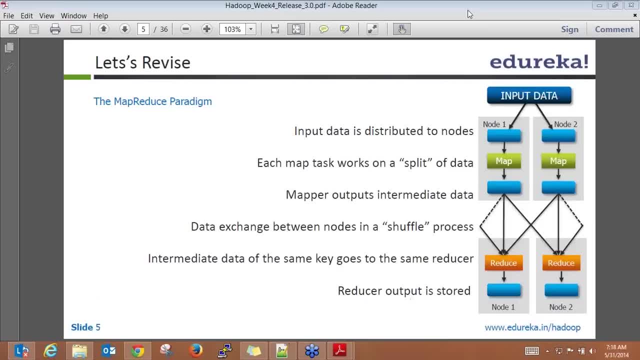 on the replication factor which we set inside the cluster. so, by default, the replication factor is the 3, and based on that the data will get replicated across multiple machines. So this reliability, automation, Now this duplication of the data which you see in the cluster, it is on the block level. 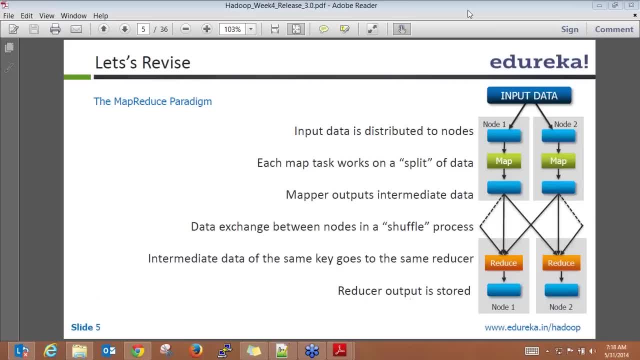 not on the file level. so every time you will have each block which will represent on the three different machines. so if one machine goes down, you can still access it from the other machine and you can continue with the processing. So that's where the data comes inside the node and it gets distributed across the node. 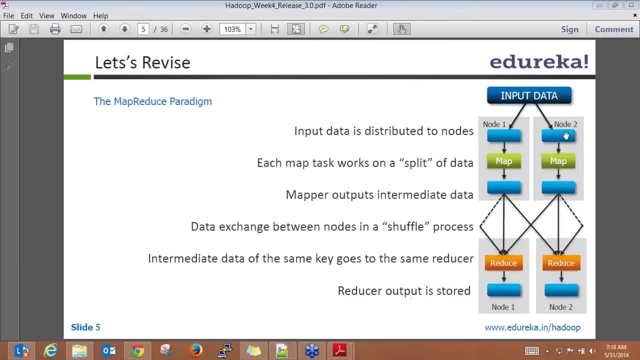 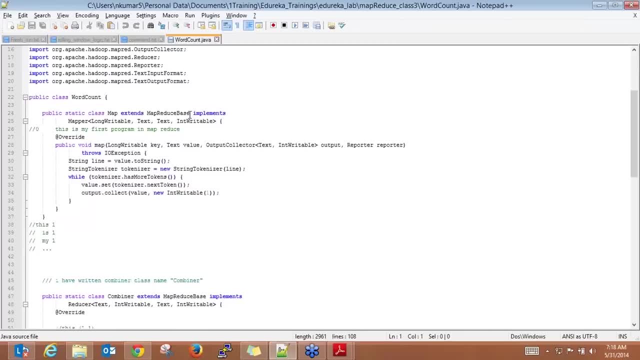 and once you have your data distributed across the node, what you do is you write your MapReduce code. Hope you guys remember this particular code. Thank you, This is the same thing which we wrote in the previous class, where you take an input path. 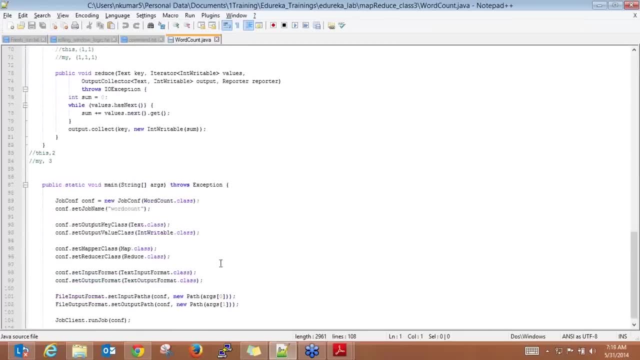 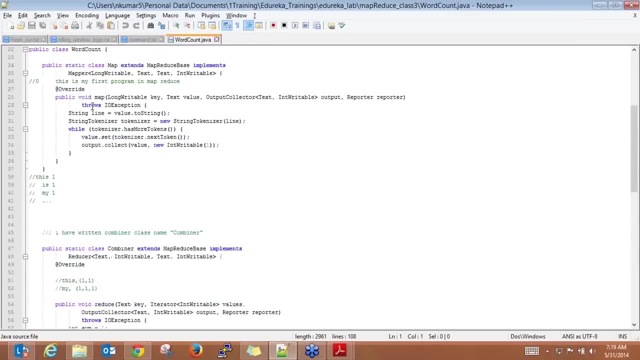 and you take an output path where you want to store the data. you write the logic how to read the data. so basically, you get the input data, you split it based on how you want to tokenize the whole input data set. so for each new line you take as one particular 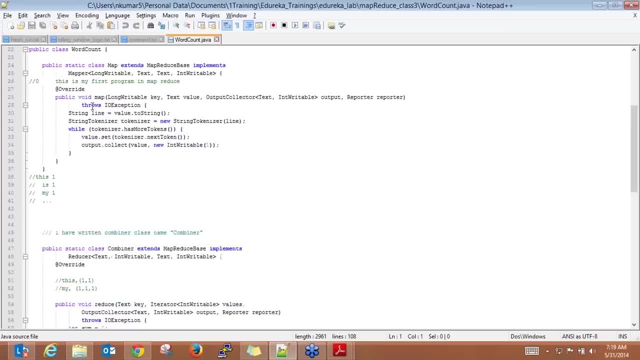 record key and value pair and for each of the line you divide each word separated by space, so you divide it in a different word, And for each word you want to count it like how many times it has occurred. so this is: 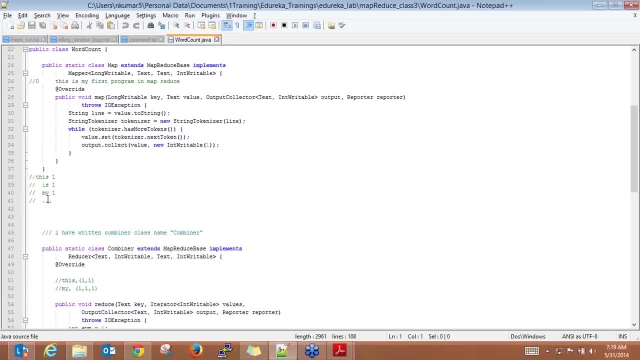 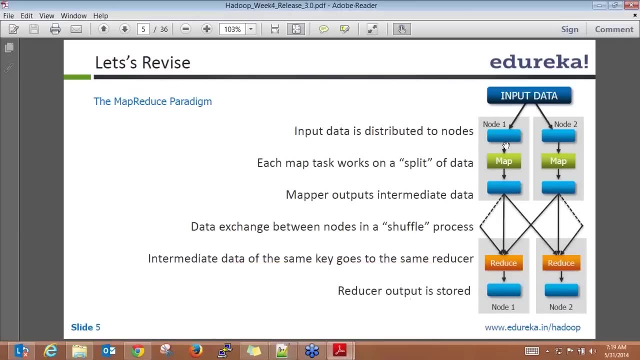 the like: if the input is- this is my, so you want to count, like how many times each word has occurred in a given input data set. So that particular thing goes like for the MapReduce program to process that. so the input data set goes to the mapper and mapper first what it does in the stage one. it just 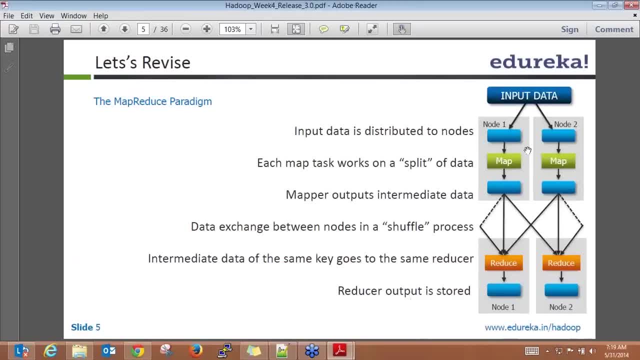 does the mapping where it says that: okay, each word has. whenever it sees a particular word, it will just mark it as that word. Okay, So that's the key value pair it will output and that you will connect in the output collector. 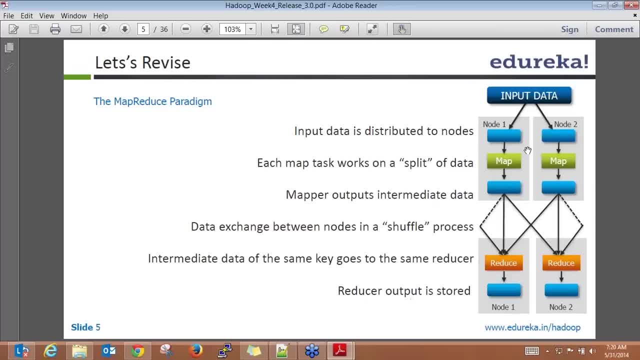 And once you have all this data coming out from the mapper, it's good that it has processed all the data, but that's not the final objective which we want to access. So what we want to do is like we want to, we want to, you know, get the final count. 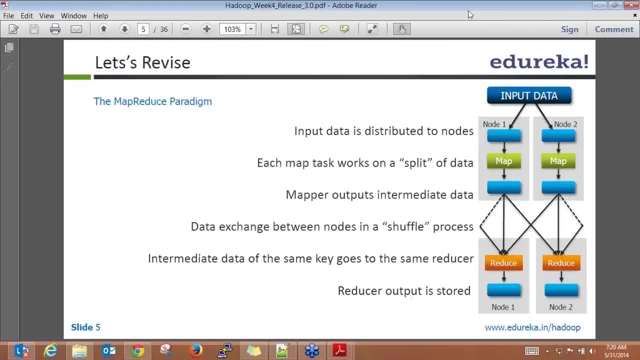 and you know we want to find out. find it out like how many times each word has occurred inside a given input data set. So to do that, what we have to do is we have to bring all the data set for that particular 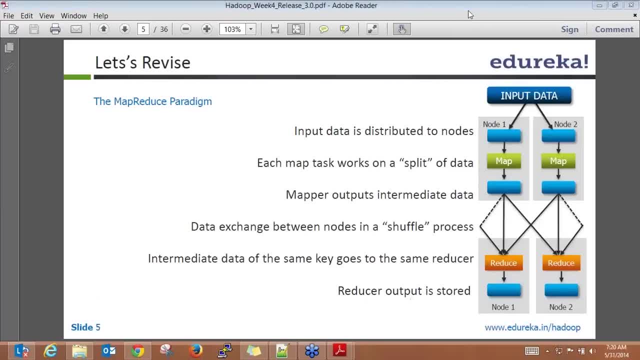 word together so that we can do the count, Like: suppose, if this has occurred three times, you want to make sure that all this, this, like this one, this one and this one three times, whenever it gets processed inside the map, it has to come to the reducer so that we can aggregate it or we can count it, and 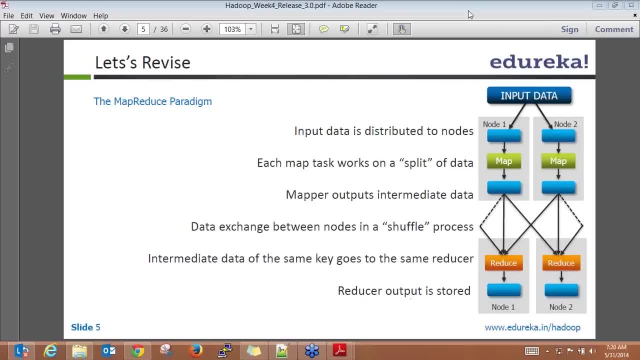 we can get the final sum Okay, Because what you have to do is you have to basically move your data from the mapper to the reducer so that it can do the aggregation, And while moving the data from mapper to the reducer, you have to make sure that all of 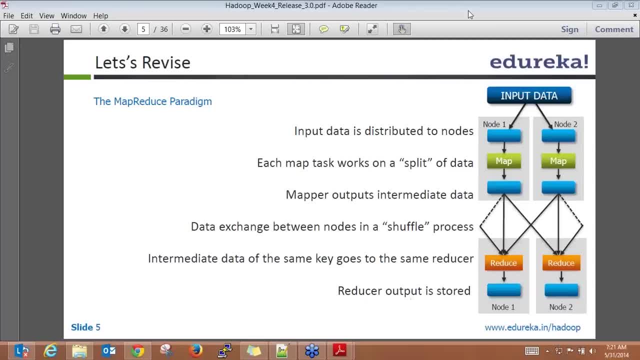 the input data set for a given key should go to one particular reducer, And the reason why you have to basically go for this particular approach is because whenever you are using the reducer, It's going to do the aggregate or the sum of whatever the input data set you have. 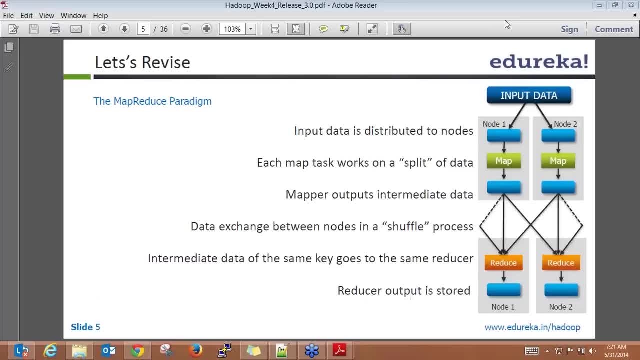 Now to get the final picture, you have to have all the key value there for a given key available to the reducer so that it can do the final aggregation Now in a distributed framework. how you basically enable this kind of the processing is you use the concept of something called the partitioner. 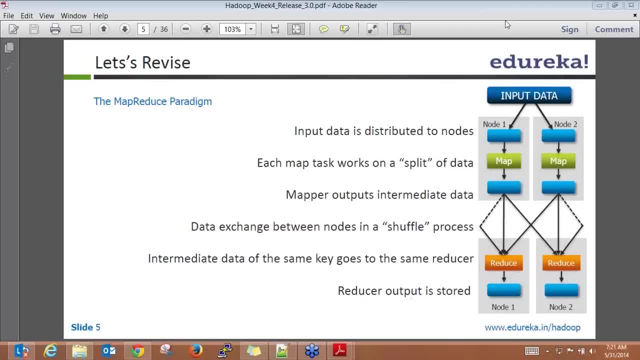 So partitioner is something by using which you will basically put a framework which will determine that whenever a output coming from the mapper, it will have a different function, It will have a particular logic and, based on that logic, every time that mapper output will go to a particular reducer. 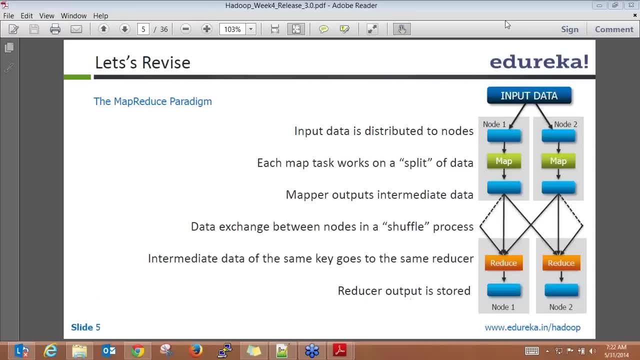 So in general, by default implementation is the hash partitioner. So whatever the key you are using, for that key there will be a hash value calculated And based on that particular hash value you will move that data set, move that particular key and value pair to one particular reducer. 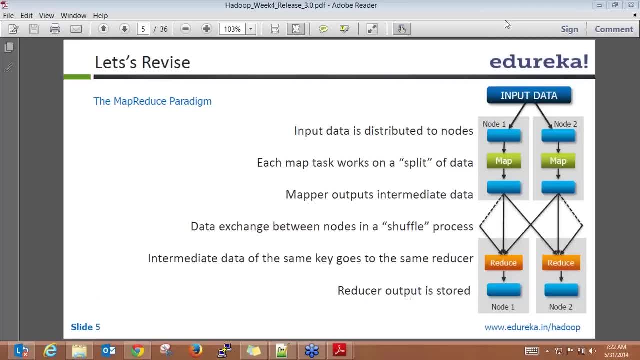 So you can think of like, suppose if you have the four reducers, so normal like, think of like hash partitioner, like, suppose it is implemented as a modular function. So you will divide whatever the key value you are getting. you will take a modular by. 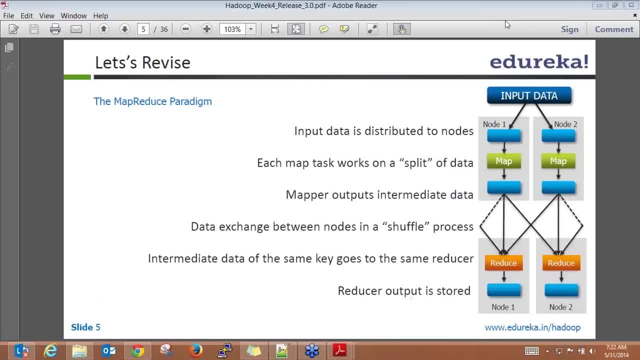 four and based on that you will get a number between zero to three. And whenever you get a number you will assign that particular key value pair to that particular reducer. So that's the process. It is called the shuffling phase. This is where you move the data from the mapper to the reducer. 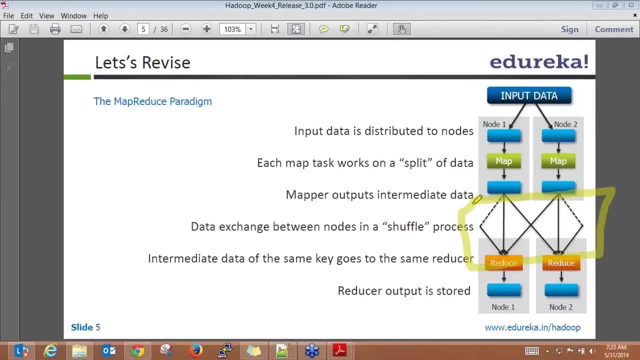 And this is the only phase where, in the whole framework, where you are going to basically move the data or move the data across the network. So that's the phase called shuffling phase, where you are going to move the data And once all this, the movement of the data, happens between the mapper and the reducer. 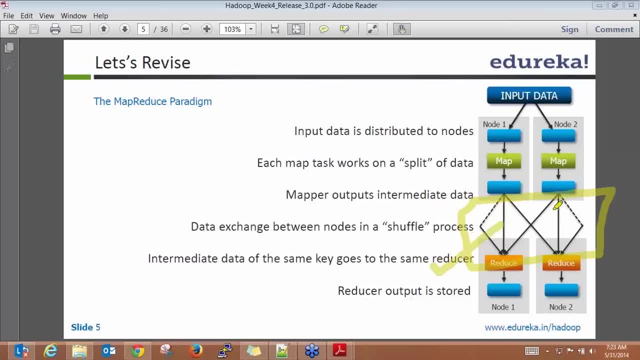 then the reducer comes in. You know the execution because it needs all the data set from the mapper to start execution. So once the data set is available to the reducer, it starts processing that input data set. And once you get the data processed by the reducer, the output of each of you know. 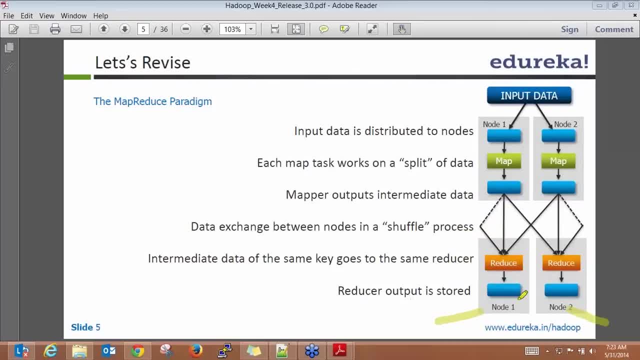 these reducer, it will go into a separate file. And the reason why? suppose if you are using five reducers, so you will get five different output file and in case, if they have the data right, so five different output file you will get inside the output. 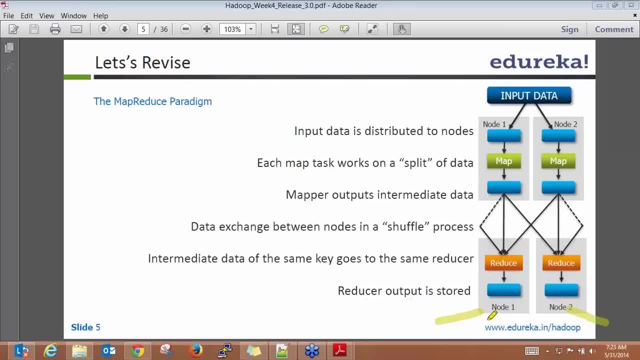 You will get the output directly, where each reducer will write in its own file. And the reason we have this kind of the architecture, where everything runs independently, is because you don't want to have a communication overhead between the two process, because that becomes costly in terms of the time it takes and also to maintain the state. 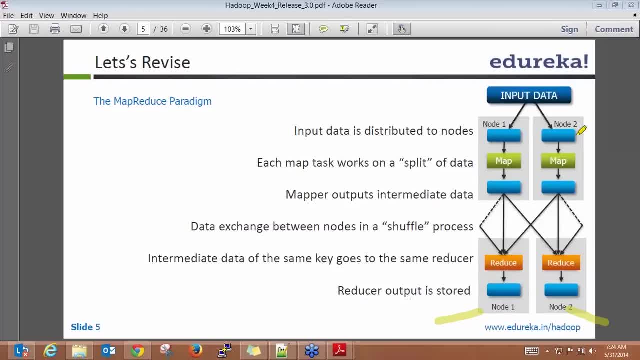 So one thing we have to understand in like the MapReduce program is like you put your algorithm or you put your logic in such a way that it can run independently. So if you have to share the state or like between one process, one phase, like one mapper, 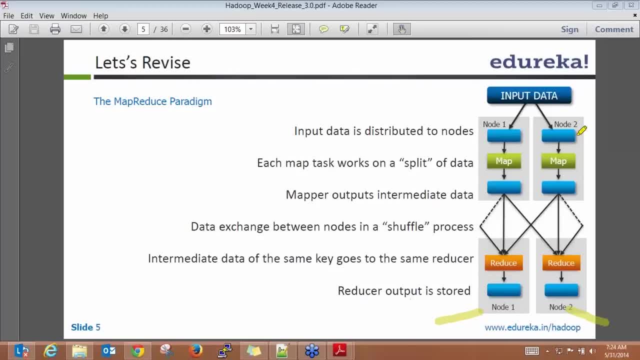 has to communicate to other mapper. so those kind of the framework, those kind of the algorithms will not be suitable for the MapReduce, because here mapper works independently, reducer works independently, right, Only communication happen between the mapper and the reducer. So apart from that phase, whole processing has to happen in parallel. 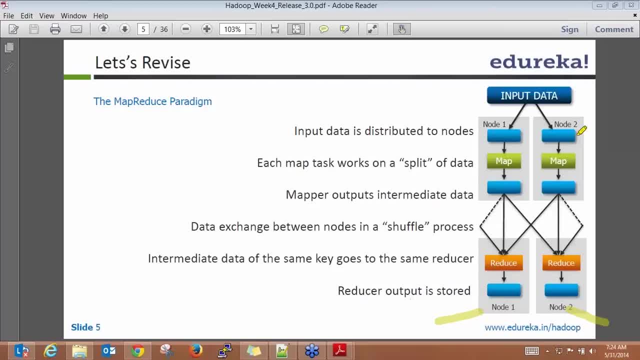 So if you have any kind of algorithm which will not be able to fit in this particular framework, in that case you will not be. you will not be able to use this MapReduce framework And that's why we have some of the limitation where you know some algorithms cannot be. 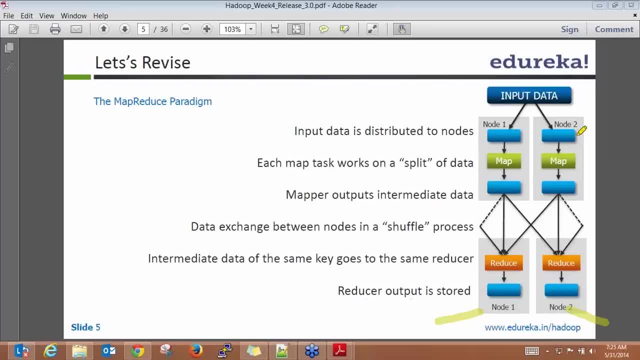 expressed as a MapReduce program, like if you are doing some graph processing or something. So for those kind of algorithms we're not. we were not able to put into a like this whole MapReduce kind of architecture. Okay, Let me see a couple of questions here. 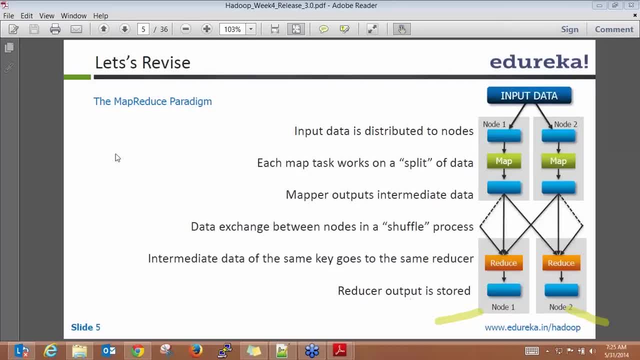 Okay, Okay. So Hitesh says: does the partitioner come in picture in the pseudo-distributed? I think you mentioned? partitioner plays the role of this in the distributed mode. So yeah, if you have multiple reducer, Hitesh, there it comes in and in this pseudo-distributed. 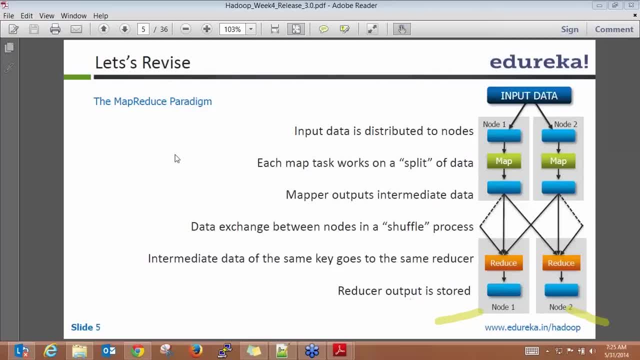 mode also, you can simulate. you know these kind of things. So it does come in picture. Meenu has doesn't all. Okay, All output from the reducer must get aggregated for the final result. I see there is a node one and node two. 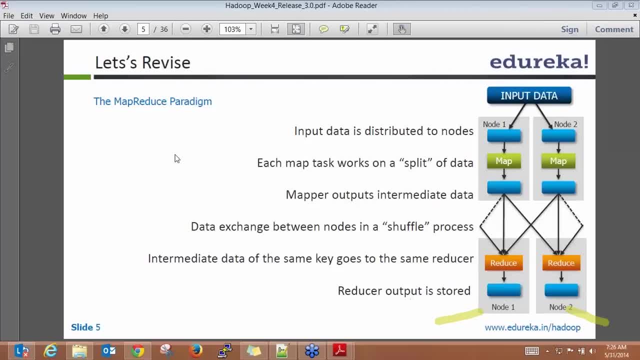 So a user needs to write another reducer for outputting the final result. Okay So, okay. So how it happens this particular thing, what you are seeing here, it's just to see you that one particular file, another Okay. 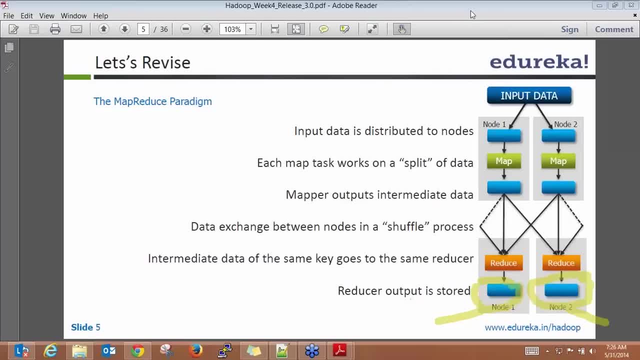 After that, what happens? Each of these file? again, it will go through this Hadoop write process where it will like. you will provide a location, the directory location, And there the file you will create. So all these three files will be accessed in that particular directory. 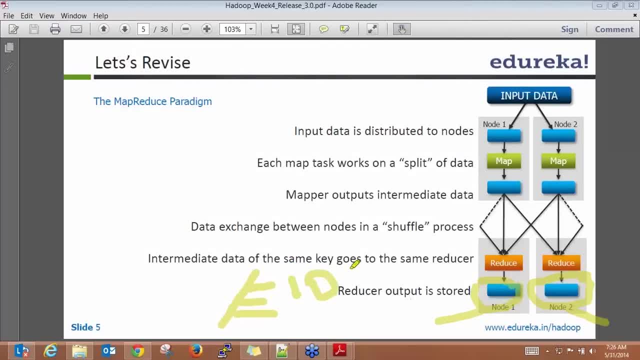 And these files suppose again, if suppose, if it is like a hundred GB file, it is coming from the reducer. So again, this file will get distributed across different blocks inside the Hadoop. So all those things, concept is still remains same, how the files are going to be stored. 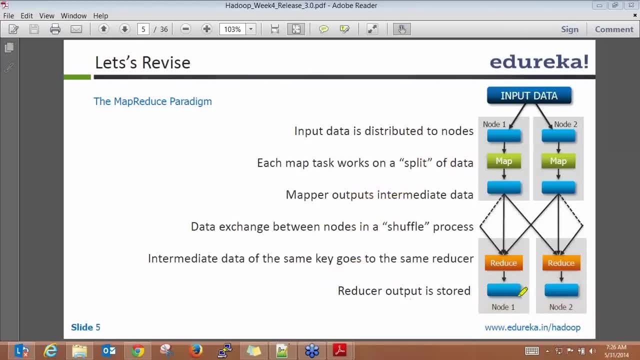 inside the cluster. So those things are still remains same, you know, in terms of how the storage will be there. Here, just to denote that each of the reducer is working independently And you know, on each of the node and giving it the output. 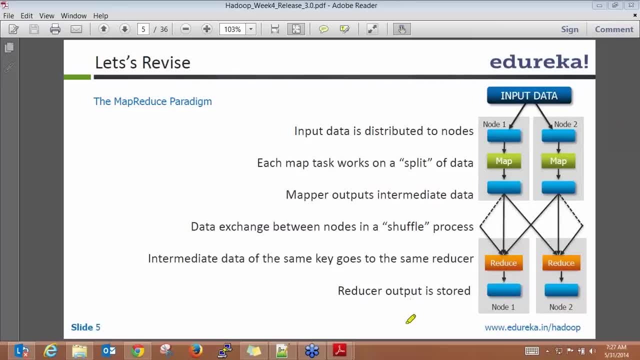 Okay, But all of them are going to write on the same name space, the same output directory, where you provide One of the thing is there? each of the node, they will write. each of the reducer, they will write on a separate file. 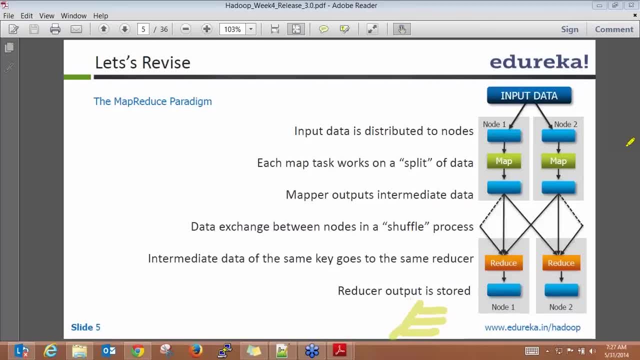 Not each of the node. each of the reducer will write on the separate output file And once we'll see the example of the partitioner, these things will be clear to you, where you will be able to see that: Okay, This data get distributed based on the which reducer it is processing. 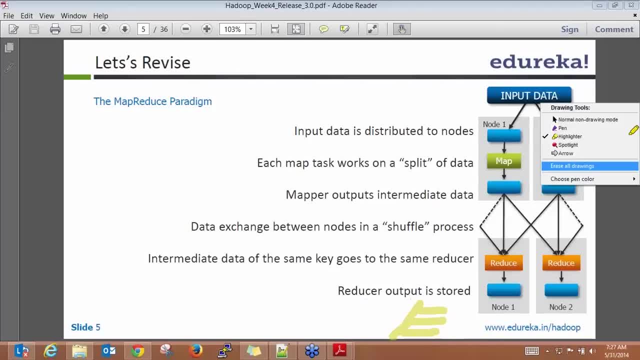 Okay, So we'll see about that. Okay, So is that answer your question? Meenu, Okay, And I see So. can I see that partitioner is responsible for directing the intermediate data of the same key to the same reducer Exactly? 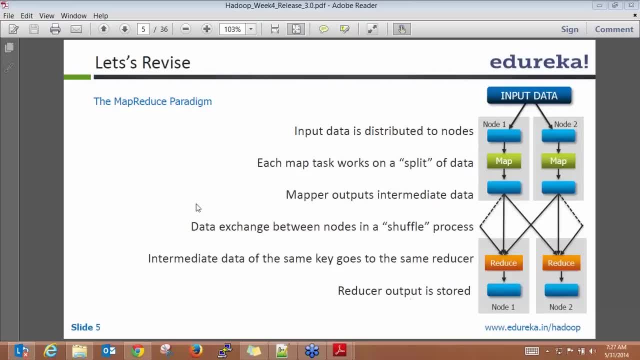 That's the role of the partitioner. Okay, So each key it will determine how to move the data from that per output to which reducer. So that will be determined by the partitioner. And if you are using, you know the one partitioner. so in that case, what will happen? all of those? 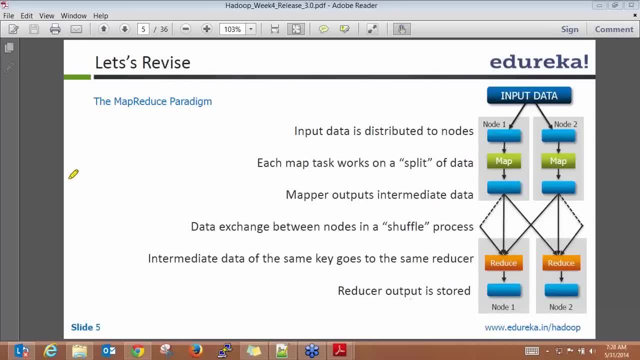 keys will go to one particular partitioner. Yeah, So this only one copy of the output will be saved after the reducer right, Not the three by default. No, it will be three because whenever you write anything inside the Hadoop. so all these reducer 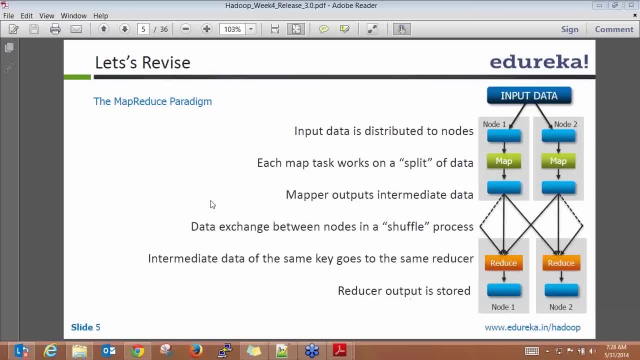 output will be also stored. So whenever you will store anything inside the Hadoop it will go basically the same writing process where it will involve the name node: get the block location and then it will write that. So it will go through like three copies. 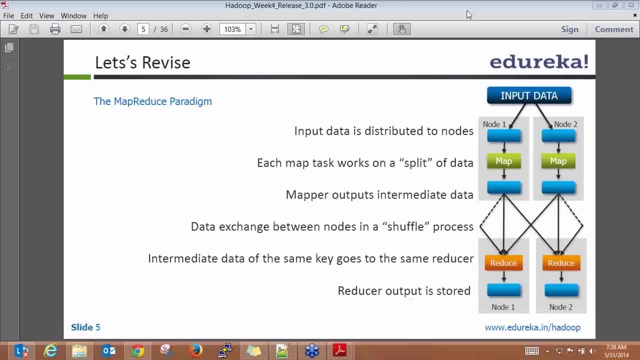 Okay, Meenu, We'll go through the examples and things will be clear. Okay, And if you want to reduce this traffic, right? We saw another concept While moving the data from the mapper to the reducer, so instead of transferring each key. 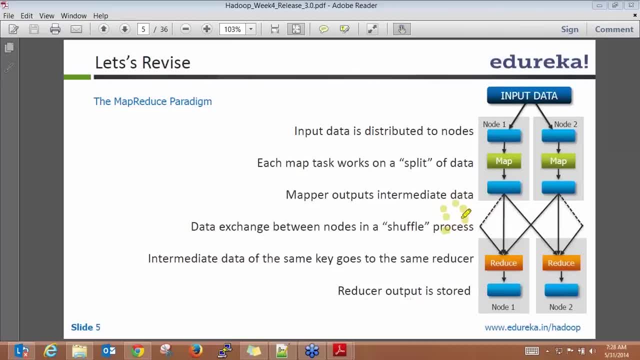 value pair. as it is what you can do. you can basically consolidate all those things at the mapper output level so you can have one key and the associated value and that particular value. you can transfer that So that you can do by using the concept called combiner. 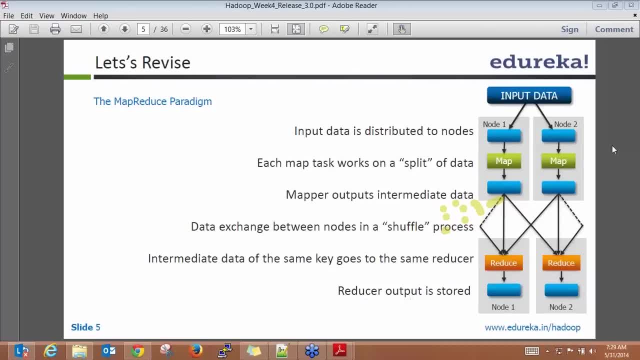 Okay, So I hope this gives you a quick overview, like what all We discussed in the previous class, about how the MapReduce flow works. right, Any question you have before I proceed with the like showing you like how to use the partitioner and combiner. 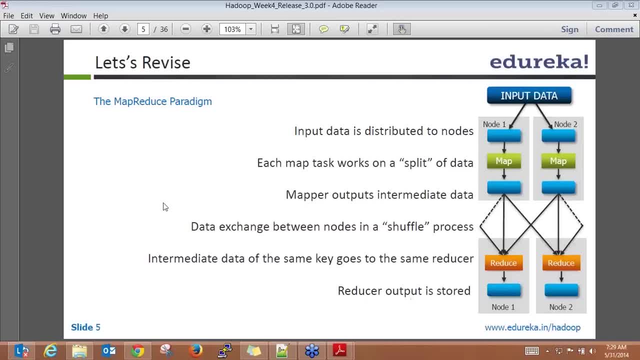 Okay, I do see a couple of questions coming here. Okay, Meenu. Okay, Just a follow-up question. So from distributing the base data, how many nodes we have- we will have that much reducer. Now I'm just trying to read it. 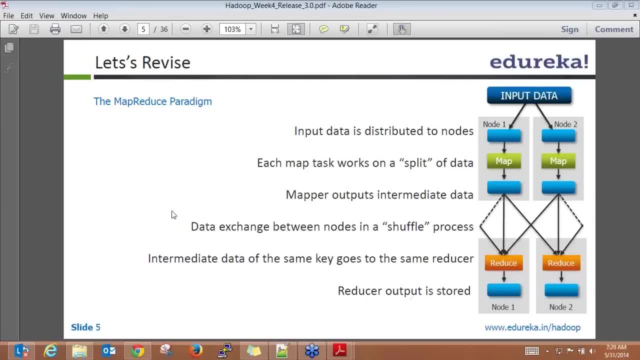 Okay, Please read your question, Meenu again. Okay, Based on the data, how many ever nodes we have, we will have that much reducer. Okay, So your question is: is it like, suppose, if you have 15 nodes inside the cluster, the 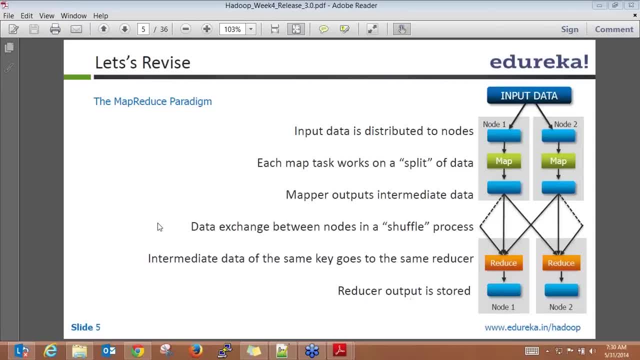 output node, the processing node. so you mean the 15 reducer is going to run. Is that your question, Meenu? Okay, No, So it's not determined like that way. So if you have the 15 nodes, it may happen that you know all of your data will get. 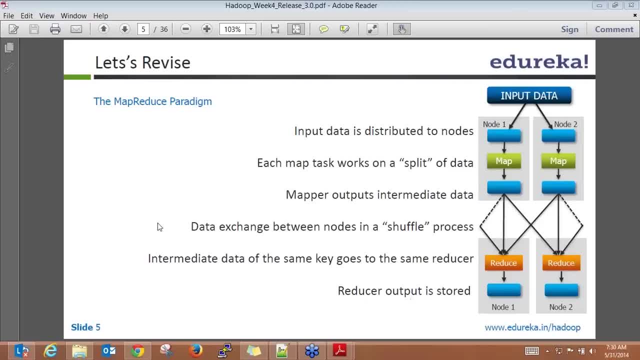 stored on all those 15 nodes. but the number of the reducer which you want to determine, that will be something you can control from the program. so you can determine how many number of the reducer you want to run. So you may run 15 reducer, you may run 5 reducer or the 10 reducer. 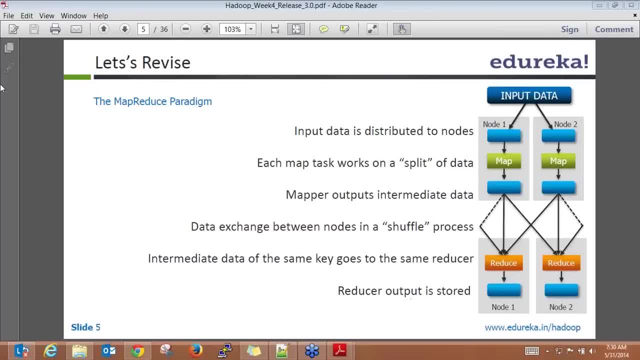 So how it will be determined is generally in a Hadoop kind of the cluster where you will have multiple, you know the projects or the programs that will be running inside the cluster. so each of the program will get something called the queue, so the number. 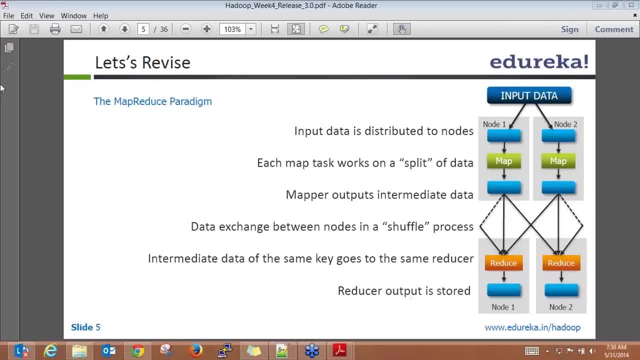 of the reducer and number of the maps. The number of the map slots which we have in the cluster, that will be determined based on how many cores you have inside the cluster. so based on that you will determine how many number of the slots you will reserve for the mapper and how many slots you will have for 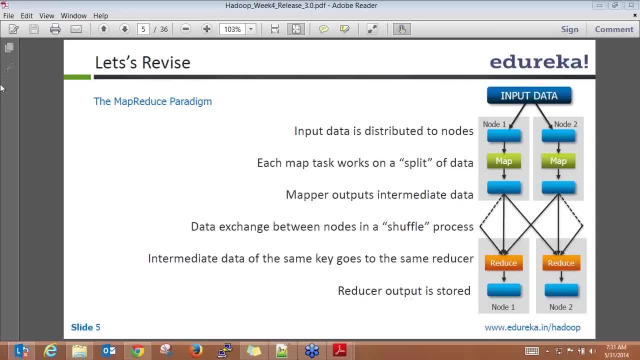 the reducer. So suppose if you have 40 reducer slots available in the cluster, if it's a small cluster. so out of that, suppose for your particular queue you have 15 reducer assigned. out of that, suppose 3 jobs are running so each of them can run maximum like 5 reducer or something. 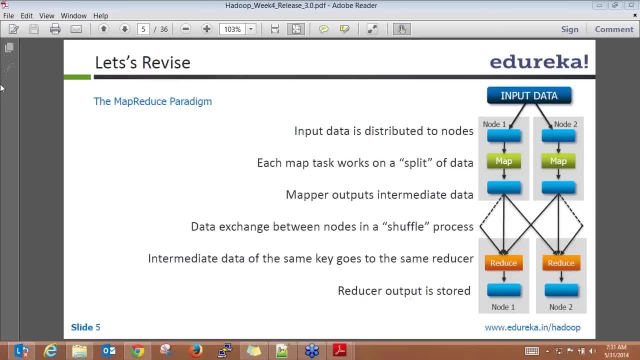 So that particular setting you will do as part of the program. whenever you are running the program you can specify how many reducer you want to run, So you can run one reducer. if you don't specify anything, by default everything will go to. 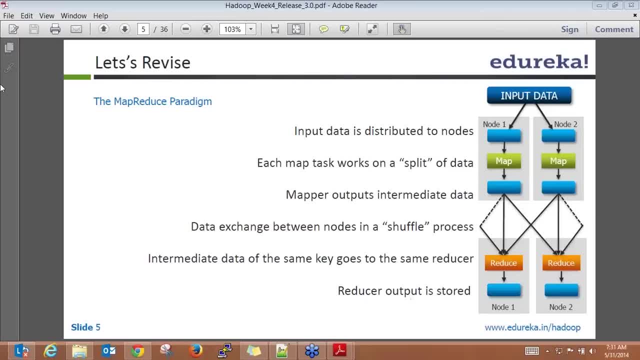 one particular reducer. so you will run one single instance of the reducer, or what you can do. you can specify like 4 or 5 reducer and based on that your data will get divided into those 4 and 5 reducer and then you will get the final output. 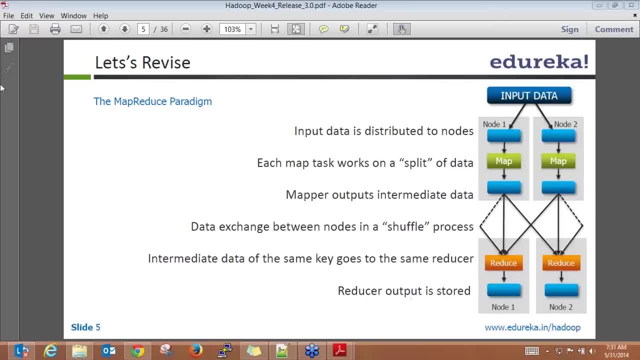 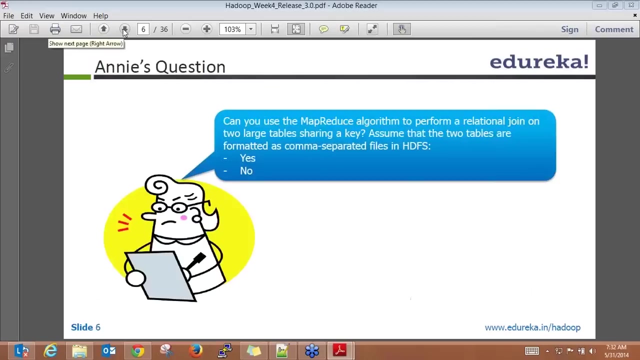 So that's the way the number of the reducer is going to be determined. So you can specify that You are submitting the command and the command line as well as inside the Hadoop code. you can, You got it. Okay. I think we have not seen the join, but any other question here, guys? 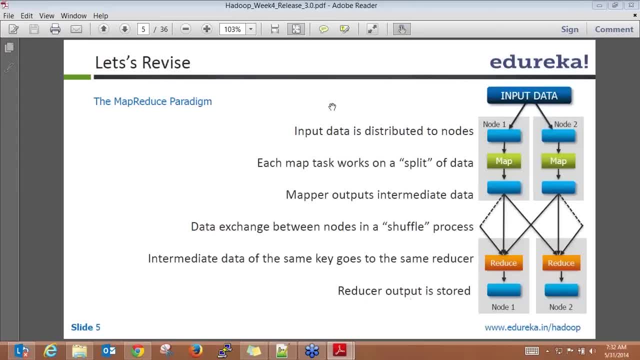 So before I take any question, I would like to take any other question. guys, in terms of this whole framework, Are you guys clear How the map reduce partitioner combiner Any other questions? So the map reduce partitioner combiner- it works. 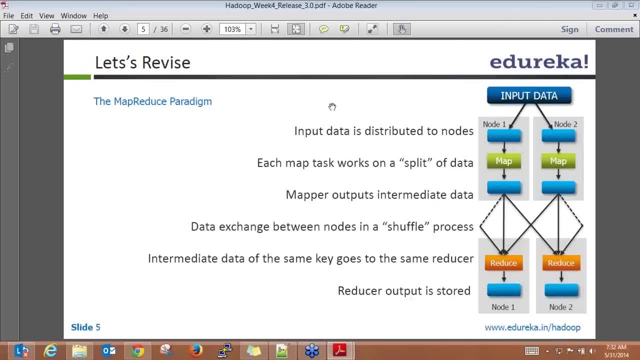 Although we are going to see again how to create the jar file and all those things we are going to see. but the concept is this whole diagram is clear. It should be clear in your mind how the input will go to the mapper. mapper will process. 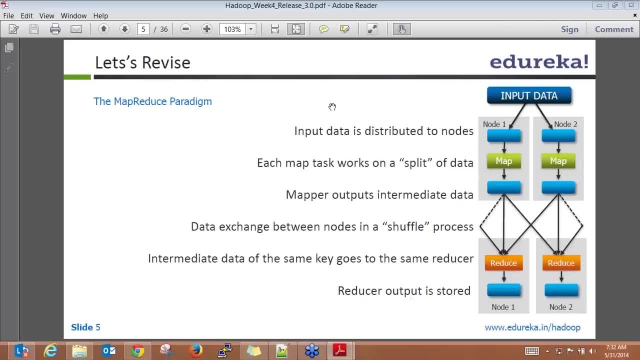 that then you will have the key value pair. If you use the combiner, it will consolidate all those output from the mapper and then you will move that to the reducer And once it goes to the reducer it will do the processing and then you will get the final. 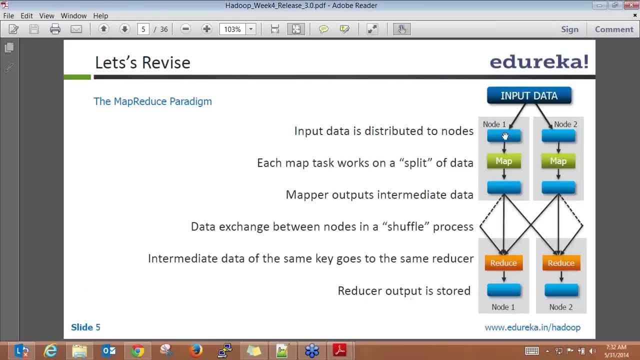 output set by using the partition logic. Is this clear? Okay, so I get minute clear: Devinder Hitesh. okay, And how about other people? Just three people let's let me assign. I need this thing. 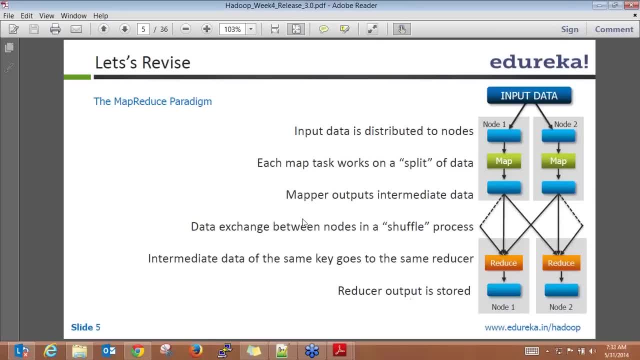 If you have any confusion or doubt, just let me know. I would like to take that one. And Subhajit says: can you please explain the modular calculation? Okay, sure, Subhajit. Okay, Okay, let me just show you. 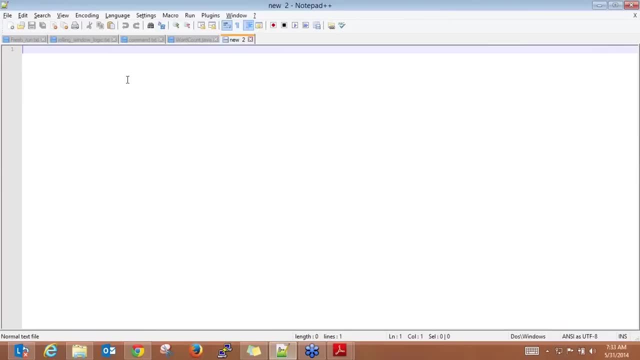 So suppose modular calculation, it works simple. Subhajit says, can you please explain the modular calculation? Okay, sure, Subhajit. Okay, So, Subhajit, if you have four reducer. so now you think of like each of the key right. 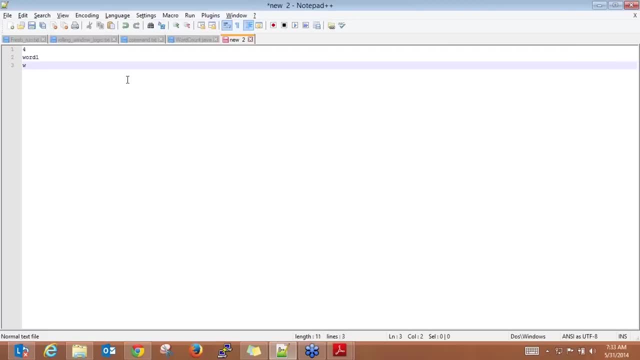 So you have maybe in the one word, one, two, okay, three. So now what will happen for each of the key? what you will calculate is the modular function. So, since the number of the reducer is four, so you will calculate modular by four. 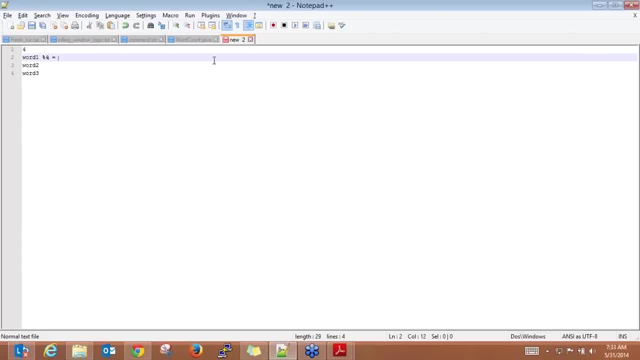 And what it will output. you right any number. if you can calculate the modular, it will get. you will get any number between zero to three. some number, it will come right. So you will get, maybe suppose two here, right. 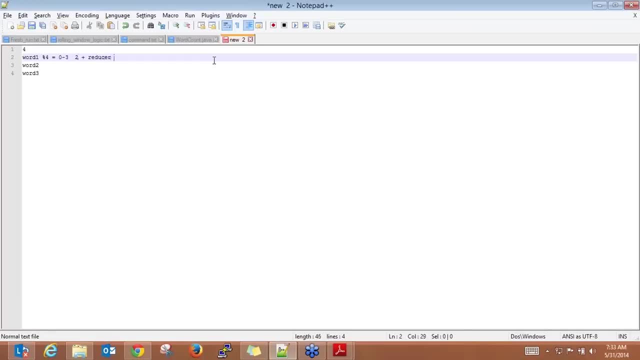 So it means the reducer- reducer will be generally between zero to three, that it will be numbered by zero to three. So when you specify this you know you get a number two. it means it will go to the zero one, two and three. 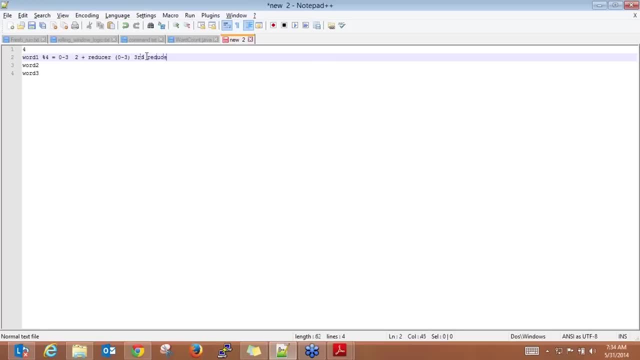 So it will go to the third reducer and it will process that okay. Similarly, for this particular key, you may get a value, something like you know the one or you know two But one. if in that case it will go to the second reducer, okay. 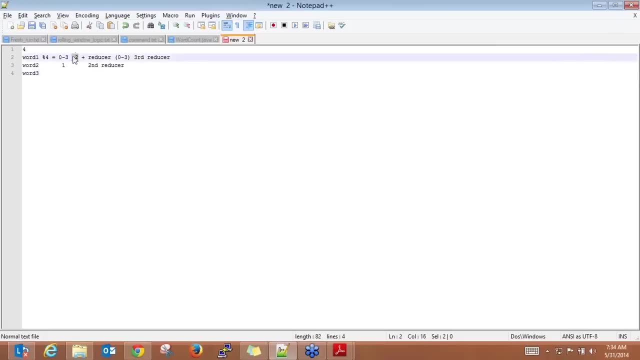 In the word three, it can happen that it can again have the output as two right, Because two of the key may have same output, like if you go 14 divided by modular, it will you know, or you know, take the example- like two right. 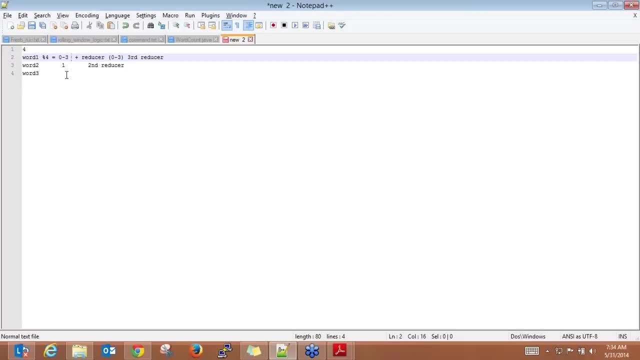 So if you're dividing any particular word, it may have a modular two. another word can also result in the modular two, right? So what the reducer say? is that all that reducer want? Okay? So the reducer says: for that particular key, give me all the input data set. 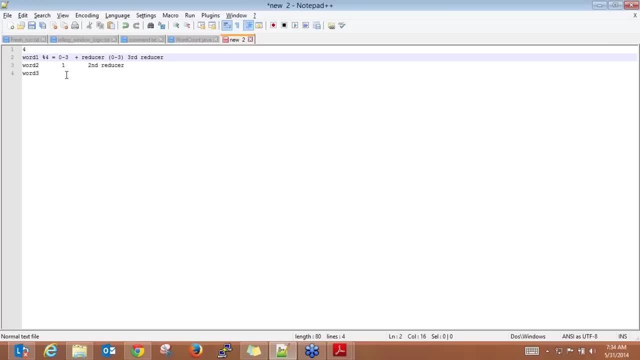 That's the reducer. It doesn't restrict that. okay, I will only process one particular key, because it's not possible, because you will have multiple keys which the modular function will result in the same value. So that's what you will have like number of mappers: put 5,000, you have then the number. 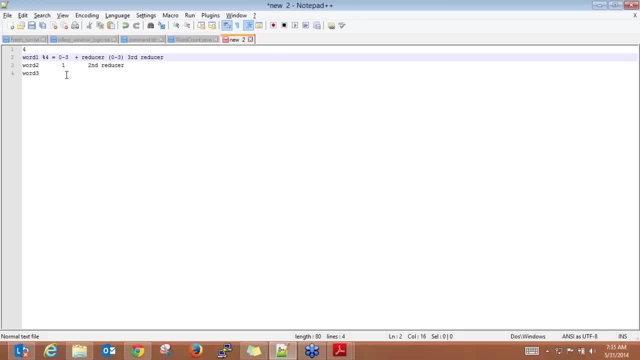 of the reducer, you will have only 30 and the 40. And all these different keys will get divided into these 30 and the 40 reducer, which you will run inside the cluster, So each of the reducer may get multiple. Okay. 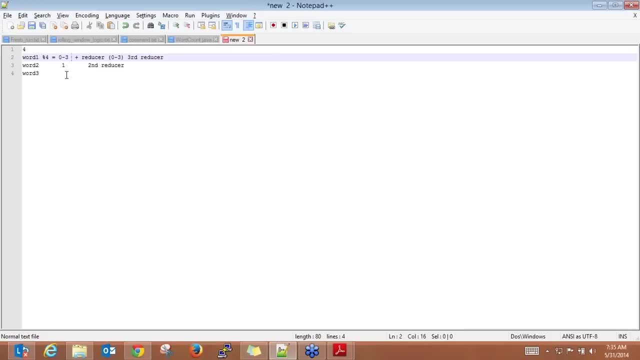 You may get multiple keys to process, but whenever they get any particular key to process, they will get the all the input data set for that particular key to process that right. So that's the overall concept we have, like how the partitioner will make sure that all 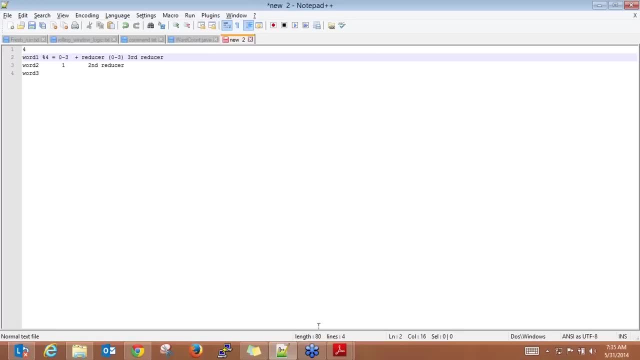 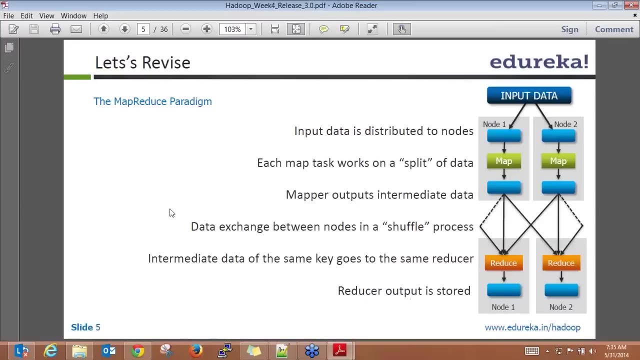 of the key value pair goes to a particular reducer. Okay, Is this clear, Subhasit? Yeah, you got it Okay. You got it Okay. Okay, Anybody has any other question? Hey, no problems, Subhasit. 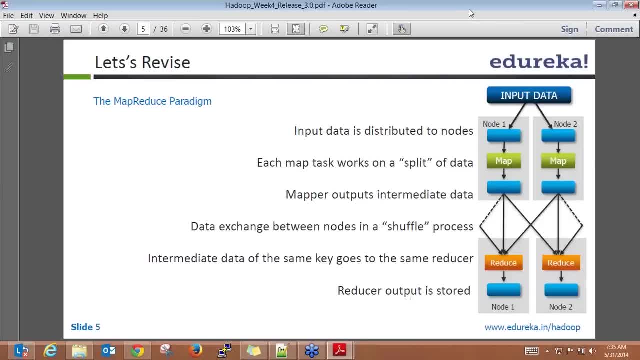 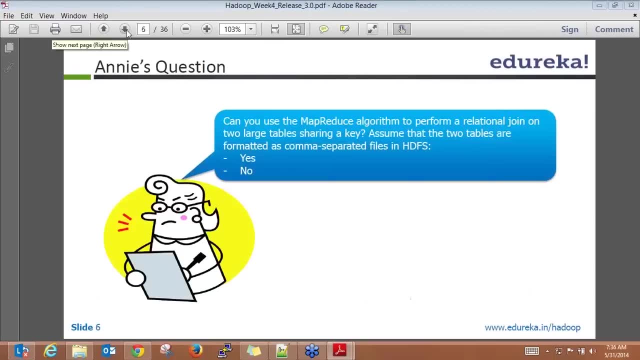 Okay, Okay, Cool, Okay. So now, since you guys have no question, right, so here Amy has some questions, so let's take some questions from Amy. So can you use the MapReducer algorithm to perform a relational join on two large data? 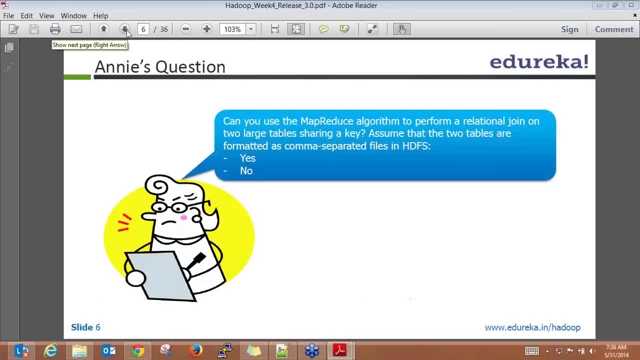 two large data clusters? Yes, Okay. So let's assume that the two tables sharing a key assume that the two tables are formatted in common separated files in HDFS. So this question is just a guess, guys, because till now I have not told you about the join. 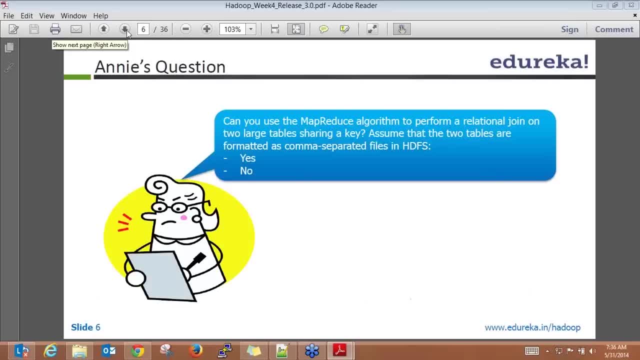 I think any question came a bit early. So yeah, just a guess: do you guys think a join can happen in using the MapReducer? We'll learn about that right how it happens. So maybe it's just a kind of a guess for you. 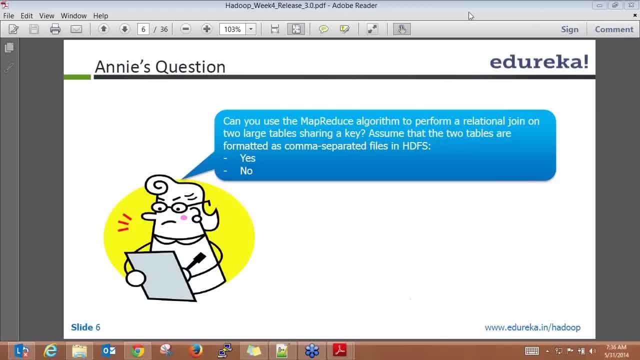 Okay. So all of you think that, yes, a join kind of operation can be performed by using this. Yeah, Yeah, Yeah. So there are a couple of ways how to do the join. So there is a map-side join, radio-side join, in-memory join. 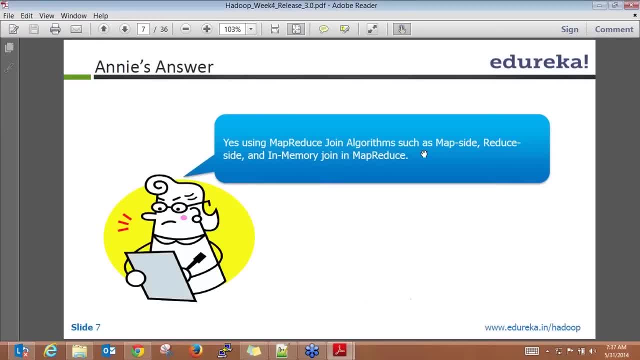 So we are going to talk about that, like how to do these different kind of the join inside the cluster inside the Hadoop framework. Okay, So here is another question from Amy. okay, So what type of algorithms are difficult to express in the MapReduce? 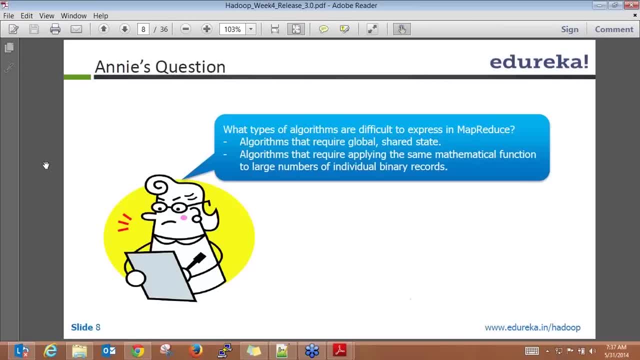 Okay, So this you should be able to understand about the whole flow, right? So just we discussed, right So, algorithm that require global or shared state, or algorithm that require applying the same mathematical function on the large number of individual binary cards. okay, 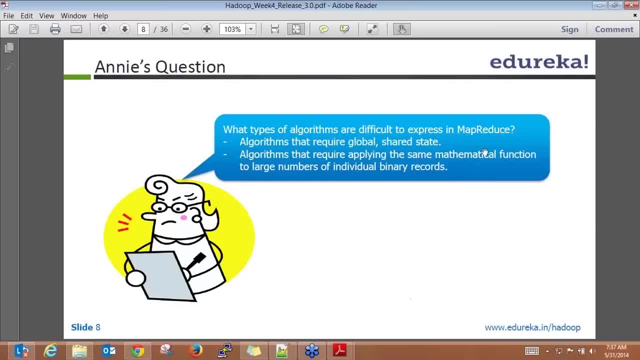 So only two options, so just pick it up whichever. Okay. So which kind of the algorithms will be difficult to implement? based on the how you see that, how the MapReduce works right, based on that particular flow, how you think that which? 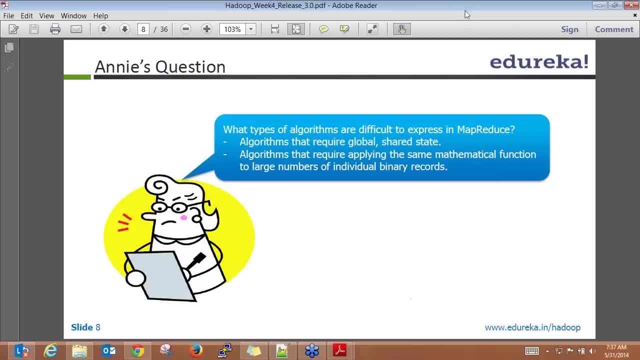 is a difficult generally to implement that. Yeah, So I get couple of answer here and people like: wherever that requires global and the shared state, right, Okay, Yeah, So those kind of algorithms are really going to be difficult to express that in the yeah. 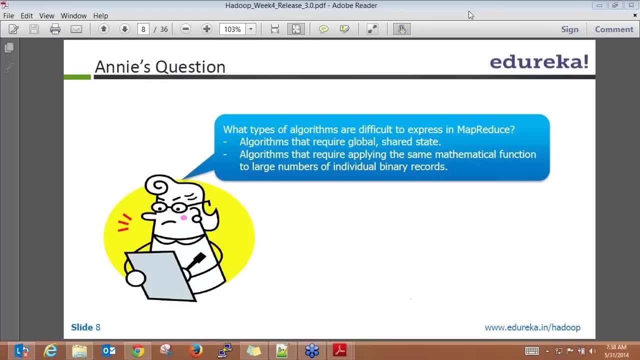 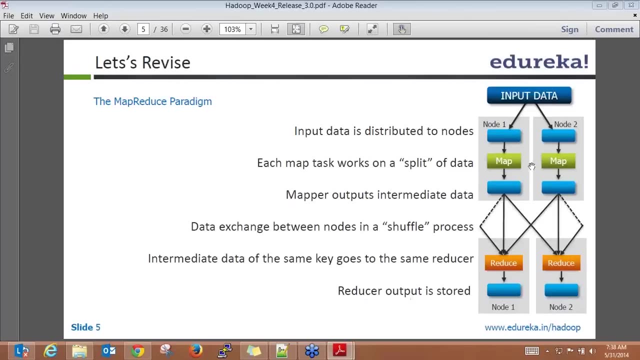 thanks, Patrick. man, Yeah, Sachin said second one. No, Sachin, it's the first one. So all the you know the program or the algorithm where if you have to share the state, it's going to become difficult for the MapReduce to implement that, because if you see the 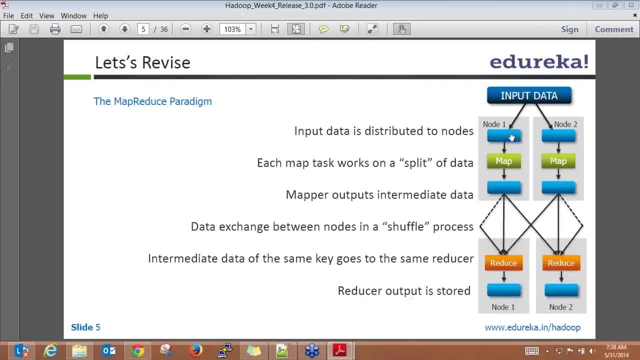 mapper and the reducer, where the actual the code processing happens. those particular functions works independently, So they don't share any kind of the state that. okay, currently my status is like this: I have the count values four and then your count value is two, so add it and then do some. 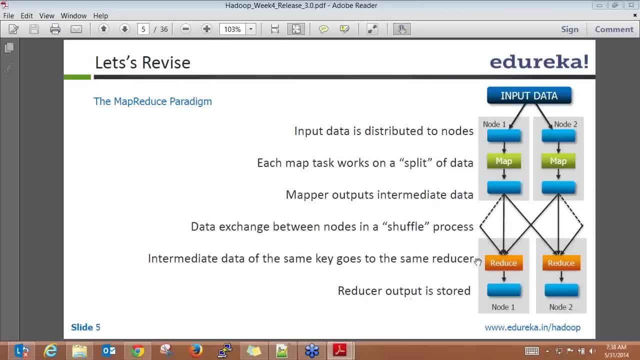 kind of processing. So there is no communication happens between all these processing part, the mapper and the reducer part. So all of them run independently And due to that, if any, that kind of the sharing is needed. So those kind of things it will not be possible to implement using this. you know particular 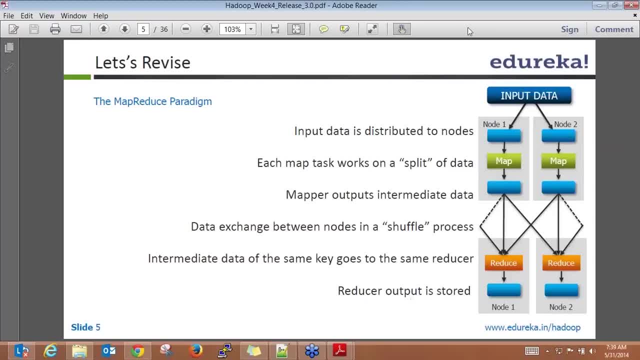 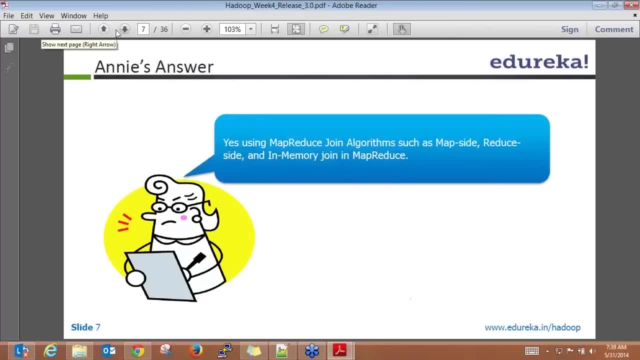 flow, the MapReduce flow. Okay, So if you guys remember the example which we saw where we had the counting problem in our hand right, So when we wanted to do the count, there was one way where you can share the state between: 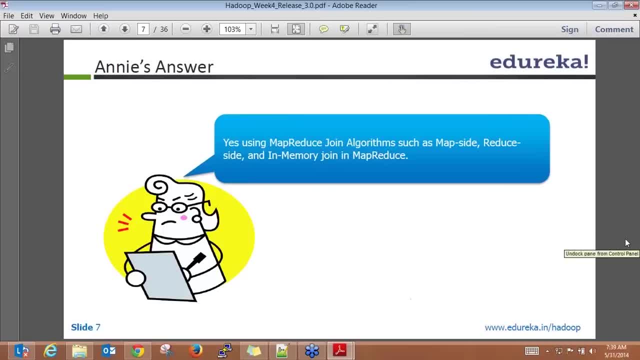 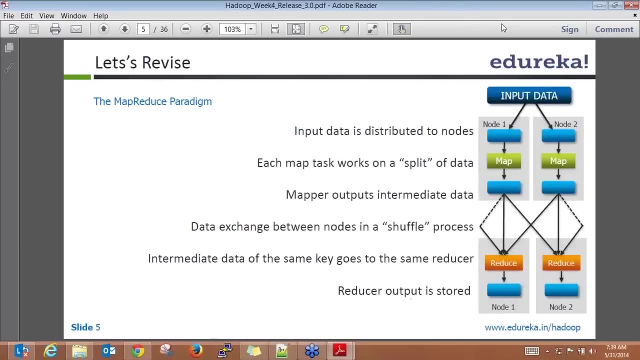 each process, So that you know like you can you can, you know, count it right. whenever one process finished, it passed the value to the next process And then you know it continued with the processing. Okay, To give the example, you know, like in the last class, what we discussed is, if you have, 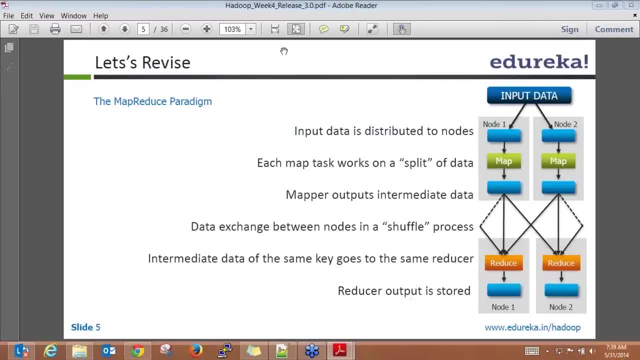 the word count example if you want to do that. one is like one mapper completes the reading of one particular input line And once it finds that, okay, each word has like four times or five times, then it passed that particular thing to the next mapper. 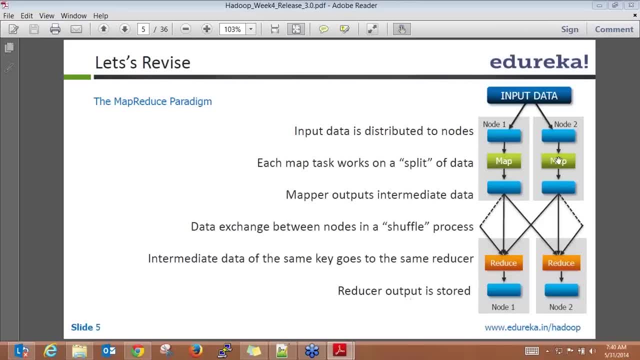 And when the next mapper runs it processed that right. So that could have been like one kind of the implementation. But in that case you share the state And suppose if this map goes down, then again you have to depend on this to come up and 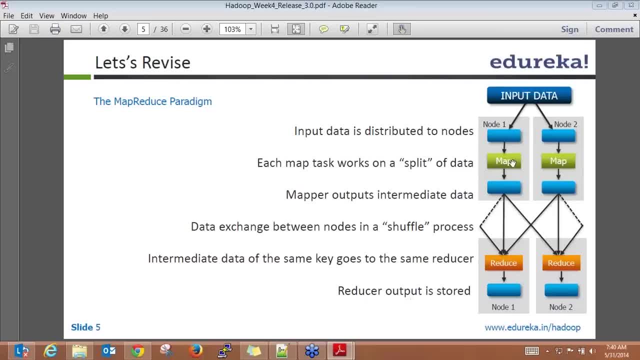 then reprocess and all those things. So in our case that's not the case here in the MapReduce framework, everything runs independently and you don't share any state between each other. Yeah, it's like a kind of you know, like one process output, go to another process. 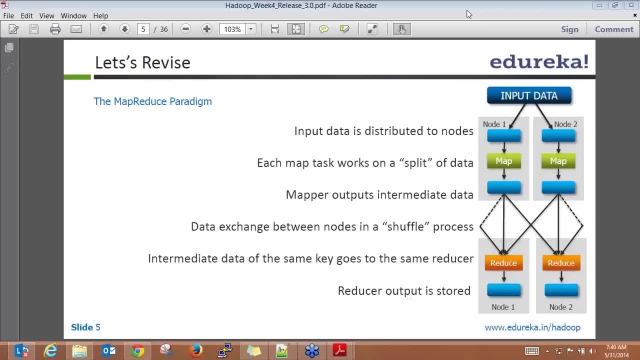 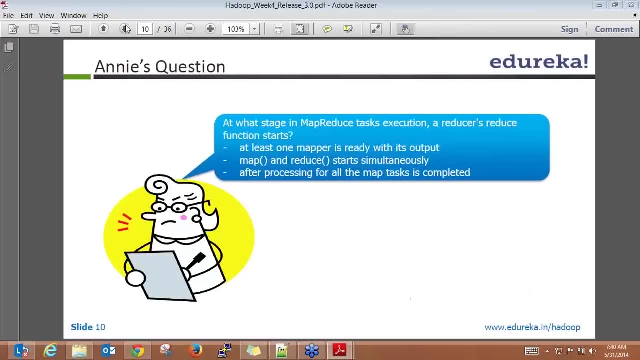 that kind of the sequence, So those kinds of things we don't have here in the MapReduce framework. Yeah, Okay, At what stage in the MapReduce task execution a reducer or reduced function starts, In general, right, This is something you can configure it. but in general, like when the reducer will start, 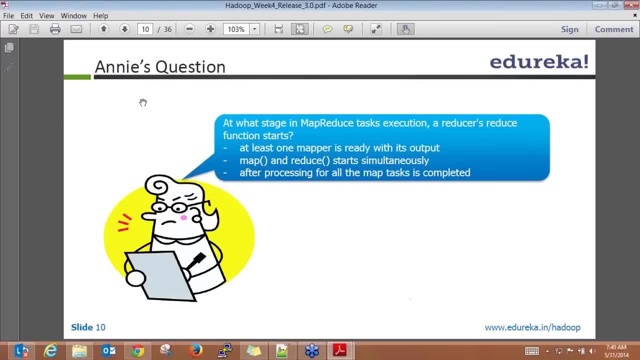 working on a given data set which is coming from the mapper. Okay, I see a couple of answers here, So all of you guys can be interactive guys here on the question window, because this is the only way I can interact with you. 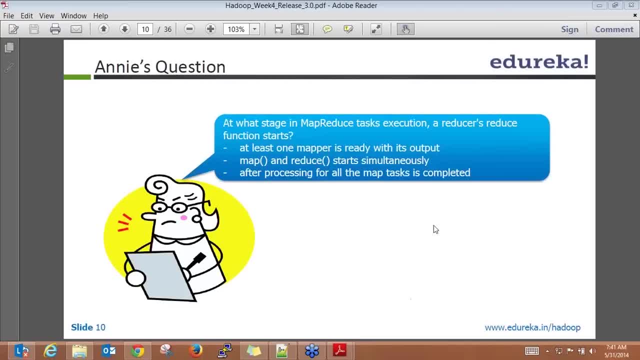 I can see your answers and I can provide the clarification. So just be interactive. All of you try to attend the question. Don't worry about right and wrong answer. right, If it is not correct, it will help me to explain it right now. if any other concept which is 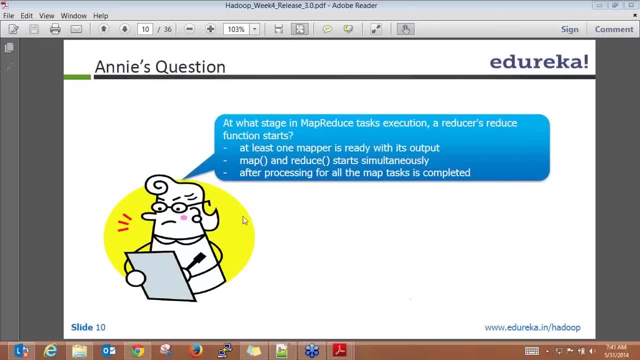 not clear. So please, all of you try to answer that. Okay, Bhaskar says Bhaskar, I see your option: three years. answer anything any other question you have? Okay, Yeah, So it basically starts after the map task has completed, and the reason is because, if 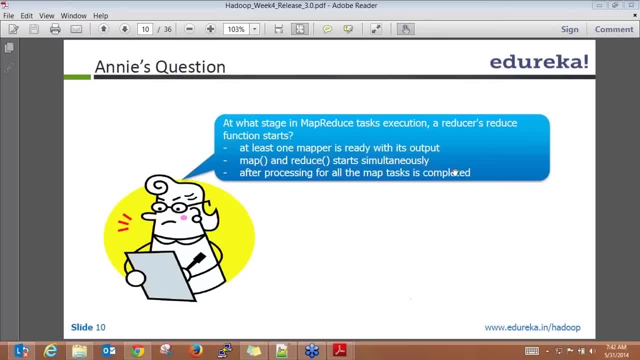 you want to do any kind of aggregation or the summarization of the data reducer has to basically get all the information, All the input data set and process that. So this is something. if you will go to the actual implementation of this one, this is 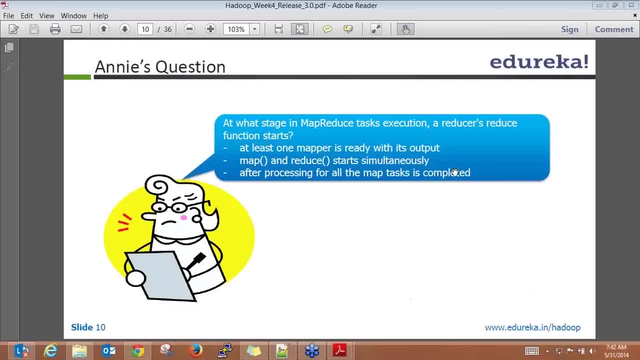 like the theoretical stuff right. When the reducer has to start, it has to start only after all the output from the mapper is available, But before that there is a process where the mapper moves the data, where the reducer needs to move the data from mapper so that it can start processing. 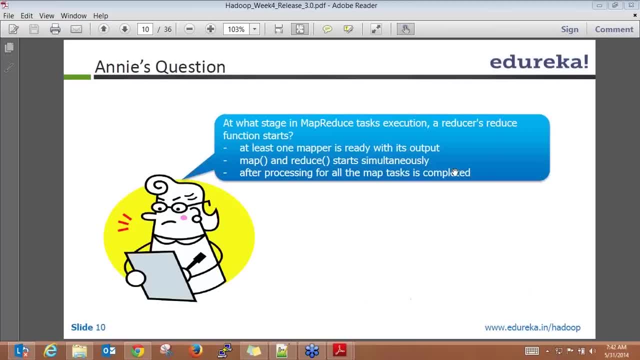 So that's shuffling process. sometimes it starts. that's configurable. you can start it as soon as the mapper output is coming, You can start the shuffling process. So that happens sometimes right where you will see that it starts, but actually not. 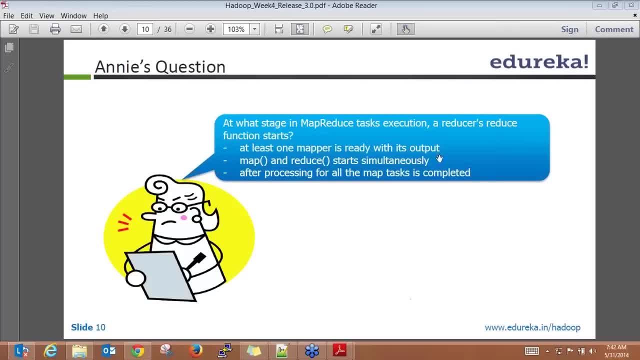 the reducer is working with that particular time. the shuffling process is what is happening inside the cluster. But generally, yes, the reducer will work only when the mapper output is coming. Yeah, Okay, Okay. So this one is an interesting one, if you guys remember the concept. 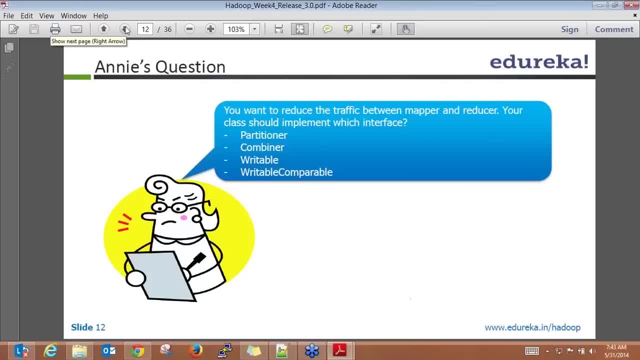 So if you want to reduce the traffic between mapper and the reducer, your class should implement which interface, Partitioner, combiner, writable, writable, comparable Which particular thing basically reduce the traffic between the mapper and the reducer, Where we have the bottleneck in terms of the disk as well as the network, kind of things. 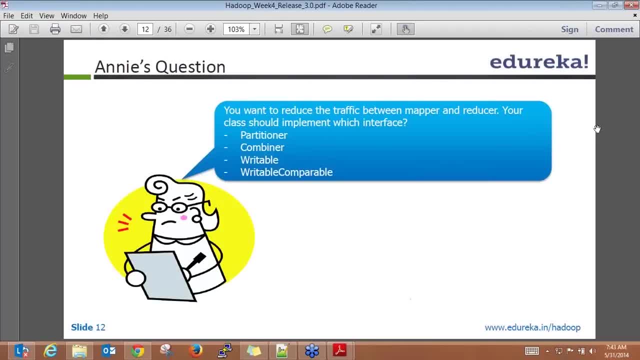 Okay, You know what? Yeah, Answer from all of you, because this will help me to understand that you are clear with all these concepts, these terms, guys. So please can all of you try to answer this one. Right wrong, don't worry about that. 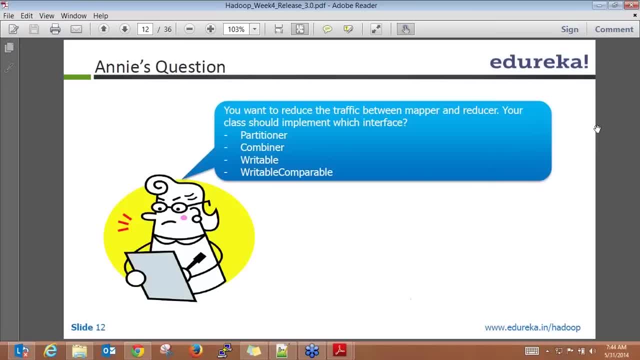 Vasquez is confused now. Okay, Okay, So the right answer is the combiner. So if you want to basically move the data from mapper to the reducer, the logic, how to move the data, how to you know? Yeah, thanks, Vasquez. 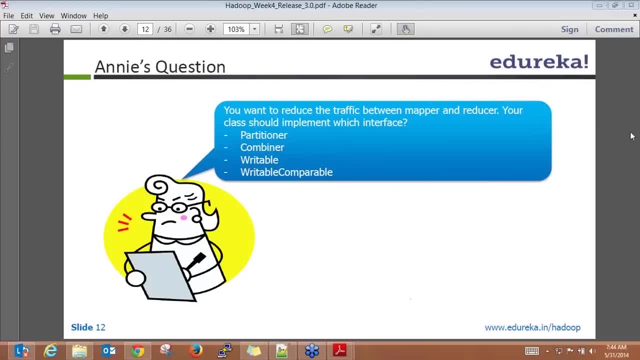 You got it right? Yeah, So if you want to move the data from mapper to the reducer, you have to put a logic, and that particular logic how the data transfer will happen. that will be done by using the concept, what we have called the partitioner. 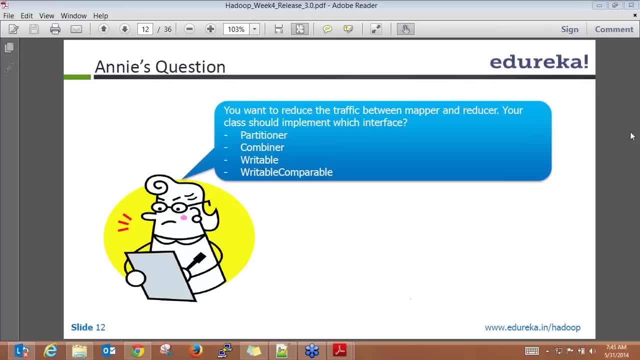 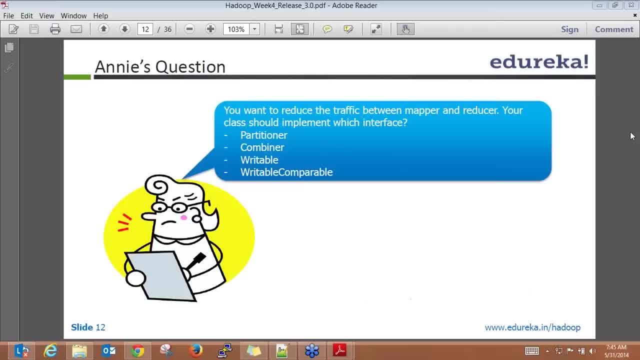 the you know each that granular level. if you transfer the data, it will be too much data to be transferred across the network. So what you can do is you can implement a combiner logic and that logic what it will? 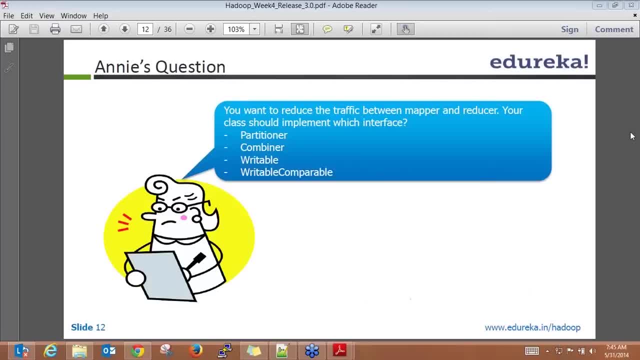 do is, instead of moving the whole data set across the network, it will just combine all the mapper output and then it will move that particular data set to the reducer. So that way you will have the less traffic going to the reducer, Yeah. 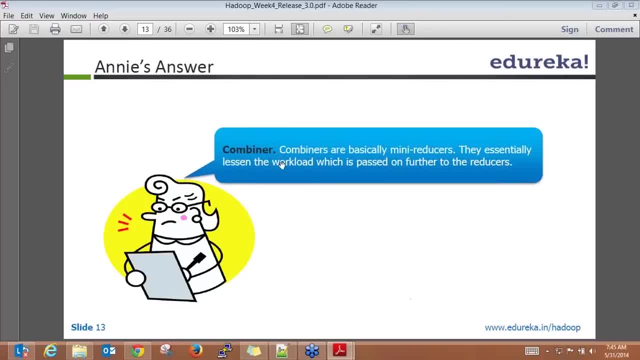 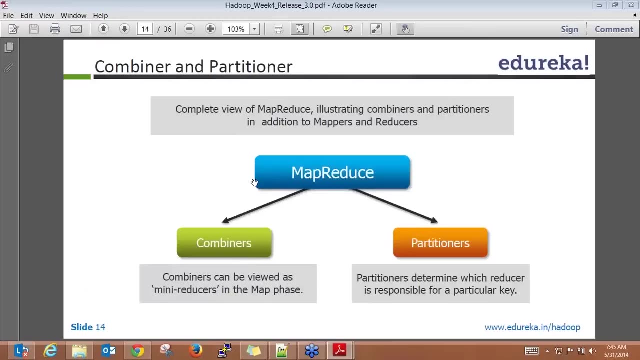 So it basically acts as a mini reducer And you know, it can basically take some of the work away from the reducer, do it locally on the mapper output and then pass that output to the reducer, which will get processed. So this is the concept combiner and the partitioner. 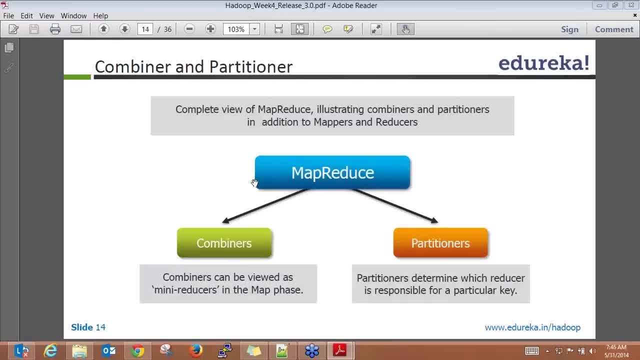 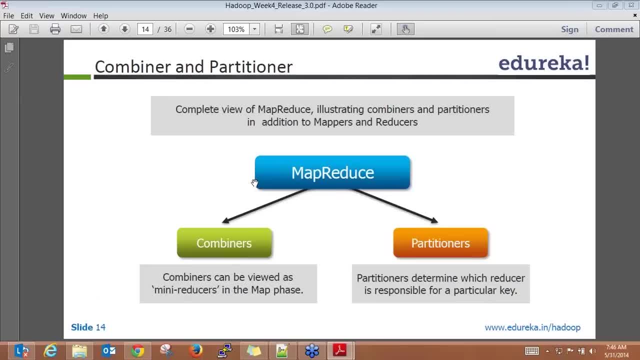 the sum value for that mapper output and then the partitioner. it basically determines which reducer is responsible for a particular key. So that will say that okay, this key has to go to reducer number 3.. So that thing will be determined by the partitioner, while the combiner what it does is whatever. 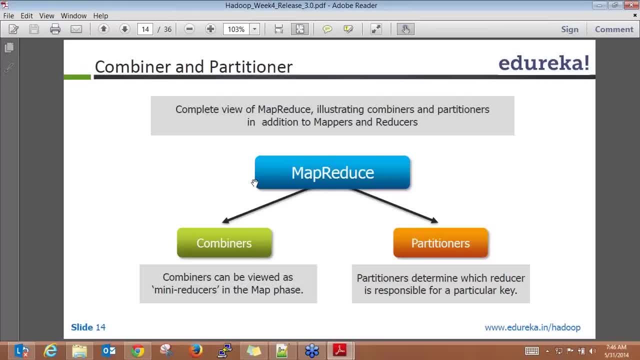 the reducer is going to do, to do the aggregation of the data. same thing: reducer will work on the whole data set, combiner only on the mapper output. it will do the same, similar kind of function and then you will be able to get the consolidated output of the mapper. 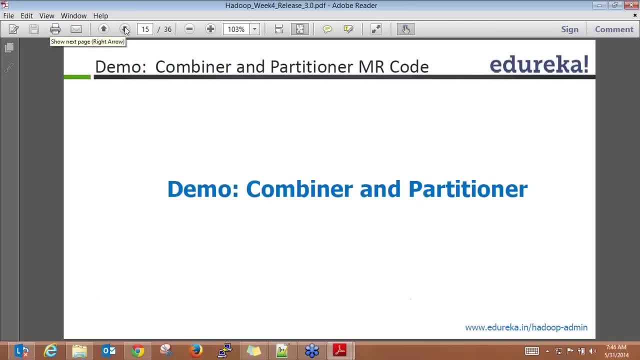 So next, what we are going to see is we are going to see an example of the combiner and the partitioner, where we will see that if you have to write your own partitioner, so till now we have been learning about the default partitioner and I'm telling you that you 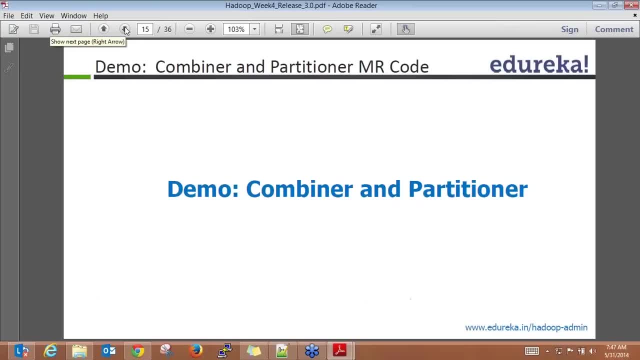 have the multiple files where the data will get stored. So now what we will see is that we will see that, how this partitioner works and how you can implement your own partitioner, and by using that you will be able to basically 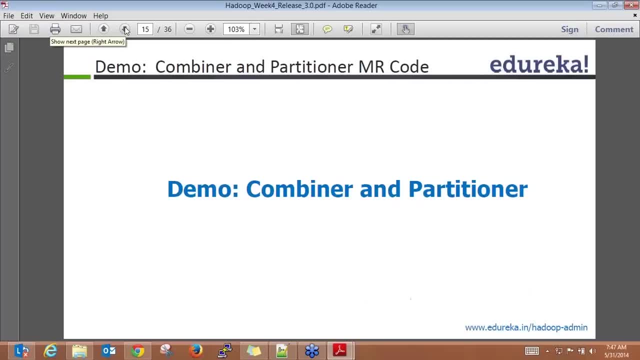 control How the data distribution we are going to happen inside the cluster right. So whenever you have the multiple reducer and you need some kind of the way to determine which is the appropriate reducer where you want to send a particular key value pair, 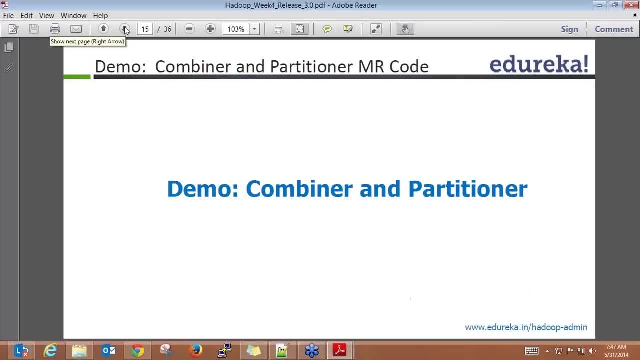 and that's where you write your own partitioner to determine that And the default. if you don't write it. it's a kind of the hash value for the key and that will determine which reducer you have and if you want to, you know, implement. 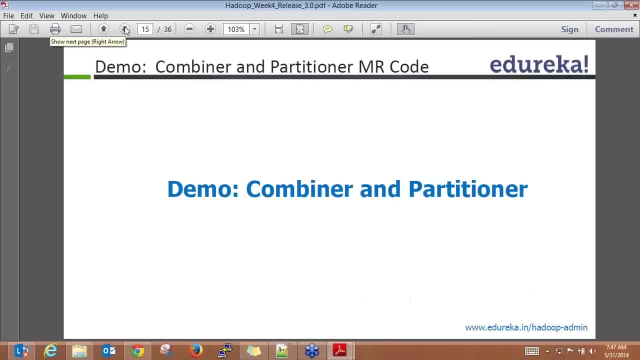 your own partitioner. what you have to do is you have to basically implement two functions called configure and the get partitioner. So by using these two functions you will be able to implement your own partitioner. So what the you know get partitioner will do is it will get kind of the integer number. 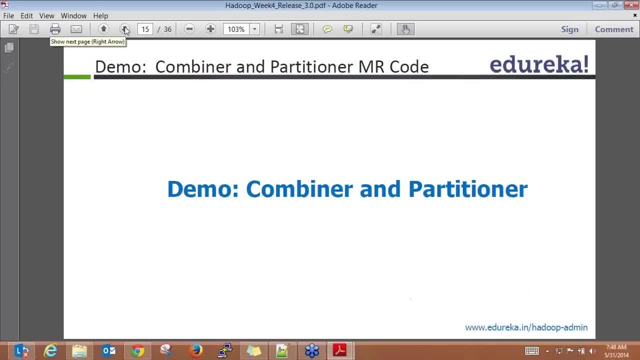 between the. you know, whatever the number of the reducer you have. So suppose the number of the reducer is four, so it will get a number between zero to three and that will determine like which partitioner it has to send particular value. 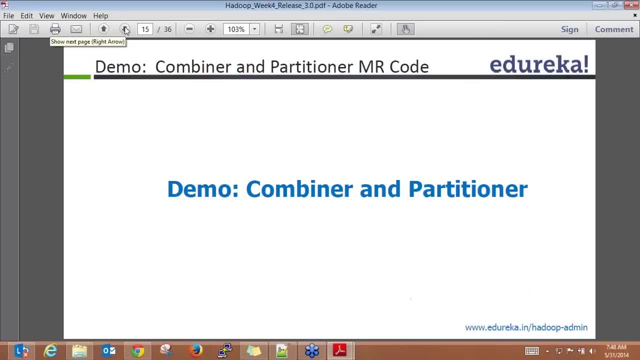 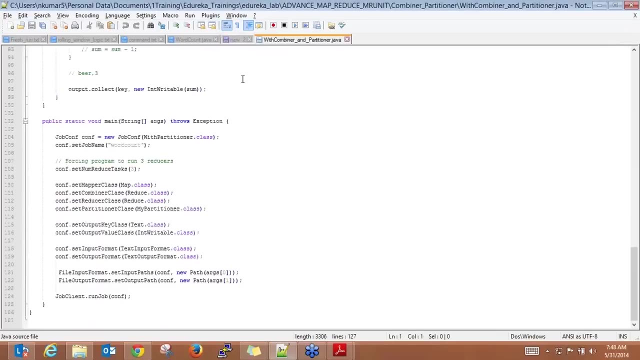 And the configure is basically to configure the partitioner to run on a given key value pair. So let me show you So in this example. what we are going to see is we are going to see an example like how you can write your own partitioner and based on that, your data will get distributed. 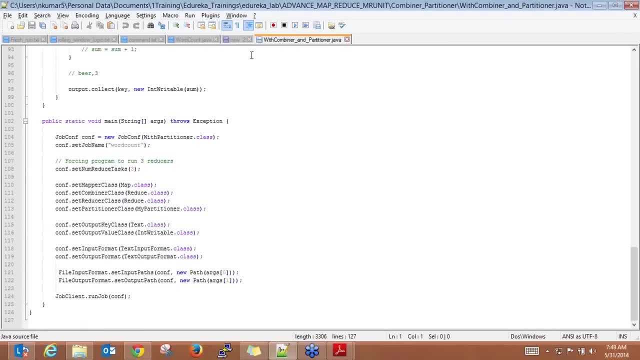 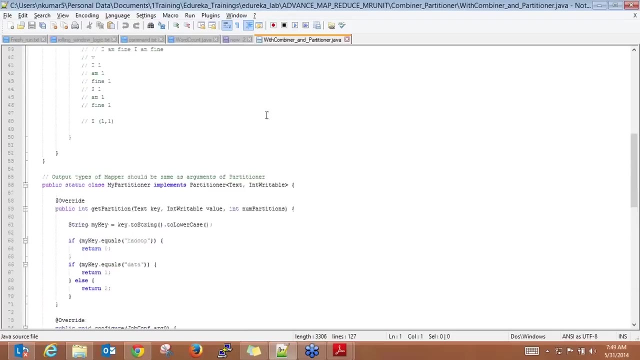 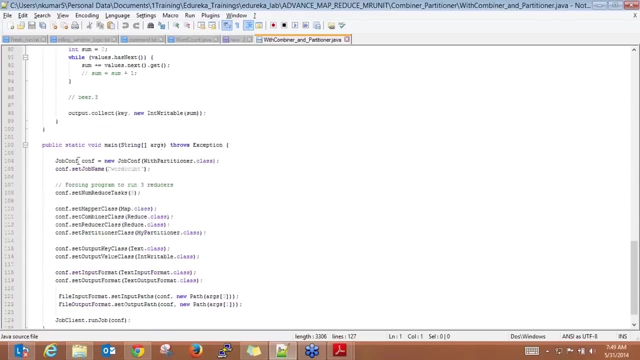 based on the logic. whatever you are going to write for the partitioner, based on that particular logic, your data will get divided to the different reducers. Okay, Yeah, Okay. So here what we are going to do, apart from the flow, what we have, where we specify what. 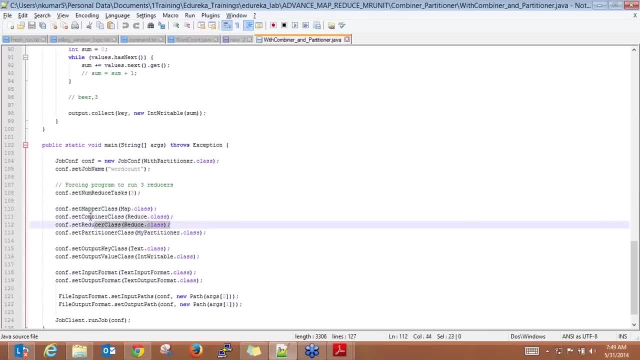 is the mapper class? what is the, you know, the reducer class we have? okay, And one more thing, guys. I'm not sure if we discussed about the combiner in the last class, the example- but if you want to specify for a combiner, all you have to do is like: 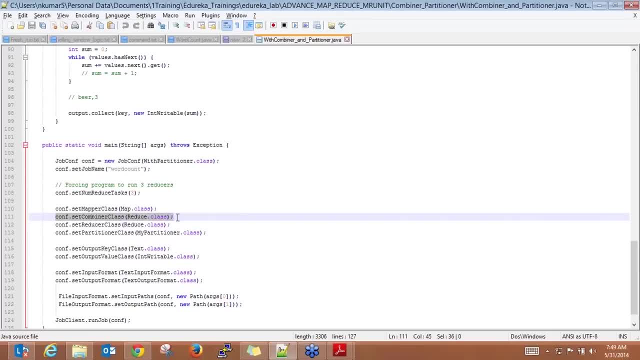 In case, if you are using the same logic, what you are using for the reducer- to use in the combiner, what you can do is you can use this confsetcombiner class and whatever the logic you have written for reduceclass, same, you can pass it to the combiner because 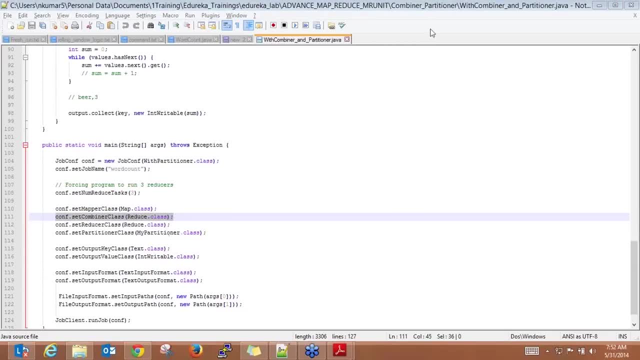 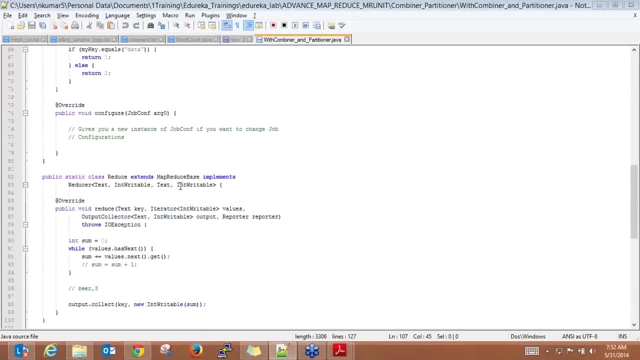 if you see, like in this case, like Yeah, So what we are doing here is we are writing our own combiner in the partitioner class and I'm going to explain to you, like, what we are going to do here and how we do that. 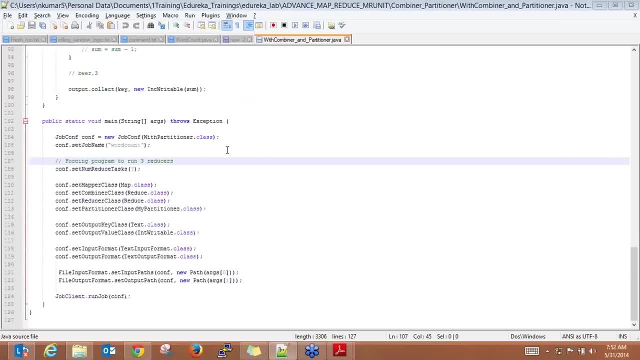 Okay. So this is like whenever you write a MapReduce code. what you have to do is basically, you have to write the mapper class, you have to write the reducer class and you have to write the driver class. This is the three things which, in the MapReduce framework, is there. 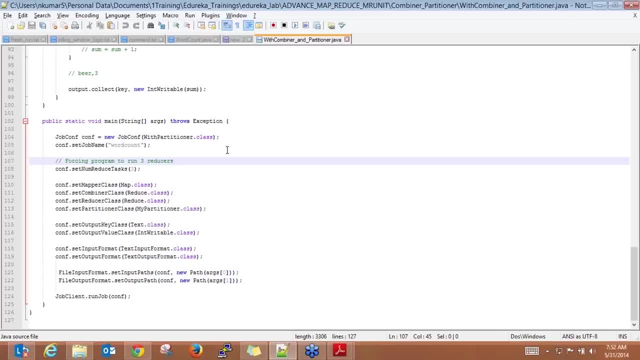 So: mapper, you write the mapper logic, reducer, you write the reducer logic. and driver, basically you control, hold the execution like which mapper it has to run. what is the input format? what is the output format? right? 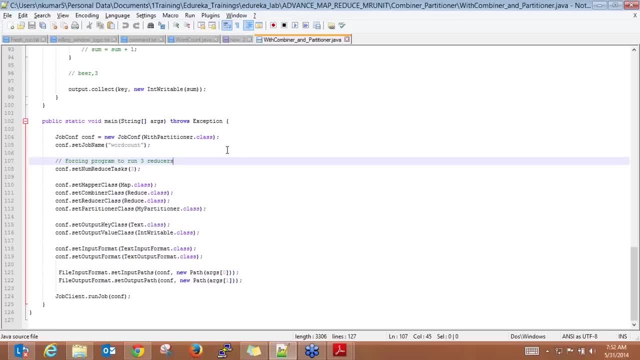 What is the input data file part? what is the output data file part? So all those kind of things you control inside the driver class. So driver class is basically Basically nothing like you can relate it with your main class which you have in the 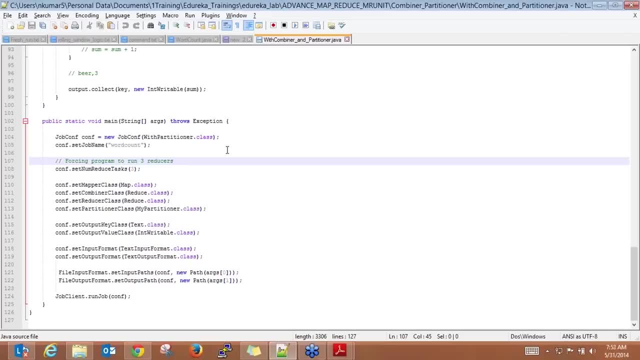 normal programming, where you basically start the whole execution and then you run the job. So here, in this example, what we want to do is we want to write our own partitioner. So what we want to do is like: let me take one example here: 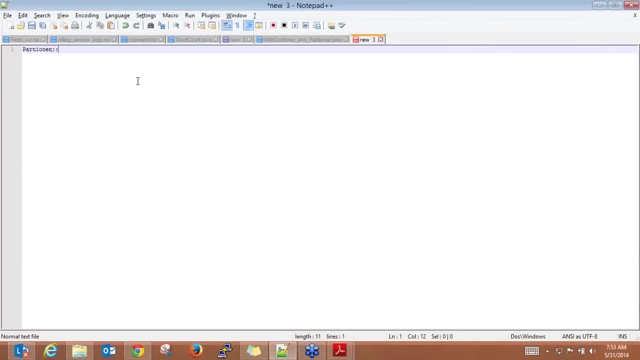 So we want to write our own partitioner so that we can define data, how our data is going to be divided between the different reducers And the reason we want to like. once you will see that how the division happens, it will give like in the practical scenario. you want to basically control it so that you can like. 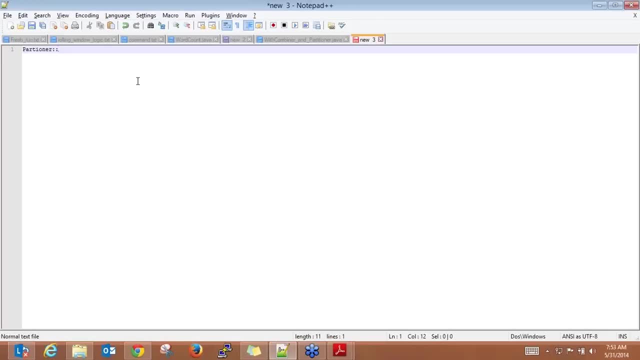 suppose, if you want to like segregate your input data set into different output file, how you want to do that, You will be controlled by using the partitioner logic. You will be able to move all the data set to the different file so that you can take that. 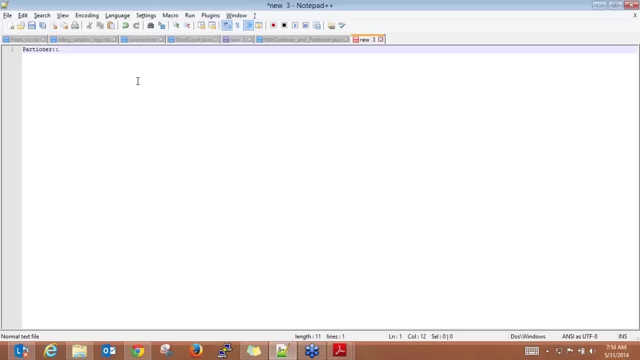 particular thing and you can export it or load into a table or whatever you want to do that. So in our case, what we want to do is like, suppose, if you have a given input line, like this is my Hadoop world. So suppose, if you have these two input lines and if you want to decide if the partitioner 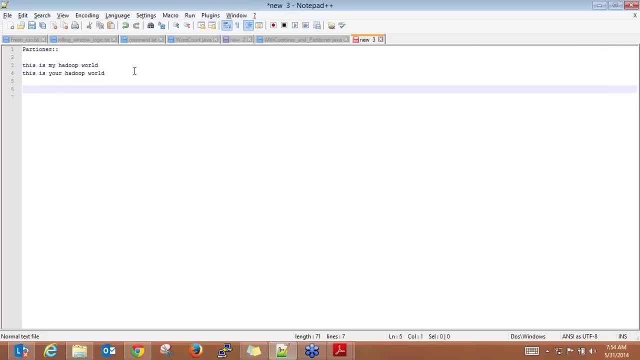 that all of these keywords like this, it has to go to reducer number one. It will process only this keyword called this And like, suppose, reducer two it's going to process- maybe you know- Hadoop. this particular has to process with Hadoop. 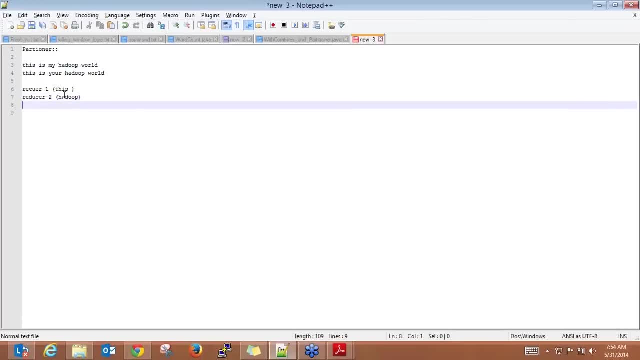 And then you will have the reducer three, which will be basically having the world data output. Now, if you want to do it like this particular way, you can write in your own partitioner and you can control that. And the reason why we go for this kind of things is like, suppose, if you are processing, 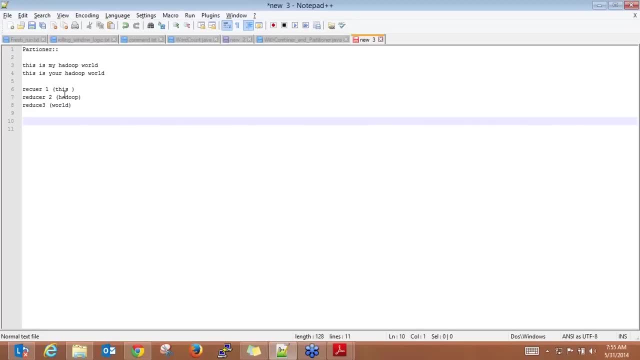 input data set where the key is like, based on like. suppose, if you have, you know a kind of a code, A kind of a data set, like where you have for each company, ideas, right? Suppose, if you have, you are catching to the multiple vendors and each vendor has a company. 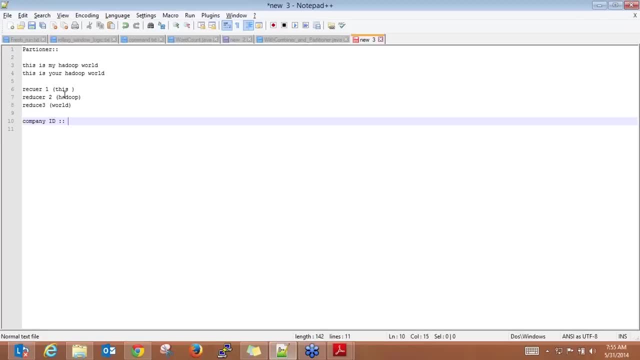 ID and you have couple of the transaction coming from them, And all these transactions is like one input data set. Now, while you are processing, you want to make sure that what were the aggregation you are doing for, like if this particular vendor you want to determine, you know how many. 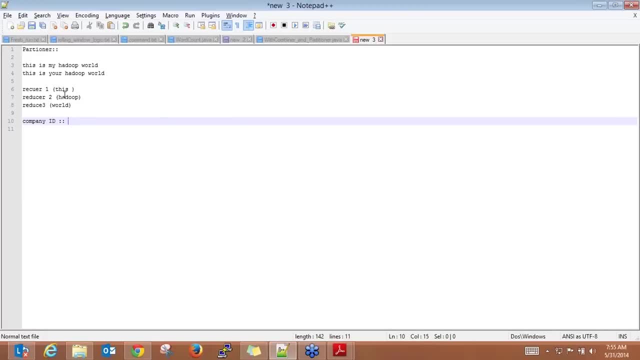 times they met the- you know the purchase order or how many times they were able to supply the things on time. But anything, if you want to do those kind of things, What you can do is you have to basically bring all those data set together and then the processing. 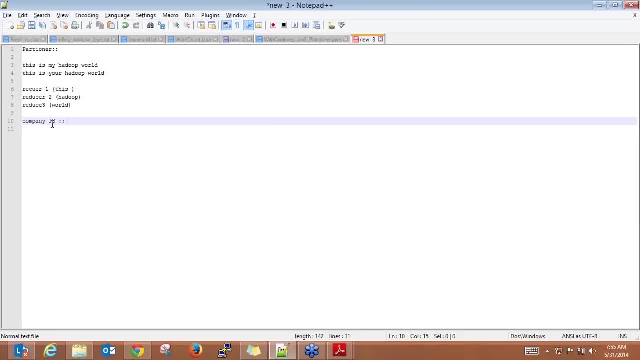 that Now, while doing that, what you can do, that you know, if you don't write in your partitioner what will happen: this company ID. it will go to the hash function and it will go to some reducer and it will do the processing. 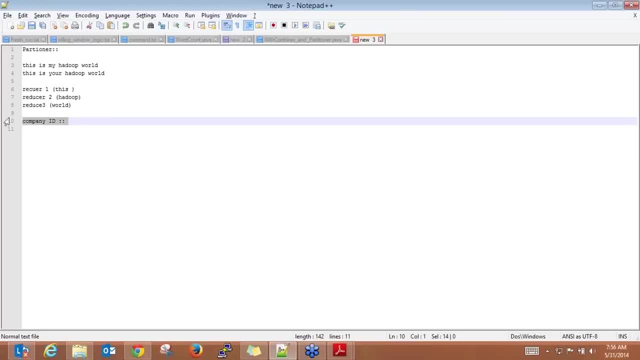 Now, in that case you will have the mix of the data because that particular reducer can have other key which has the similar hash value and it can. you know the process, that as well. Now, if you want to vary, specific, Like you know that you have the 10 vendors and you want, when the input suppose what? 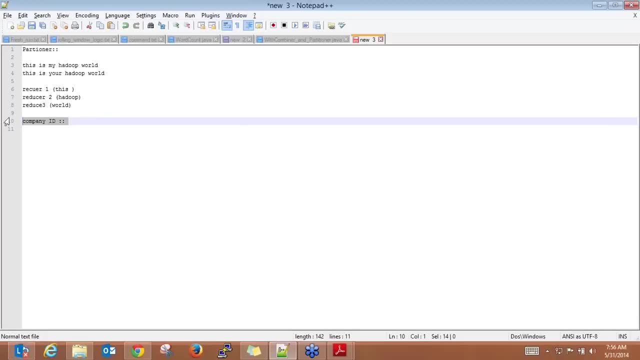 were the 100, 200 GB of data you are getting. when it comes to the output, you want to basically separate it out, all the data set into the different output files, so that you can take that file and you can process that. So how you can do: 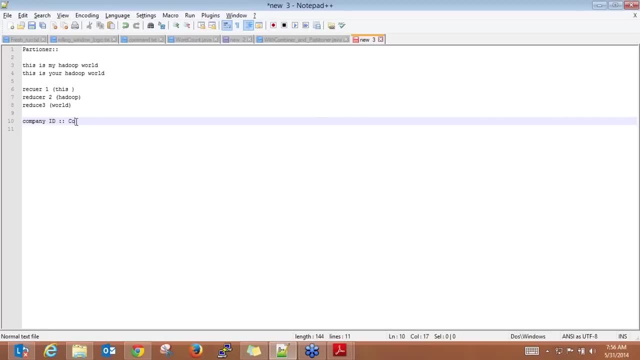 You can write, you know a custom partitioner and you can tell that anything is starting with the company one, it has to go to the reducer one. That anything is starting with, like the vendor two, or you know a company two, it has to. 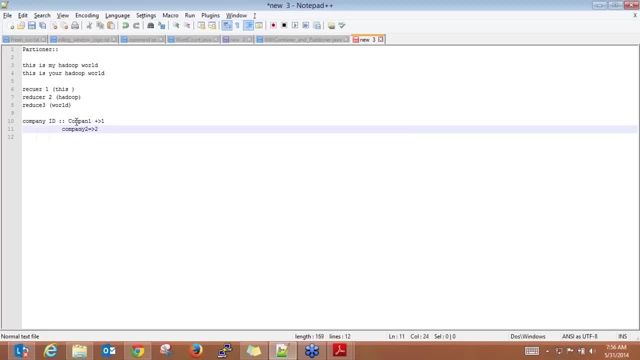 go to the reducer two So you can specify how you will specify. I'm going to show you in the example. So once you specify this kind of the logic right how your data partitioning is going to happen, your whole, the whole data will get processed with this particular logic and 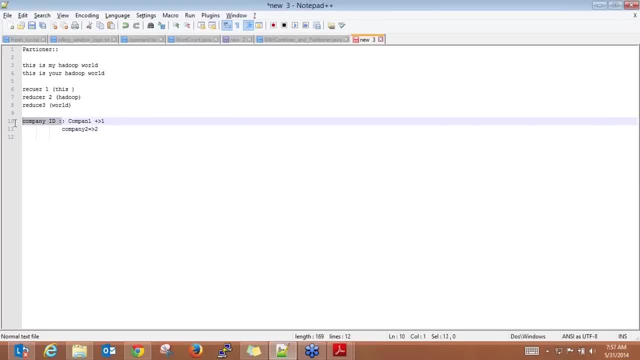 you will have all these different files. So it will have one file which will contain all the details about all the input data set: output data set for that company, one which will process by the MapReduce framework, And similarly for the other couple like vendor two. it will have another file where you will 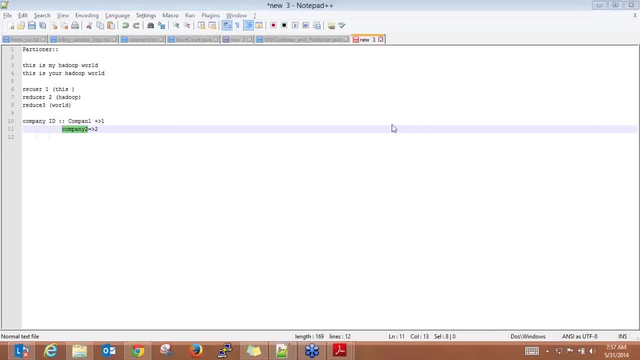 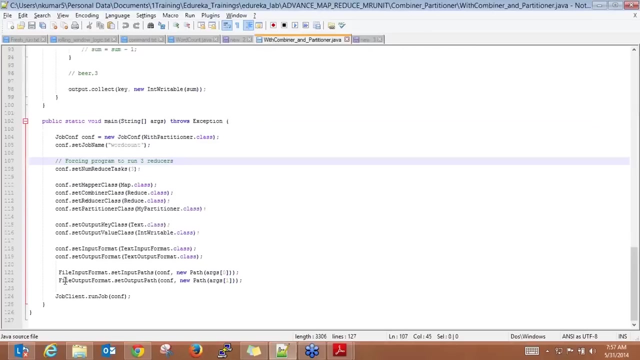 have all the data set for that particular vendor. okay, So now let me show you like how you do inside the program, how you basically write this one. So you get this like you MapReducer class, you write it and then you specify that you 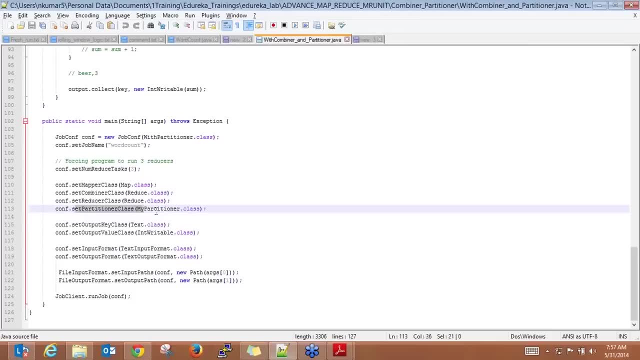 are going to implement your own partitioner. So you specify like set partitioner class and you are telling that, okay, I'm going to implement something called my partitionerclass and you are going to write a logic how to basically partition this particular whole input data set. right, 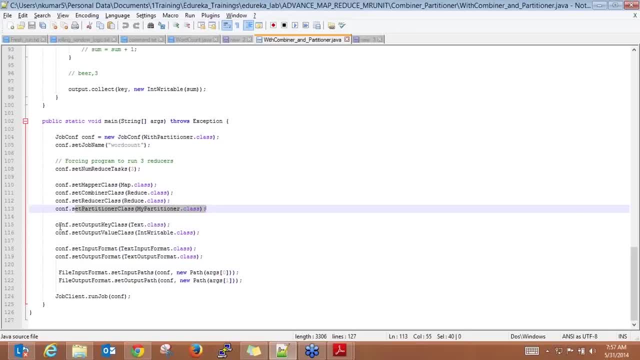 So we will see how to do that, okay, And then you see, like, what is the output key class? so it is the text which is going to be output and the value class is intratable. So in this case what we are doing is, whatever the input data set we are giving, like this: 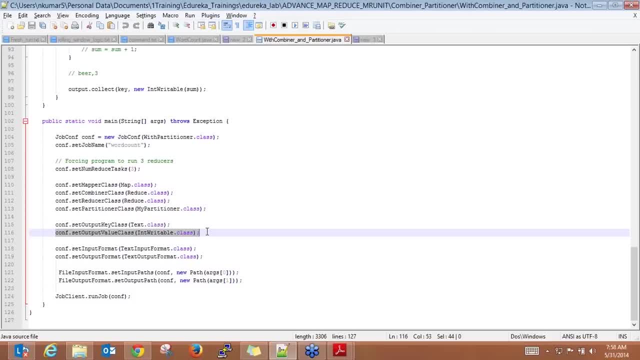 is my Hadoop world right. So in this case we want to count each word, but whenever we are counting we want to make sure the output, So the output of each word, it goes to one particular reducer, like if it is this: it. 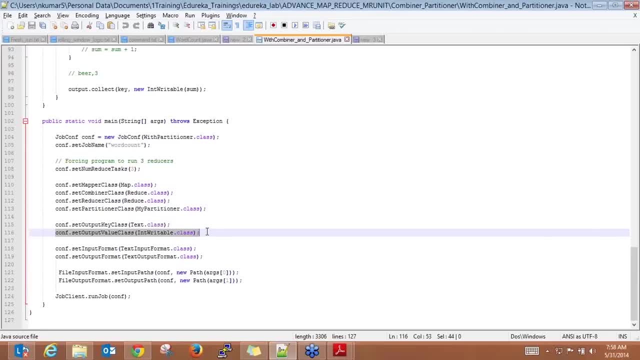 has to go to the reducer number 0 or 1, if it is, it has to go to the reducer number 2.. So that way we want to control how the reducer- which reducer- is going to work on given input data set. okay, 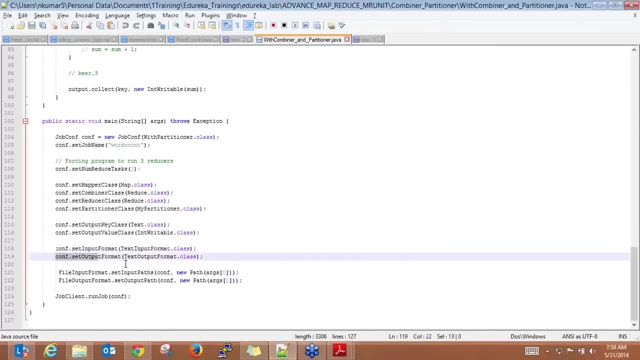 And then you have the input format, the text input format, the data which is coming and the output format. again text output format. whatever the data is coming, we are going to write into the output folder And then the input file format. it's again. we have the argument 0, that's the input. we 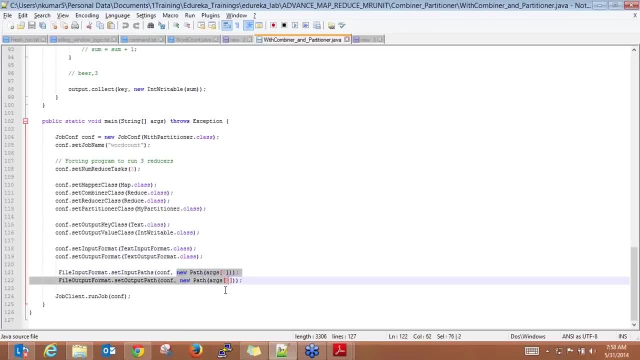 are going to take and argument 1, that's where our output is going to be stored And how to read this data. that is something set here like text input format, so we are going to read the data as the text. So what it means that whatever the input data set we will get, it will start line offset. 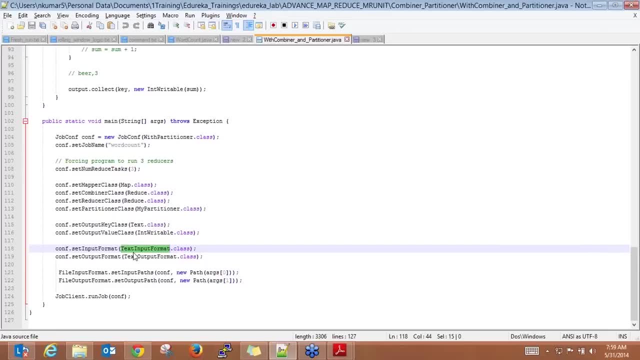 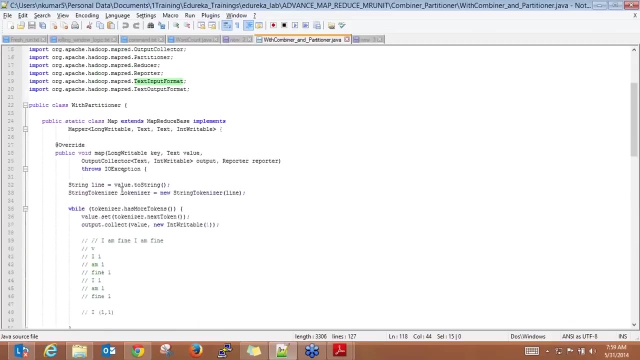 as the key and the rest of the content in the new line as the value. So that way we are basically telling our program how to read that input data set to process that inside this particular program. okay, Now the logic for the mapper. it's again going to be the same, what we have in the previous. 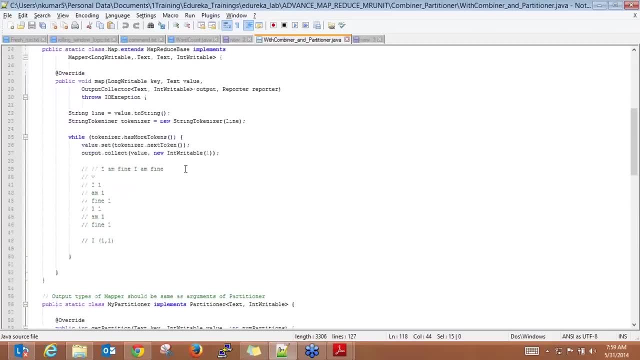 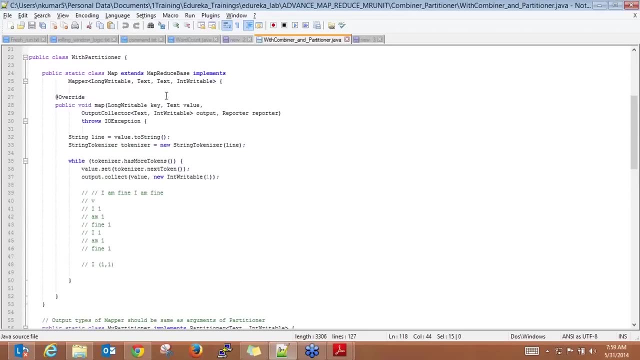 class. So you basically implement the map method. you have the key long writeable as the key, line, offset as the key and the text as the value, And what output you get is basically set of the like: the list of the key and the value. 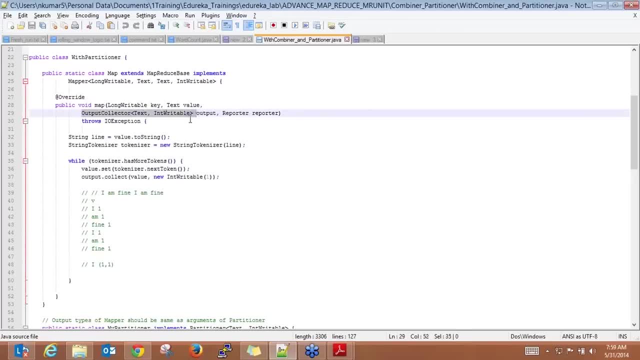 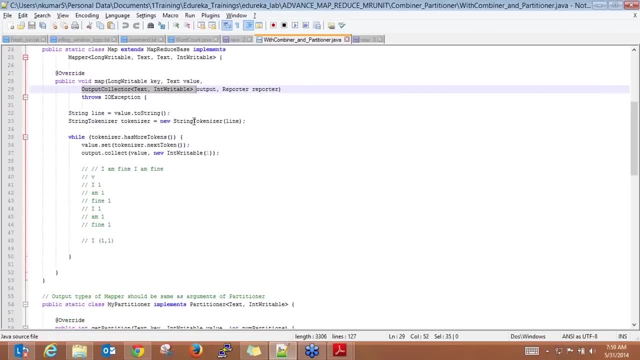 pair so that you collect it using output collector, where you have the text and the value, Okay, And for each of the line when you get, you convert into the string. and then, once you convert into the string, you basically do the tokenizer. that is like the space or the tab. 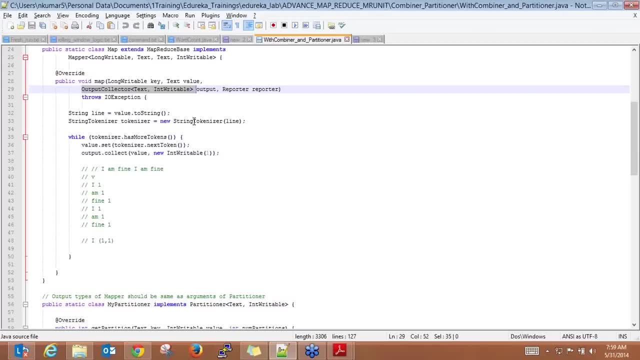 or the comma you can define, like how you want to tokenize the word. In our case, we are just using the default one. so by using the space, we are tokenizing each of the word And once you have that one, what you are doing is for each of the word you are setting it. 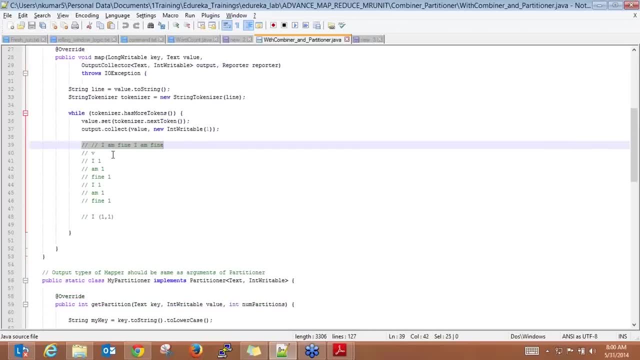 like this, like. suppose the input line is: I am fine, twice, it is repeating. So in this case, what will happen? Each of the word, it will get output like this, Like this way. So now, instead of passing all these values, like this particular way, like each, like, in. 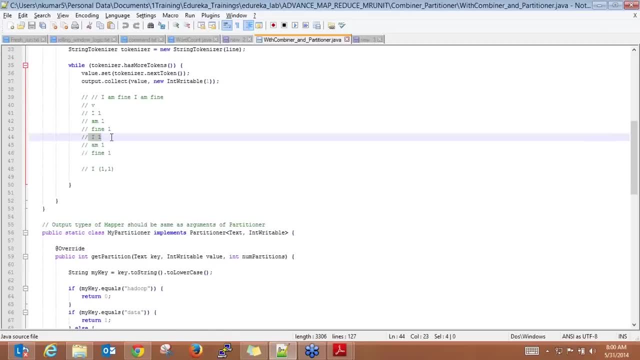 this case, you see, I is one and I is one. So instead of passing all these I one and I one- to the reducer, what you can do is you can write a combiner. and what the combiner will do? it will basically combine these two outputs coming from one mapper and it will pass like I two, and that will be the value. 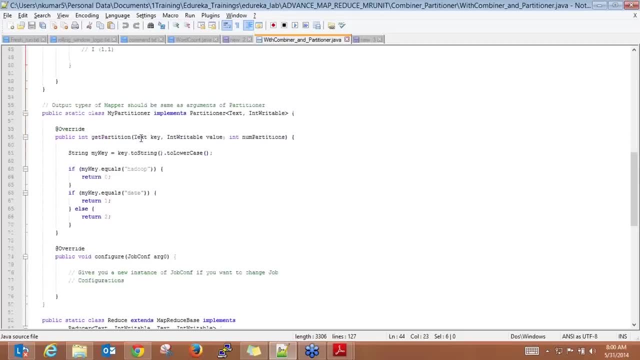 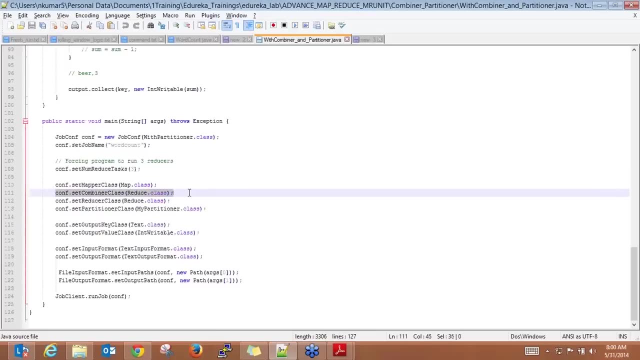 it will go to the reducer. So how you implement that one is: if you have noticed, in the driver class what we have is that we have set the combiner class and that is similar to whatever the function you have written for the reduce. So in this case, what will happen? it will call the same logic to aggregate this value on. 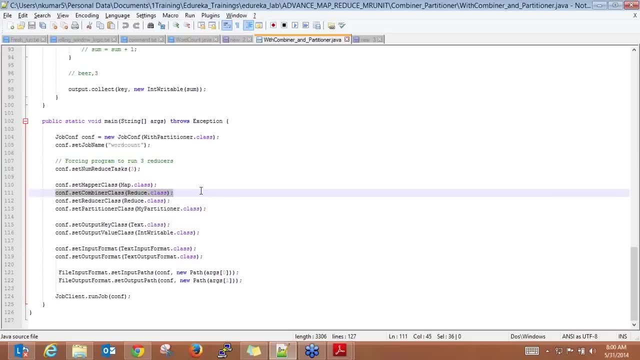 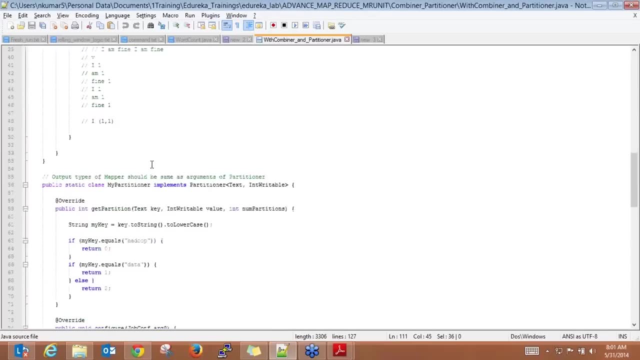 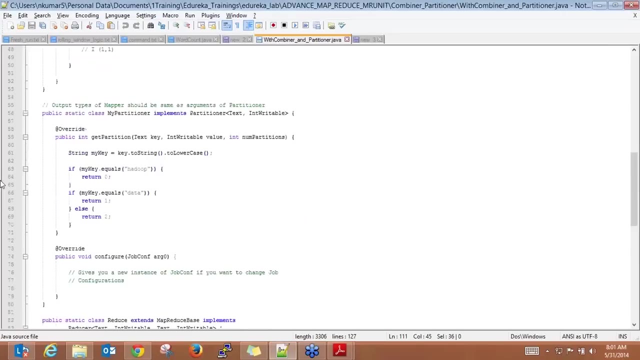 the mapper output, and that's the output which will get transferred to the reducer. And then what you have is you have this partition logic. so the partition logic is the logic which is actually going to determine how your data is going to be transferred from one reducer. 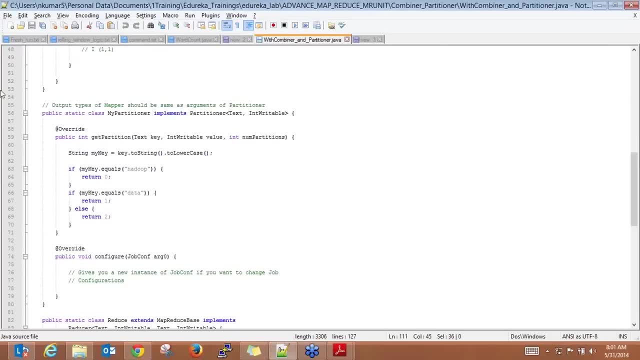 to another reducer. Okay, So what you can do is you can implement this partitioner. so all you have to do is you have to use this get partitioner to get the number, like, which will be the number between zero to the number of the reducer which you have. 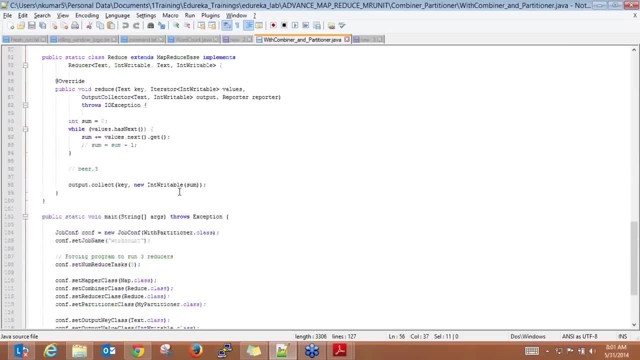 So in our case, if you see, we have set the number of the reducer, task three. so I think somebody had the question right how to set the number of the reducer so you can see inside the program itself you can set how many number of the reducer you want to run. 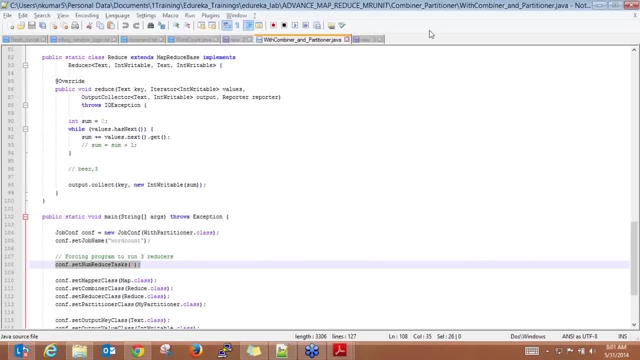 Yes, Satish, your question. yeah, you got answer. okay, When do you people go and change the partition? that's what I'm explaining, Meenu, here, like when to change the partition. okay, and I'll show you okay mobile number: every number has ten digits- how we can process this. okay, I will come back to your question, Satish. yeah. 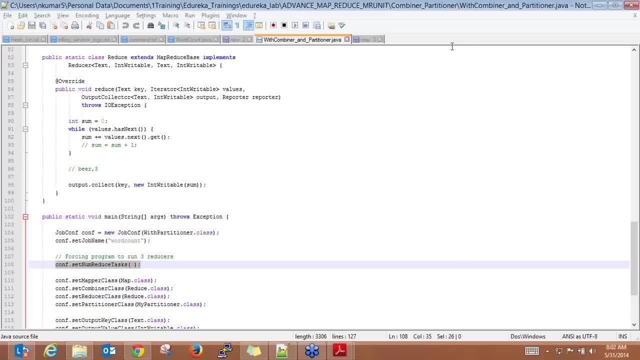 okay, So the partitioner can be used only for custom data streaming using the mapper reducer. yes, Satish, yes, Okay, You got it, Meenu. yeah, so now what you are doing is by using this set number of the reducer task. you are telling that, okay, I have like three reducer which I want to run, so give. 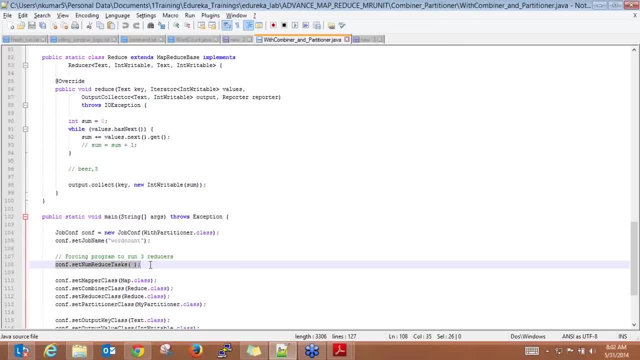 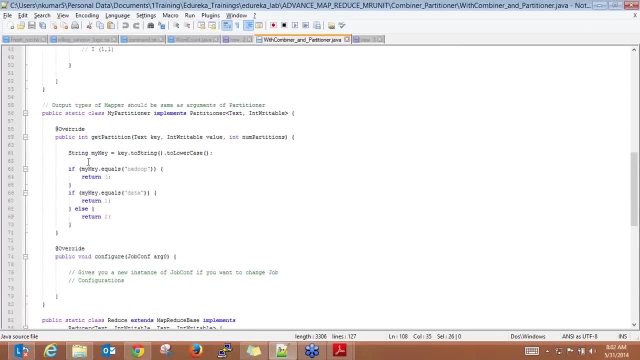 me a number between zero to two and based on that I'm going to determine that which reducer I have to output the data. So now what you are doing is like to determine, like how you want to do so, one by like, that you take the key, you calculate the hash value, you get a number and based on the number, you 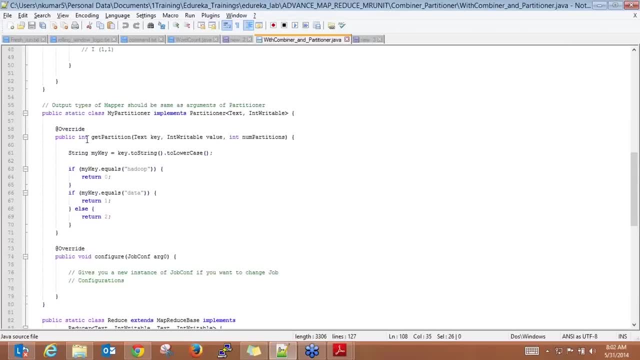 determine which reducer it has to go. there is another way. now what you are doing is we are writing our own method how to do that, and that is using the get partitioner. So, by using this get partitioner method, what we are doing is we are going to get what is. 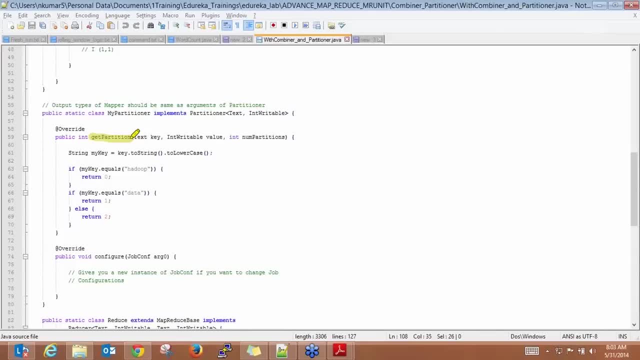 the reducer number where the data has to be. you know, flow from the mapper to the reducer. So how you implement this: get partitioner, is you get the key. whatever the key you have, you are converting here into the lower case so that you can do the comparison. so you can. 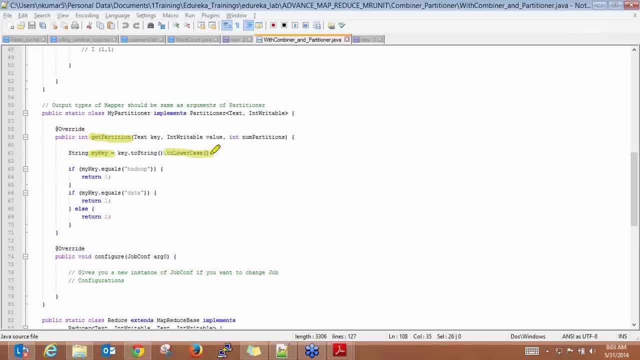 have the case sensitive. in this case you can have the case also and then that way also, data will get processed right. so in our case what we are doing is we are converting the key to the lower case and after that what we are doing is we are saying that, okay, if 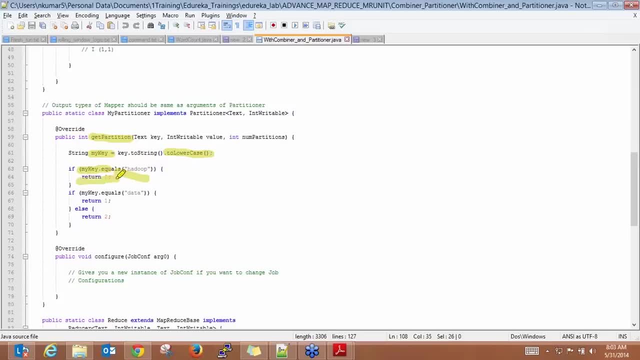 my key equals to hadoop. send it to the return, a value called zero. so what means it? send it to the reducer number, the first reducer which we have inside the cluster. if the key value is equal to zero to the data, send it to the reducer number two which we have inside the cluster. right? 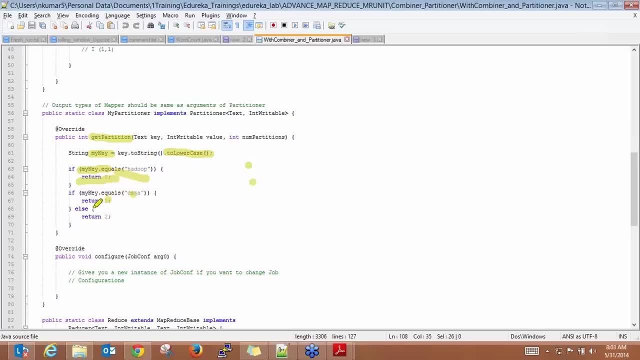 so that's why I'm telling you, if it doesn't match all these hadoop and the data, send everything to the, you know the default reducer, that is, reducer two, and where it will get processed. So, number of the reducer: we had the three, so zero we have put the logic one. we have. 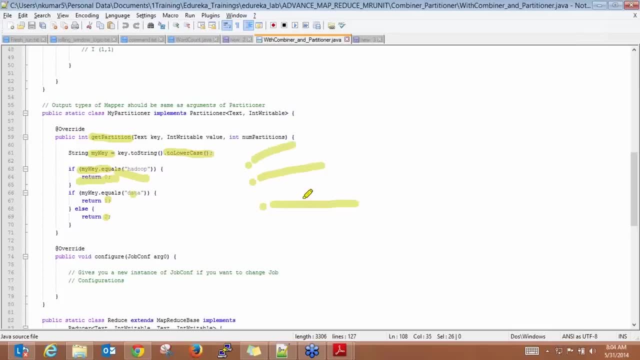 put the logic and the third. we have put the logic that default everything will come to the reducer three. So if any word or any key which will be equal to hadoop, it will go here. anything which is equal to the data, it will go here and rest of the things. whatever the key is, it will. 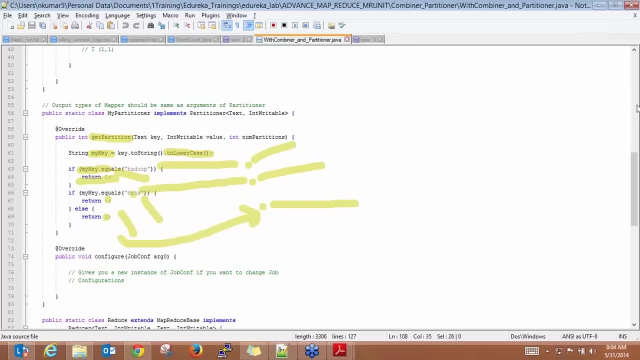 go here and rest of the things. whatever the key is, it will go here and rest of the things. whatever the key is, it will go here and rest of the things. whatever is not processed, all this will go to this input data set, So that the way you will, so, in this way, what you are going to do is you are going to you. 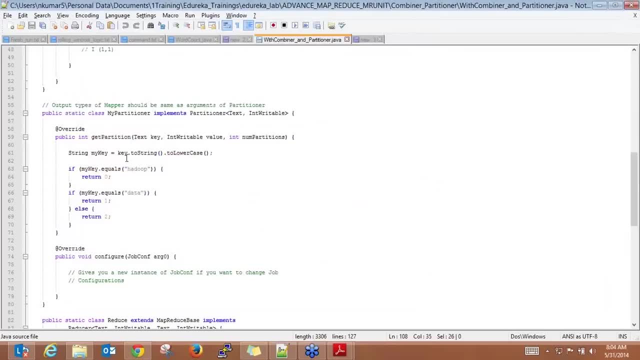 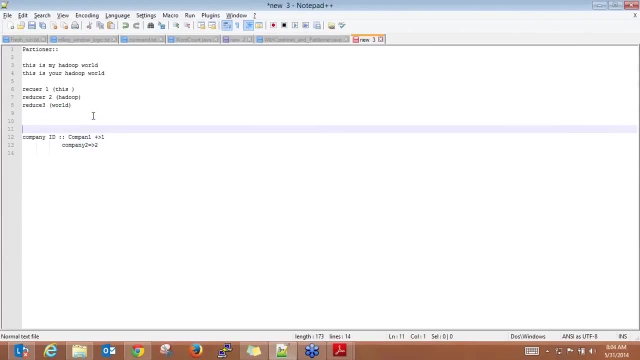 know, make sure that which particular reducer is going to get you know which input key right. so if you see here this particular example, get partitioner. here we are not using the hash value which we discussed earlier. So here the hash value was, like you know, for a given key, like, suppose. if the key is like: 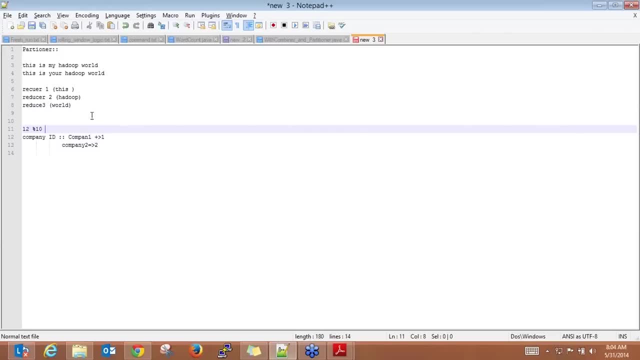 12 and you have the number of the reducer as 10.. So if you calculate the modulo by using the default, so what will happen? you will get a number two and that is the hash value. you are getting as two and based on this, you will 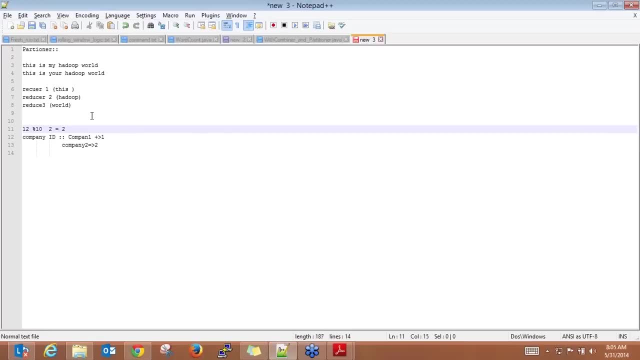 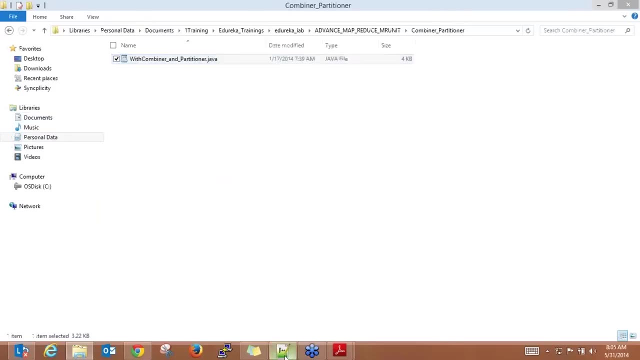 tell that. okay, the second reducer, it has to go. Now, instead of going for this particular logic or divide that we are writing our own logic. and that particular logic is like: okay, if the key, if the input, is equal to the number two and the output key is equal to this particular word, and that is the custom partition we have. 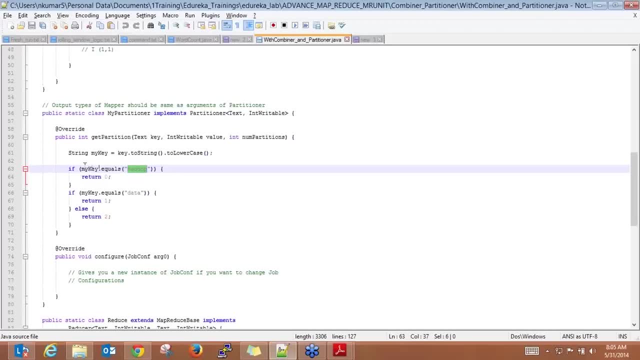 we are not using that. you know the hash value to calculate. here we are writing our own key. So you get a key, you compare it with the value and based on that you are returning it a number, and that number is basically nothing but the reducer number where it has to flow, that particular. 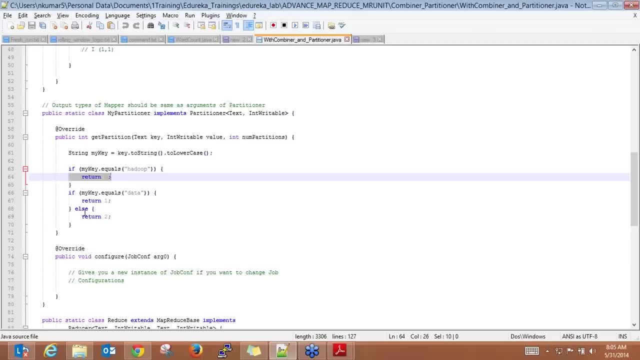 output of the mapper to this particular reducer. So that is what you are implementing in the custom partitioner? Yeah, it is a function provided by the MapReduce framework that you have to override. yes, So all those things, like all these things, will be getting provided to you by the Hadoop. 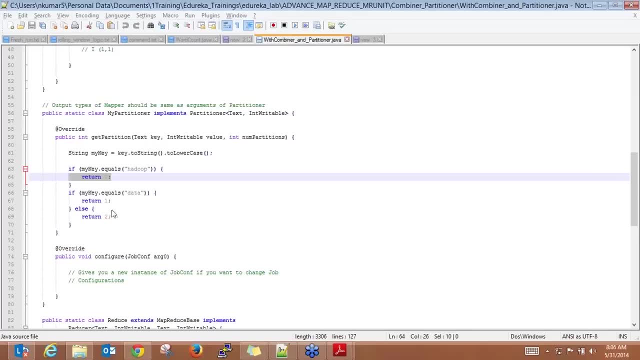 framework. Sorry to ask, but can you tell me what is the hash value? okay, actually hash value is nothing, but you know how you calculate. for a given key, you calculate a unique value out of that. so one way is the modulo. So there are other functions. by using that you can come up with a very efficient hash. 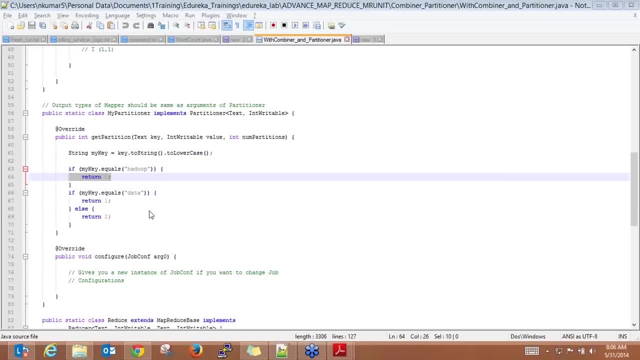 value and that will you know, a very unique or it will not repeat those kind of things, right? So there is a lot of like when it comes to the data distribution. you use all this hashing algorithm to come up with a value for a given particular key. 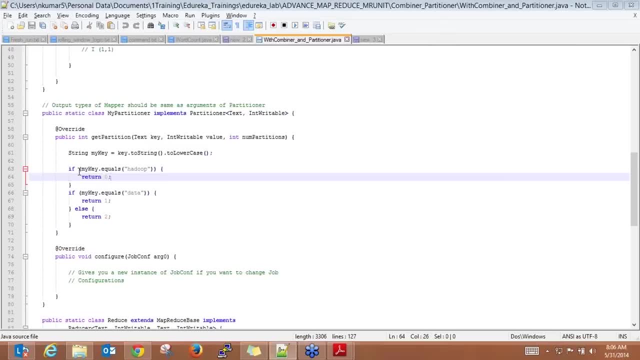 So in our custom partitioner we are not using the hash value. that is what I am saying. So here we are writing our own logic that if the key is equal to this particular word, then move this data to the reducer two. Reducer: zero, one and two. 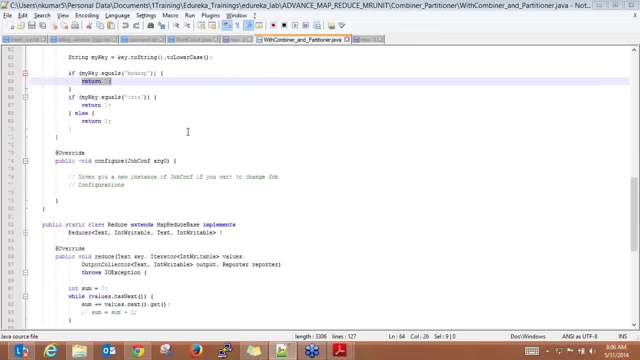 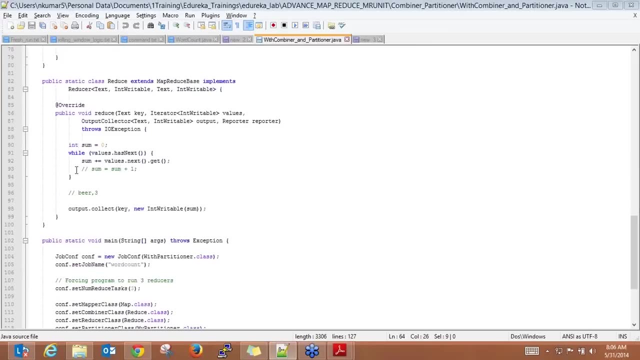 Reducer zero, one and two, And then you have this reducer function where what you are doing, again, you are getting all the value and till you have the value, you are doing the sum and once you get the sum, you will, you know, basically output that value and you will get the final count of like how. 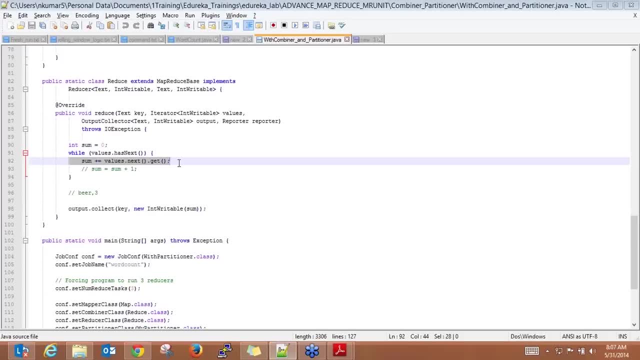 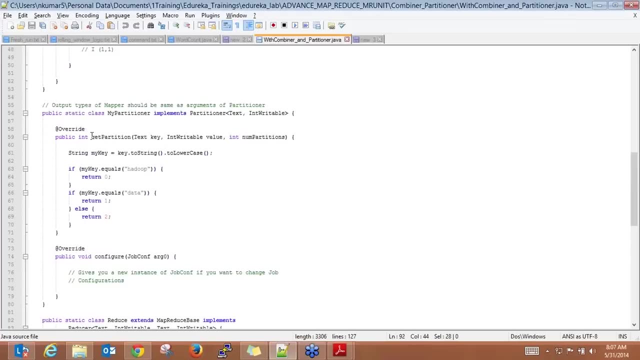 many times each word had occurred inside the given input data set. So the core of this whole implementation is where I want you to focus in, like how to implement this partitioner. So that's what you are doing using this. you know the get partitioner. you are using this. 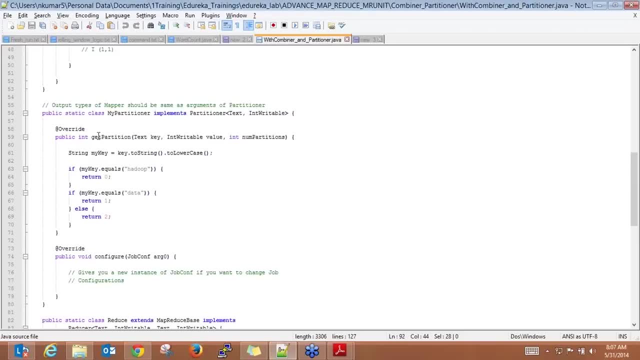 particular method to get the partition number or the reducer number where you have to move the data. So, using this get partitioner, you are implementing your own algorithm, how to get that particular partition number, and the logic is we are comparing each word. so we want to be saying of control. 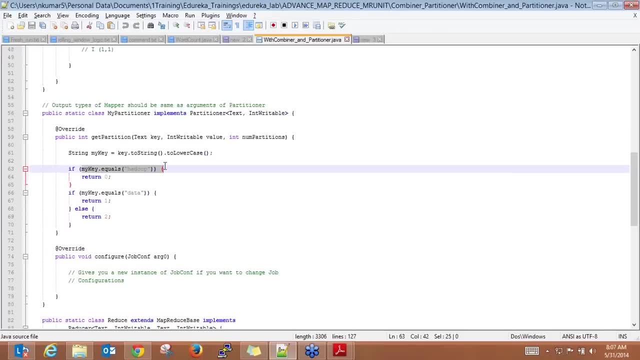 based on the each key value. So these key value has to go to this particular reducer. So if you take this example, what we were discussing earlier, So suppose if you want to be based on the company ID, so what you will do is like, suppose, 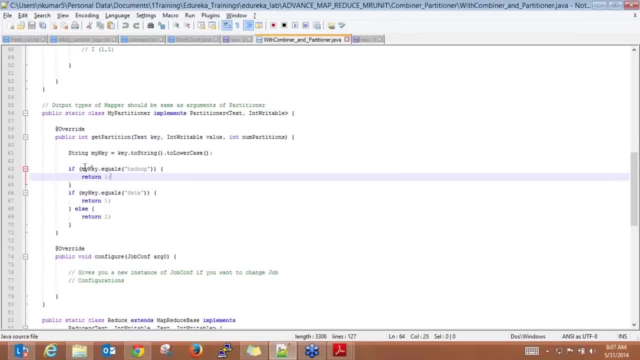 if you have the 10 vendors. So for each vendor you will. each vendor you will tell that. okay, if the customer ID is equal to this particular thing, maybe the vendor one send it to this particular reducer. if customer two send it to the reducer two, 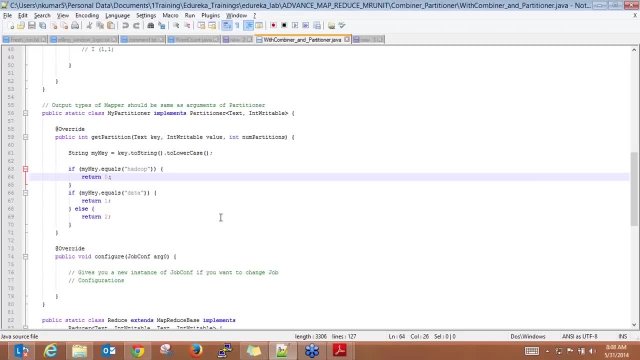 So that way you will be able to control how the reducer output is going to be there, So how basically whole MapReduce flow is going to output the data set and then, if anything doesn't match with this particular thing, what you have put, it will go to the default reducer. 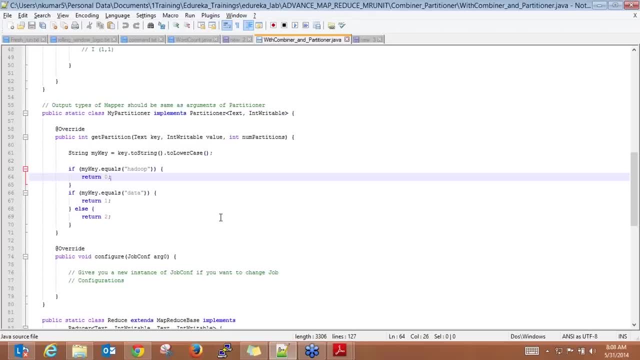 and you will be able to get the output there. So that way you implement your own partition. you are not using here the hash value to just move the data, but instead you have put your own logic how to move the data and based on that your program is going to work and move the data between the mapper to the reducer. 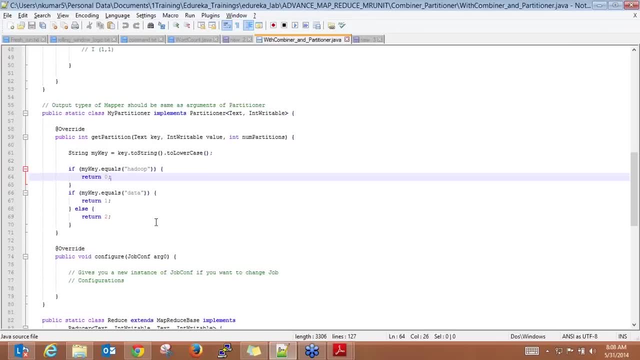 by using this particular algorithm. So now, what I will do, guys, is I will show you, with an example like, how this thing works, and I think that will give you the clear sense How you are able to control. Okay, So, using this partitioner to the output, right? so let me bring the virtual machine here. 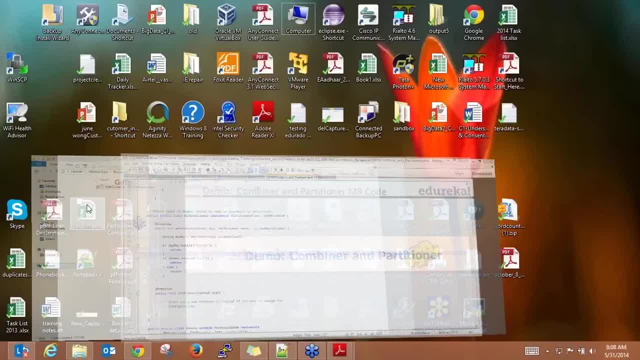 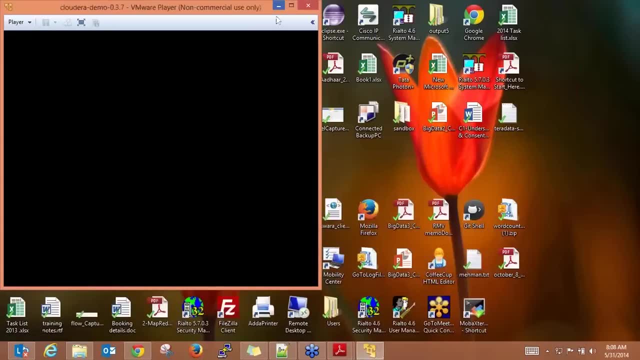 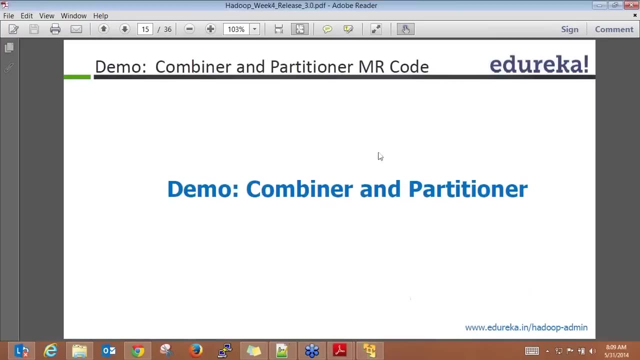 Okay, let it come. So what it says: can a single reducer work on Two different keys simultaneously? okay, So what happens? Subhaji, it is like: whatever the input data set you provide to the to a particular reducer, it does a sorting and, based on that sorted data, it starts the processing. 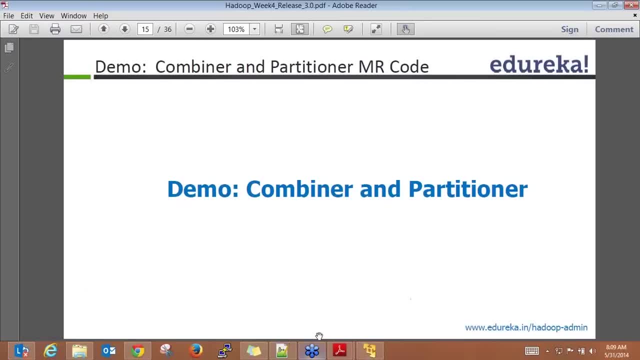 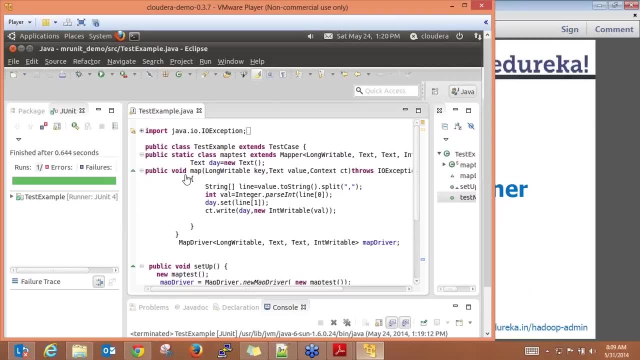 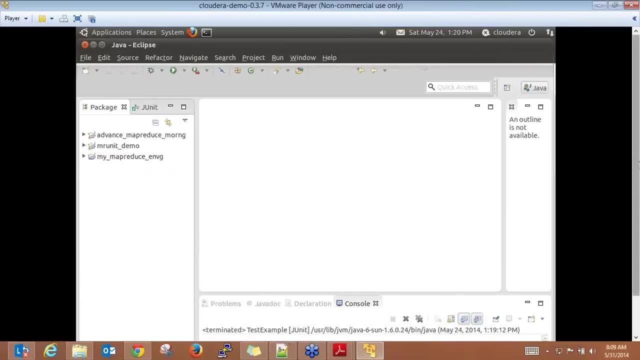 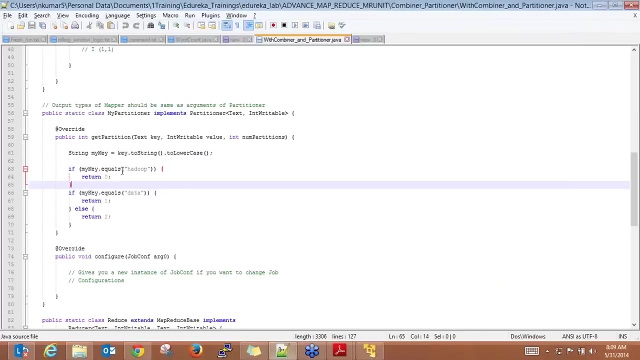 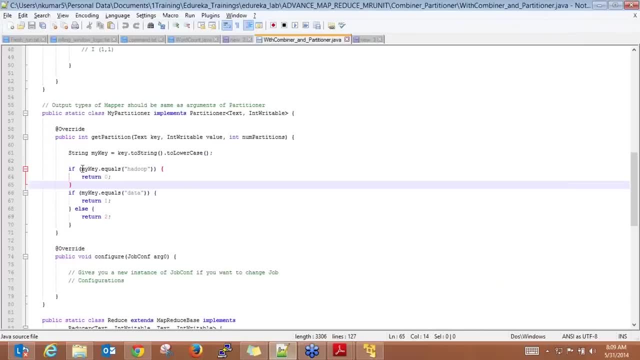 All right, Okay, Okay. So before I go ahead, Any other question with this particle partition logic, Are you guys able to get a sense right? I'm going to show you how to work that. So all the logic we are, What we have put is like for a given input key. keep our word right. 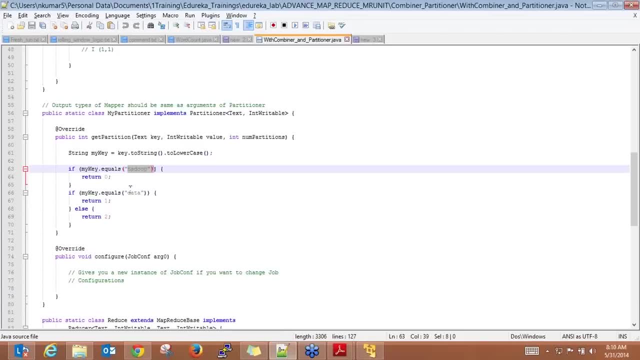 Key value peer. So we've given input key. Whatever, it has a particular value. there's a hed моз. we can go to one at user. If it'll have a new data, it will go to another at user. So that's the way we are going to put a logic here and we are going to control. 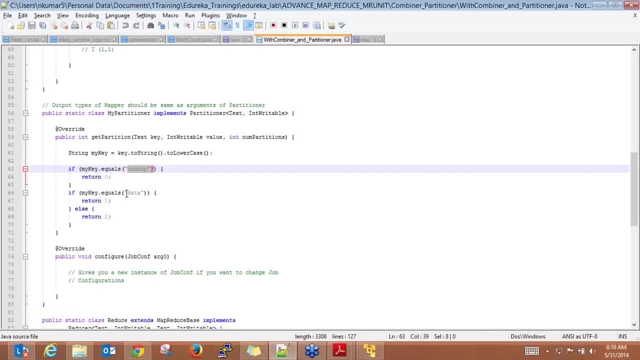 Which in this is going to get what particular input data set. Okay, so that's the logic, and we are going to control which is going to get what particular input data set. So let me come back here. so let me create a project here called java project, and then 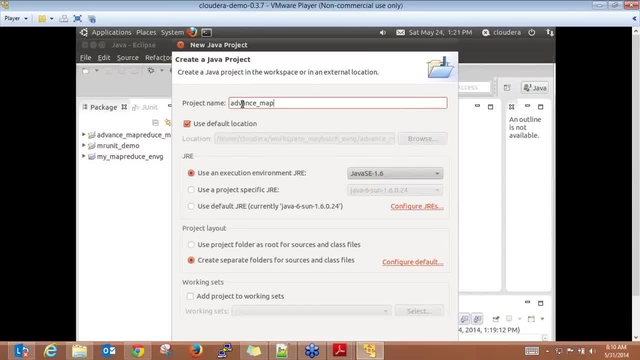 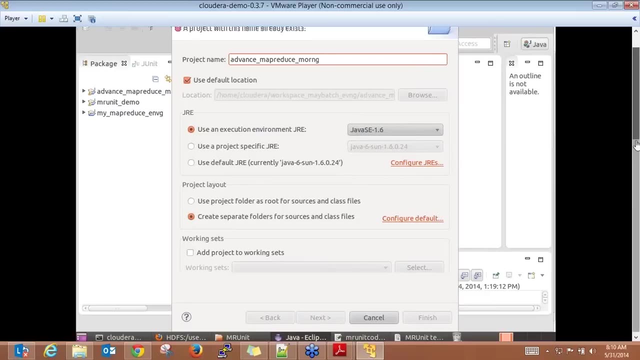 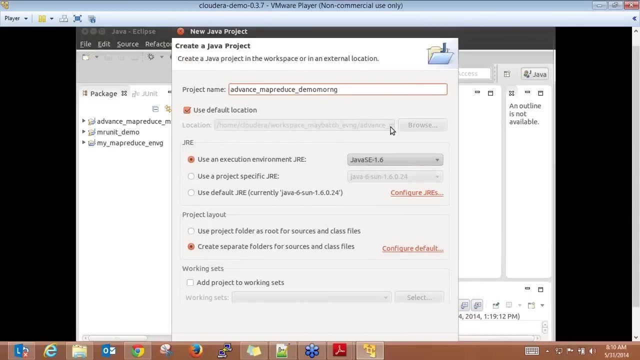 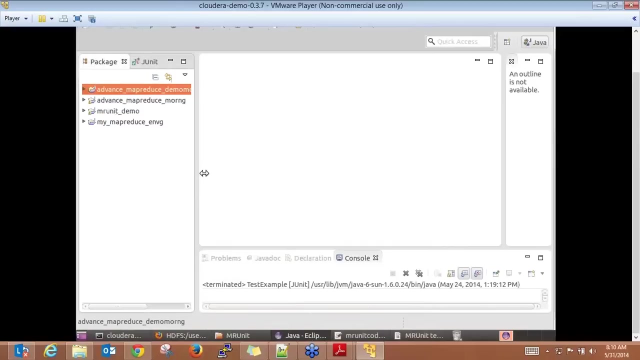 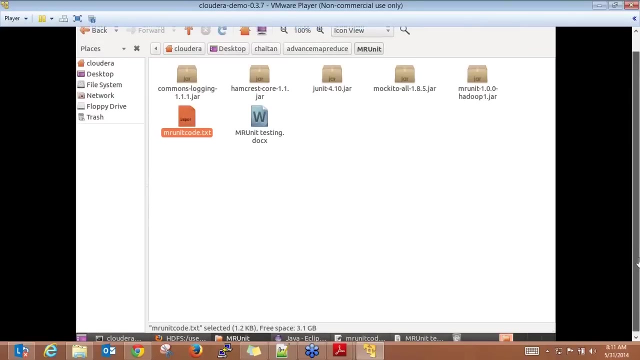 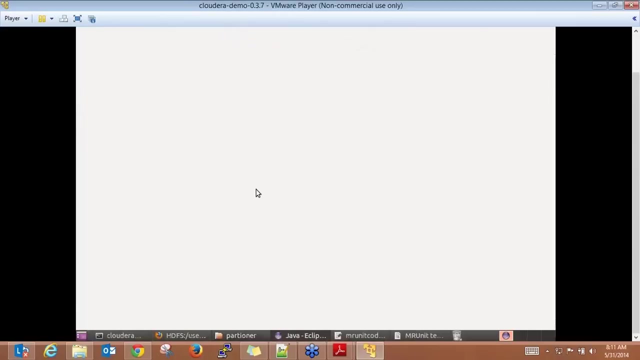 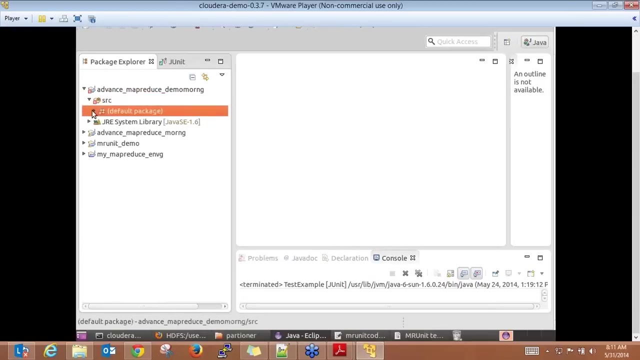 give me like name it: advance produce. oh, it's already there, okay, Okay. so now let me take this code first and then explain. all right, Okay, Okay, Okay, Okay. so in this case, what we are doing is, whatever the input data set we are providing. 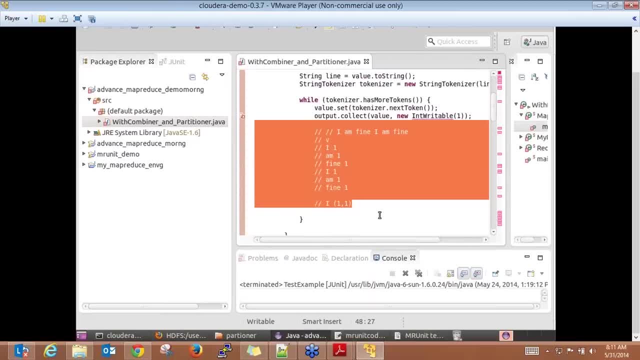 based on the input data set. if the key is equal to one particular word, we want to control where the reducer has to go. right, So now, okay, so first let's do a thing. so first let's include the jar file. so all these: 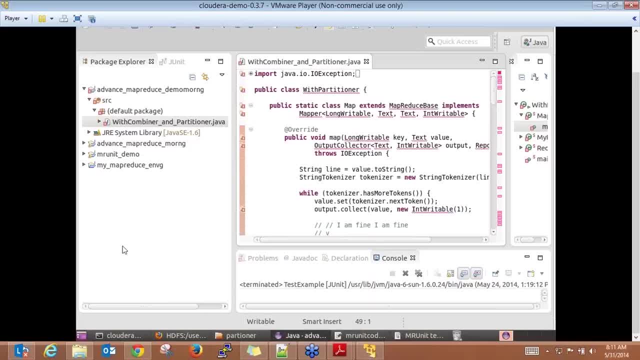 are the definitions is available And it will share these codes so that we can practice. sure, it is all these codes what I am going to discuss in the class. it will be shared in the LMS and you should be able to access that, okay. 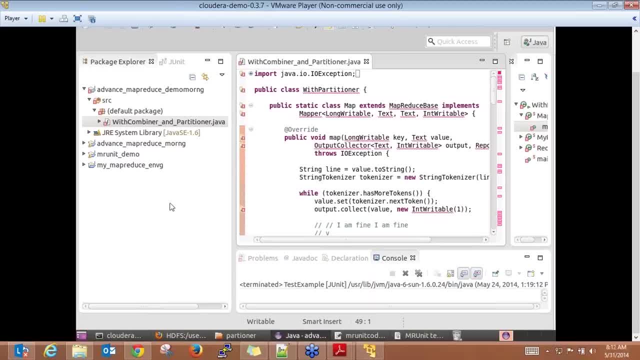 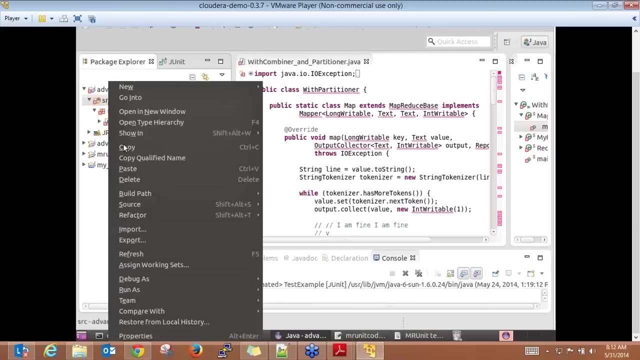 And, in case, if you are not, just check with the support team and make sure you get a copy of this code, okay, So, yes, it's all, everything will be available to you. Okay, So how you implement where the jar file is there, how you include that you do, you go? 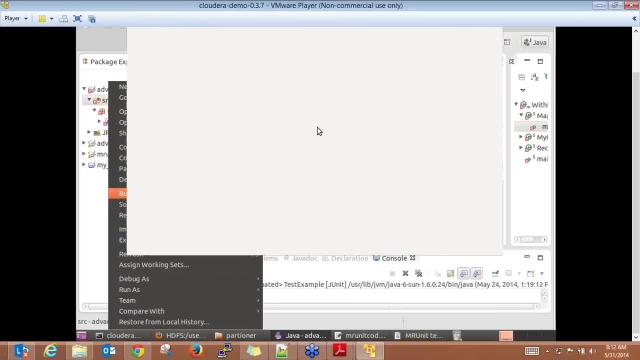 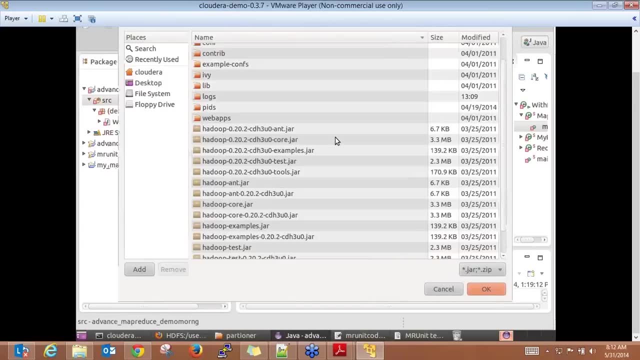 to the build path, configure build path And you have to basically include some of the code. Hadoop library is what we have, So you take it everything here. user lib Hadoop- right? so this is the user lib Hadoop. 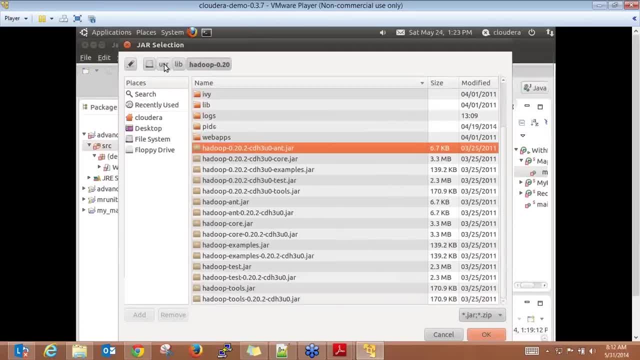 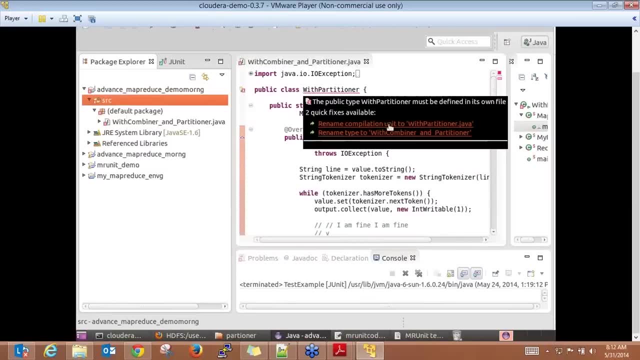 you go and then you basically get all the jar files, whatever we have you do, okay, Okay, so everything is there, okay, So we'll rename it with partition. so here, the one thing is the whatever the class you 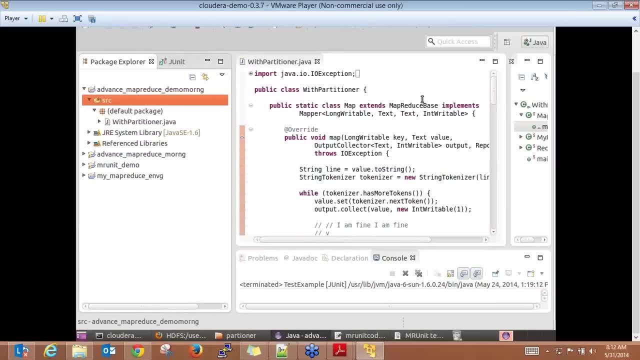 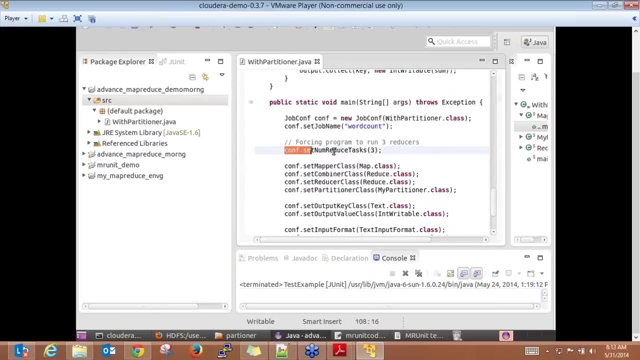 are going to write and the file which you are going to say. both should have the same name. So, in case, if you're there, you can just rename it. Okay, So now let's do something here. So how many reducer we have, number of the reducer is set by this particular thing: set. 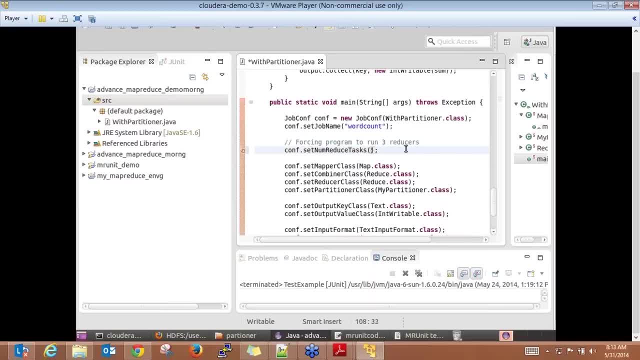 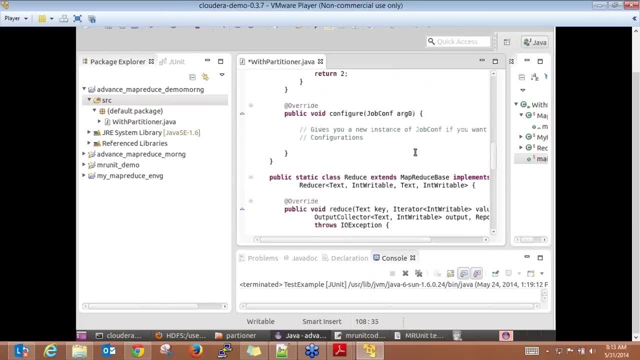 number of the reducer, that's three. So let's see that we want to number of the reducer. we want to is a five. So now what we can do is we can write our own way how the data will get transferred here. So, as you can see, here we have all these. you know the. you know the. you know the. 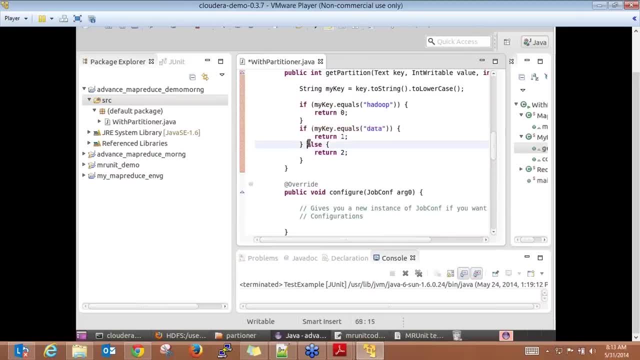 way the data has. the data is going to be, you know, let me put it here. so now we have the five partition so you can have five different way how the data is going to be transferred. So let me take some of the people who were confused here with the partitioner thing. 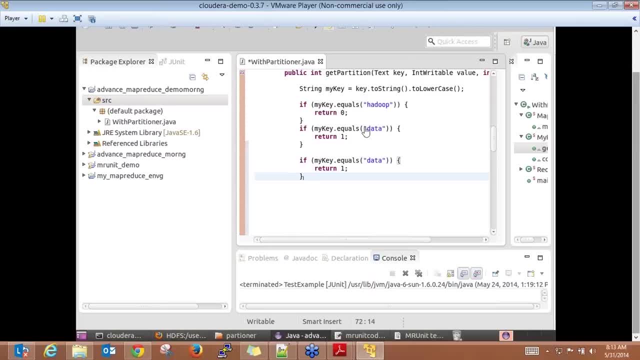 we have the questions okay, So let me take first Hitesh. okay, Okay. So what we are telling here is that if any key Okay Or any word which will have value, Hitesh, send it to the. you know the reducer number. 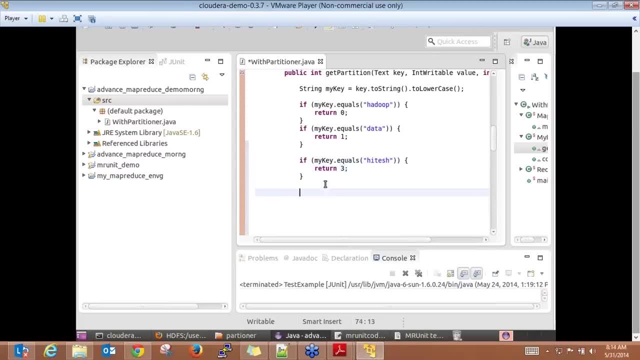 third reducer, so that will be like 012, right? So now suppose, if anything is related to you know, let me do. and so this is: if you do not mention the condition for some of the reducer, they will. they will not be utilized. 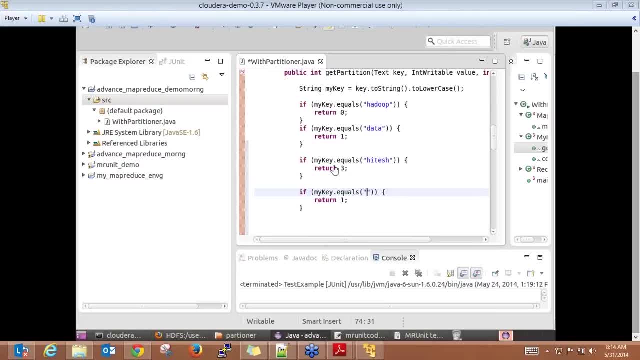 They will go to the default reducer, Hitesh. okay, So like, suppose third one is Hitesh, So the second one is like Edureka, right, Okay, But we are telling: go to the reducer number four. So 0,, 1, hold on 2, 1 sequence 3, okay. 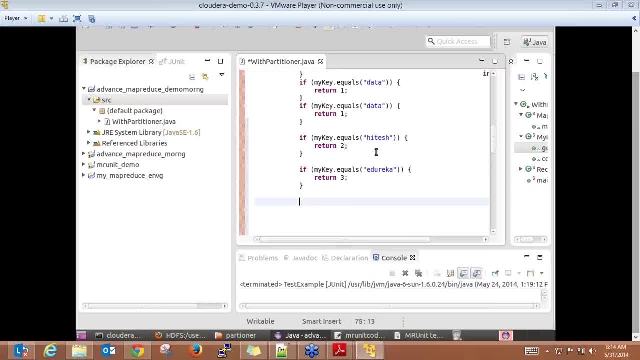 And the rest of the things go to the Hitesh. Okay, So what we are doing here? a number of the reducer. what we have is 5, right? So all the 5 reducer. we are writing a logic how the data will get distributed. 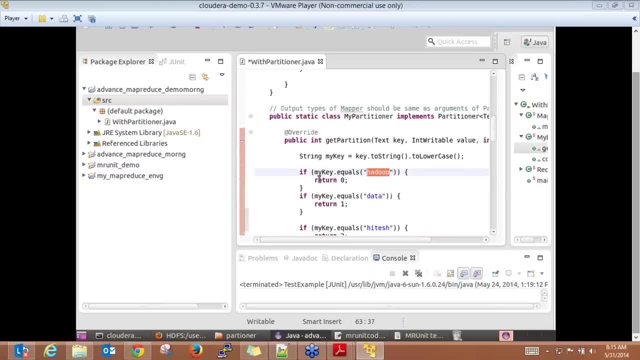 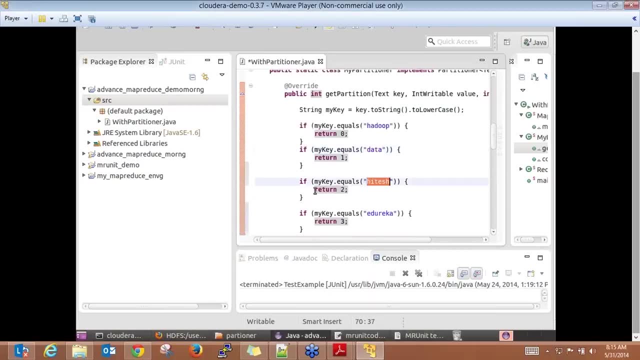 So we are telling that if the data is having the value Hadoop, it has to be processed by the reducer 0. It is, you know, the data it has to process, reducer 1. If it is like this, it has to process by the, you know, the third reducer. 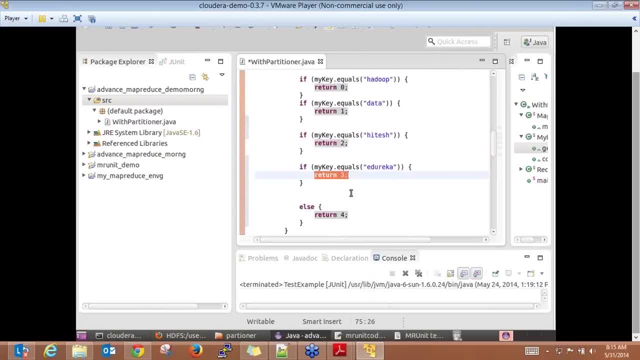 If it is Hadoop it has to process by 4, and then the rest of the things it will go to the default. So any of these things, when there's cut a measurement, it will go to the last reducer and which will basically get the multiple keys value to process that and give the output. 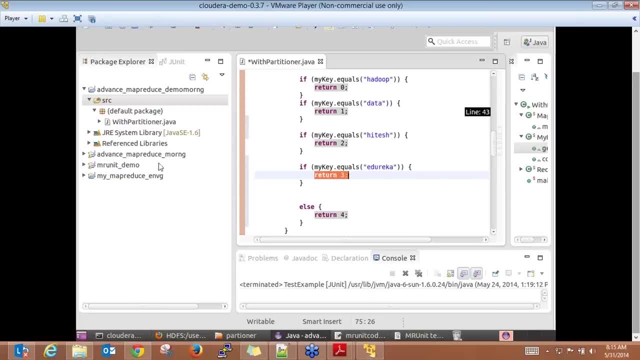 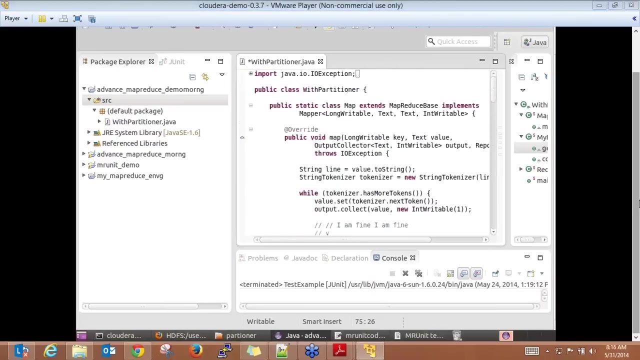 Yeah, it will not utilize this. If you don't give the output, it will not be utilized. okay, So those things. you can just try it as a piece while working on your yeah. Okay, So now what we do is: let's save this particular program, okay. 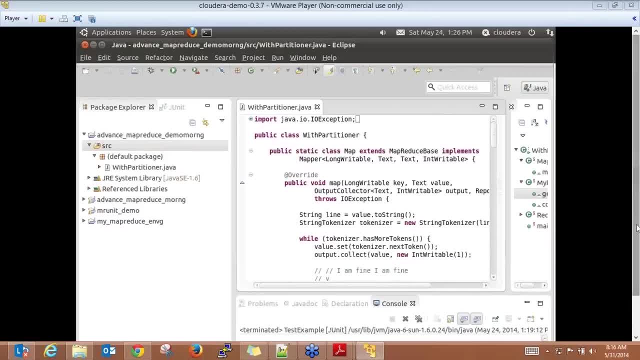 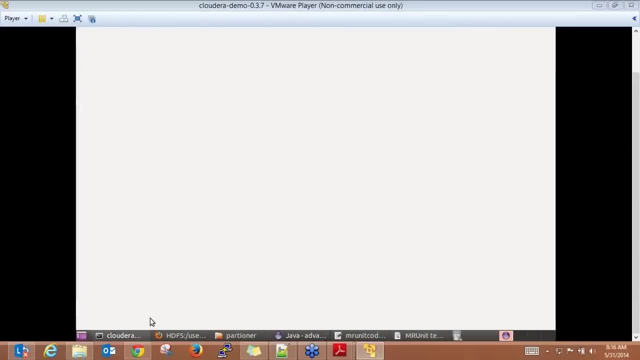 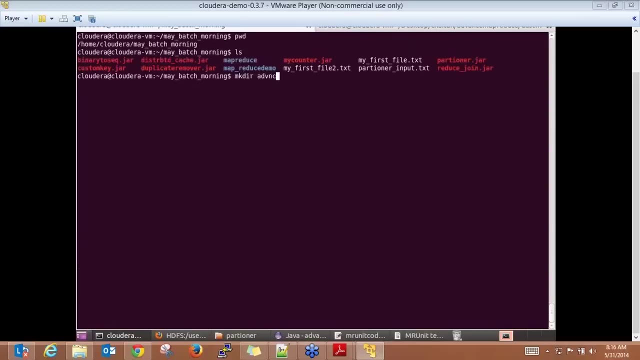 And now let's create a jar file here. So let me go here: Control L, Okay, Okay. Okay, Let me make it directly in KDIR. It runs Okay, So let's go ahead and create a jar file out of it. 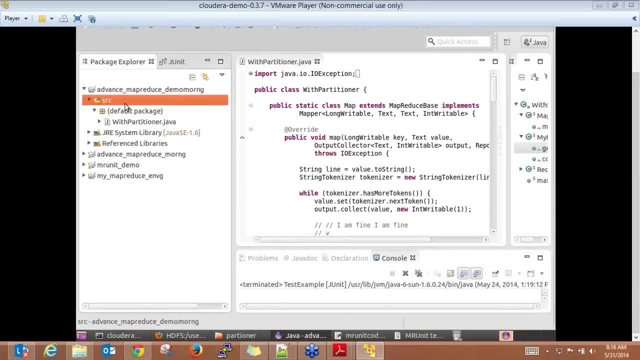 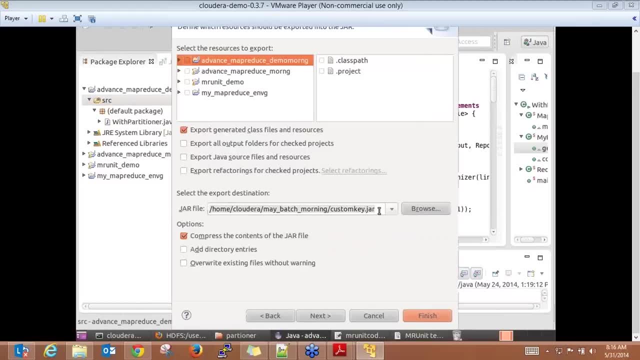 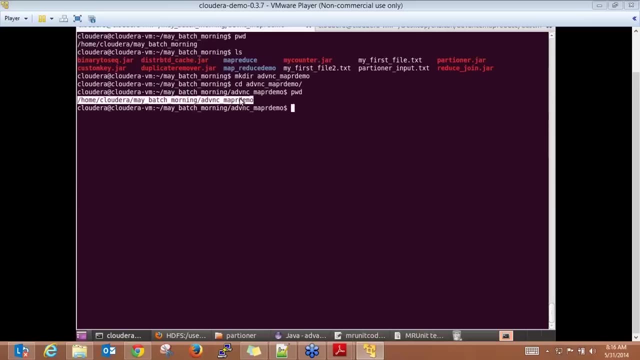 So how you do that Export And then you do a jar file Next And you specify where you want to store the jar file. Okay, So here we are going to write mypartitionerjar. Okay, So this is a jar file of which we are going to create as part of our program, as part. 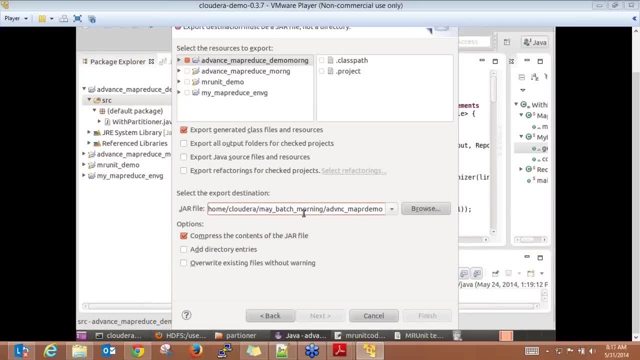 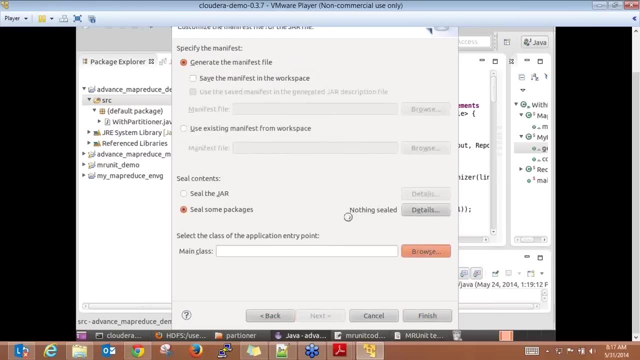 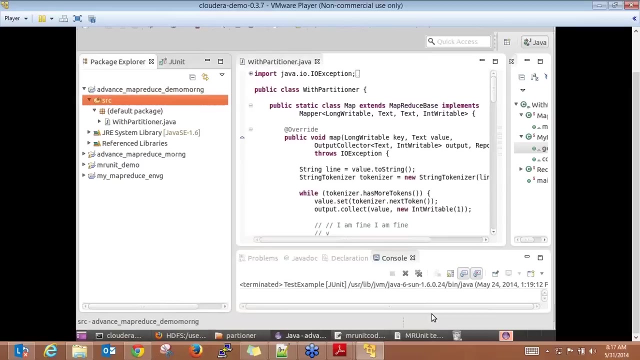 of our logic, what we have written. So the logic is very simple: We are comparing for each key And based on that key, we are going to write the value And based on that key, we are determining which particular partitioner has to be which. 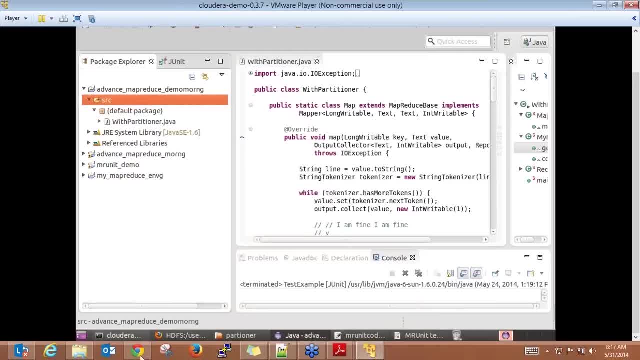 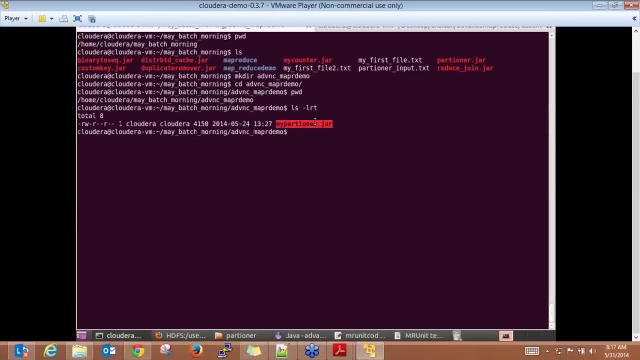 particular reducer has to process this particular key. Okay, So it sees, the jar file has been created. You do ls minus lrt, You have the mypartitionerjar. Let's create an input file also for this one, guys. So let's do gedit. 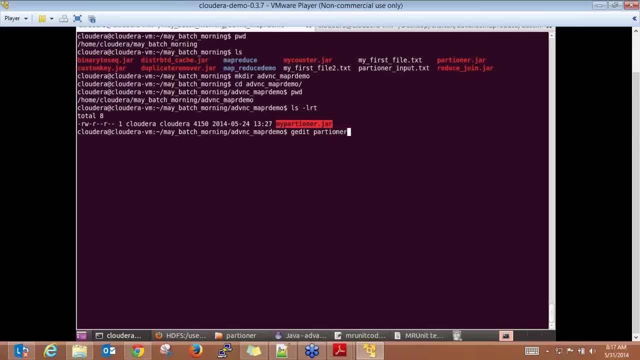 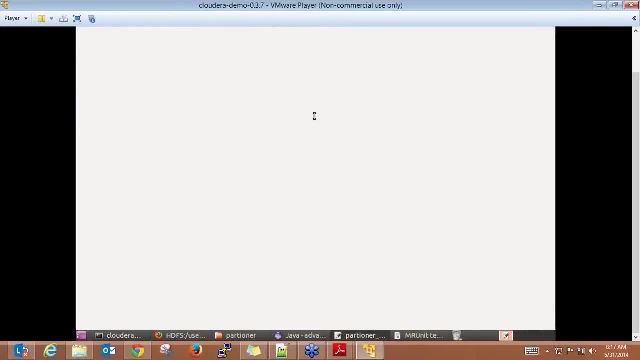 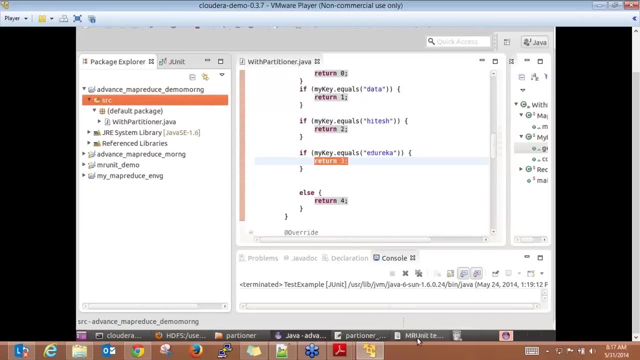 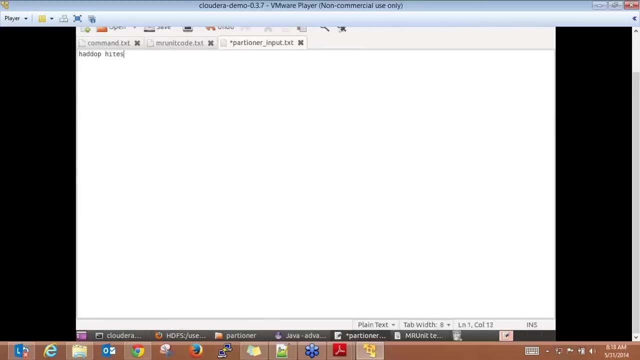 And partitioner: underscore: input, dot, txt. Okay, And here let's use some of the key words which we use, like Hadoop Data, Hitesh, Edureka and the rest of things. Okay, We have these four, And then we have something called learning others, collection, something like that way. 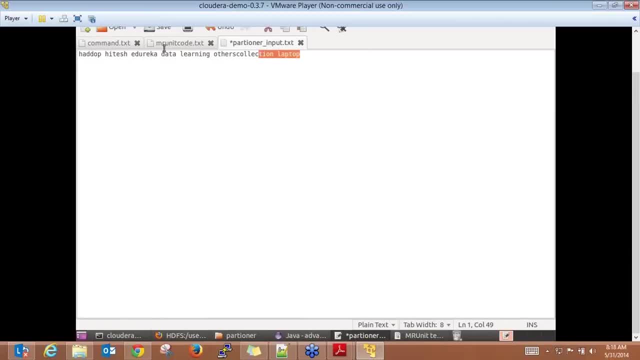 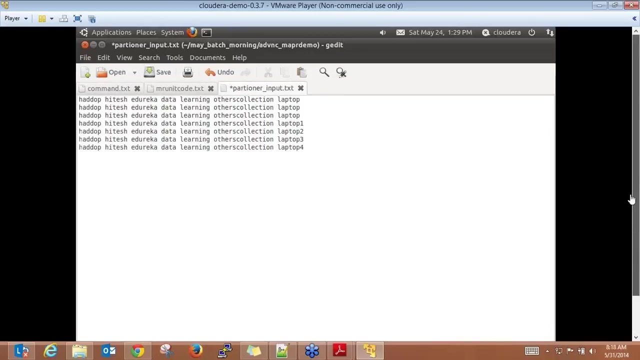 Okay, Some data set like this way. Okay, Suppose, if I do it, like all this laptop, one, two, three and four. So now, if we give this particular input data set to the process, what will happen is first, you know it is going to like take all these input data set and will mark like: 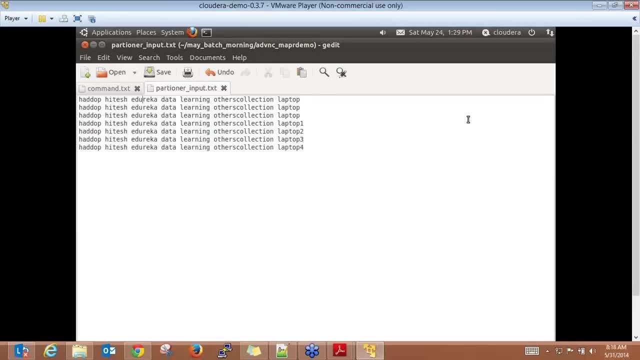 Hadoop one, Hitesh one, Edureka one is going to mark After that, since we have written the combiner, it will combine that value also and whatever the mapper input we have, it will basically get the combined output of that. 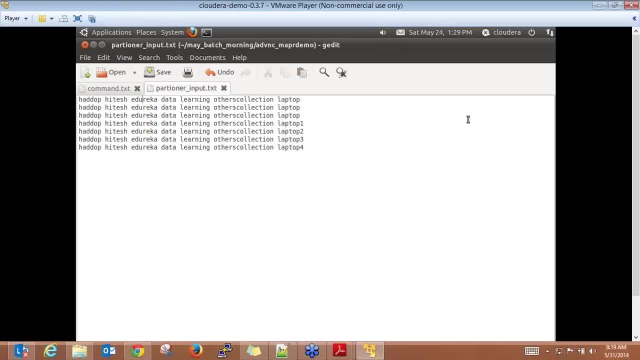 And once we have that particular thing, what we want to do is that we want to aggregation of these two, These all data has to be controlled by the logic which we have written, that is, using the partition logic which we have implemented. So, based on that, we want to make sure that all of the data goes to one particular reducer. 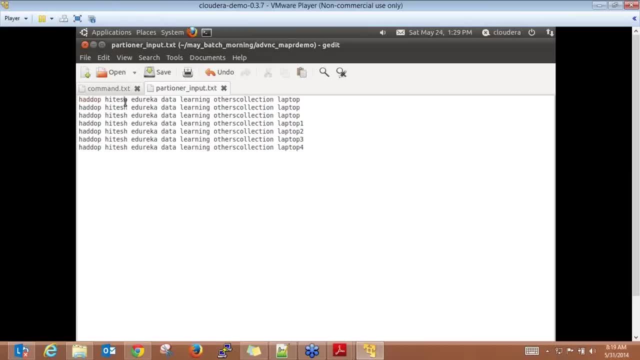 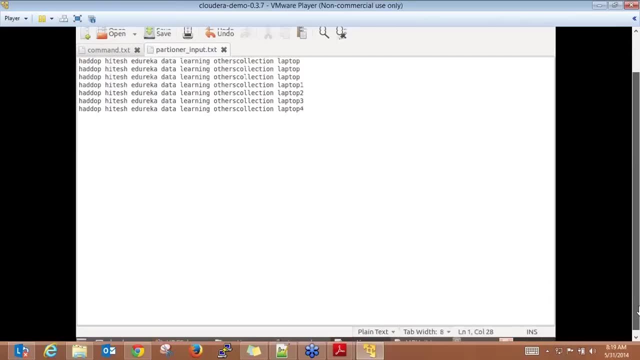 So, like Hadoop, it has to go to the Hitesh one, and you know, and like that way, like if laptop one, two, three- since we have not put any particular condition for that- So they all has to go to this. you know, the else part that the fifth reducer they 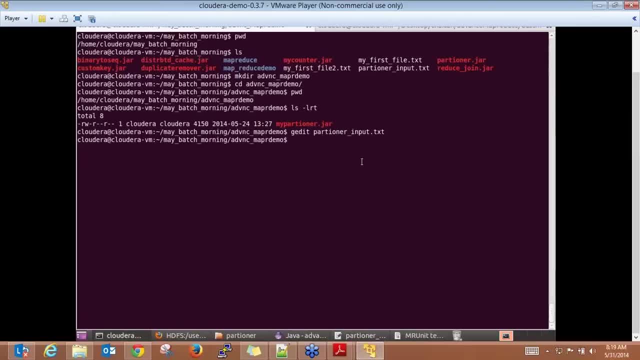 have to go there. So now let us go back and read this particular, Let us run this particular thing. So let us take it back to Hadoop fs-mkdir slash advance mapper reducer. okay, And let us move this data set. 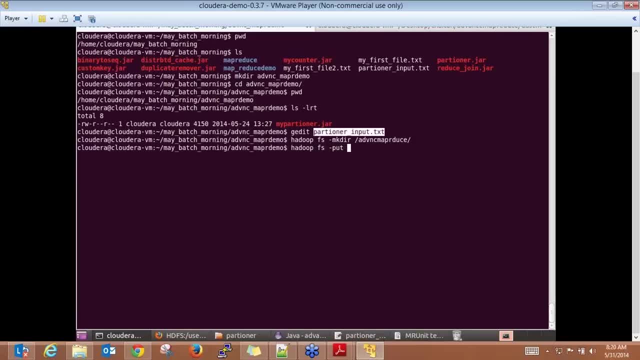 So how you move the data set? Hadoop fs-put this particular data set and move it here. okay, Now, if you want to run this jar file, guys, what is the command we have to use? So now you have the input data set. 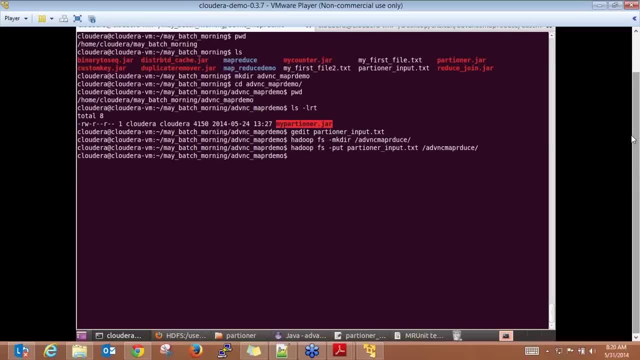 You want to run it. Of course we are going to see how the output going to come, But you know, okay. Oh, is that something? Okay, Thanks, Surya. Let me just do a quick check, Okay. 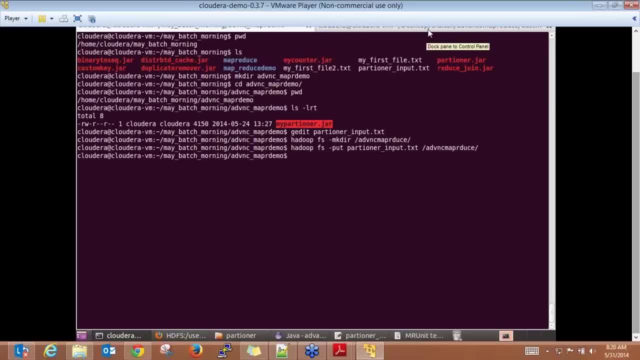 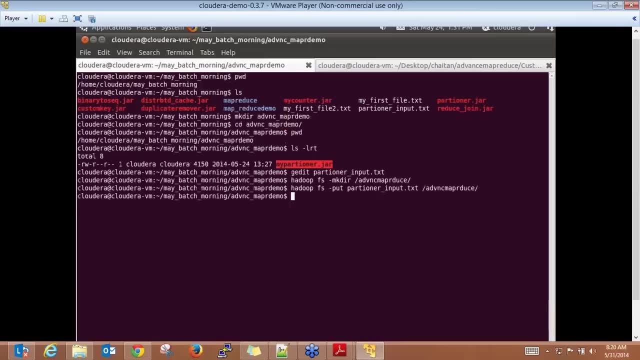 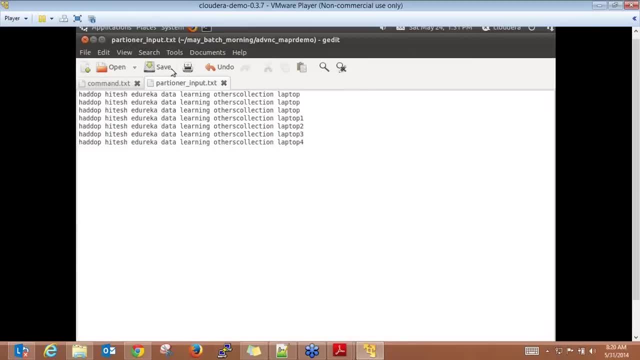 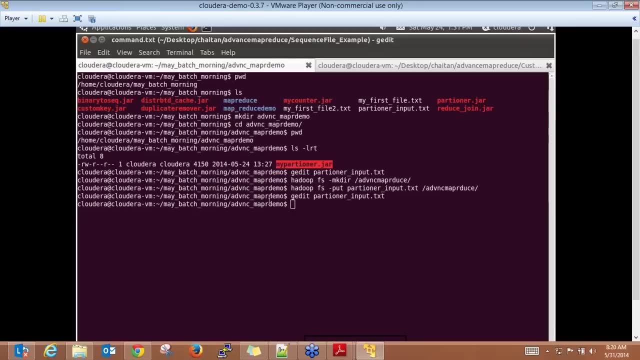 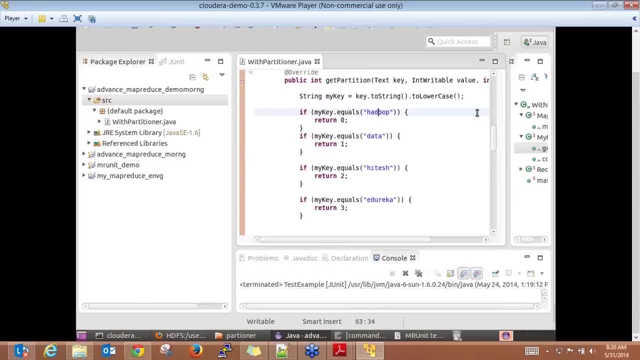 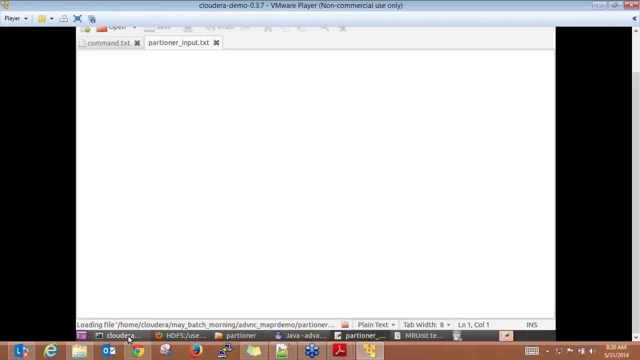 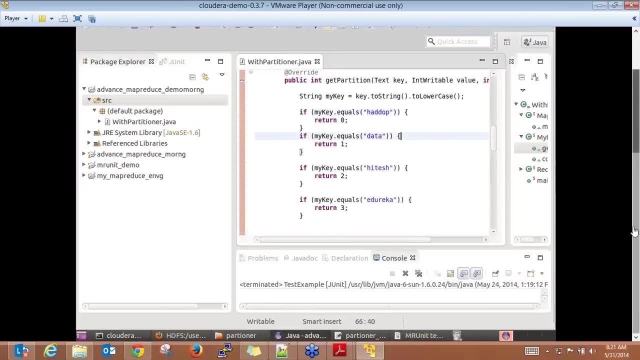 Okay. So let me just do a quick check on this. So, instead of this, what I will do is I will change the program itself. Yeah, Okay, That is what we have given. Yeah, So now, once you change this control S and just do export here. 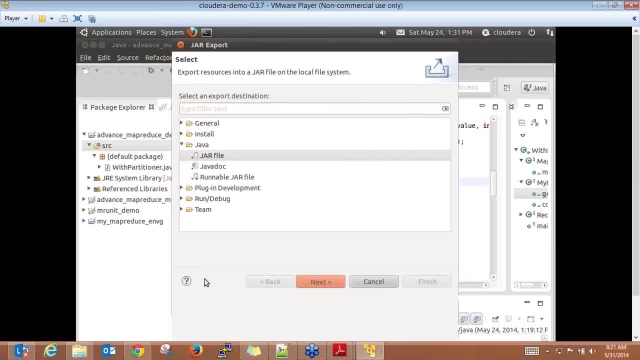 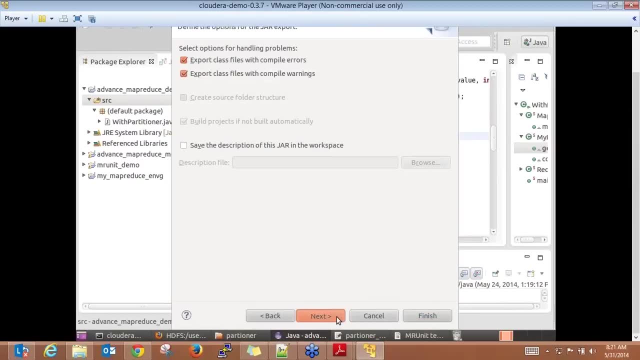 So there was a typo, guys and I say like, okay, so I just, you know, change that one. Thanks, Cecilia, okay, yeah, over-edit. okay. so now, if you want to run this one, how you? 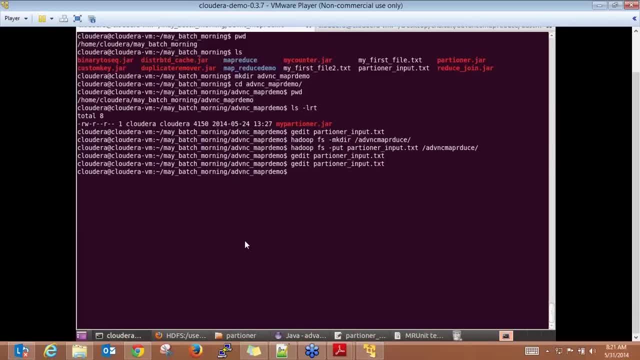 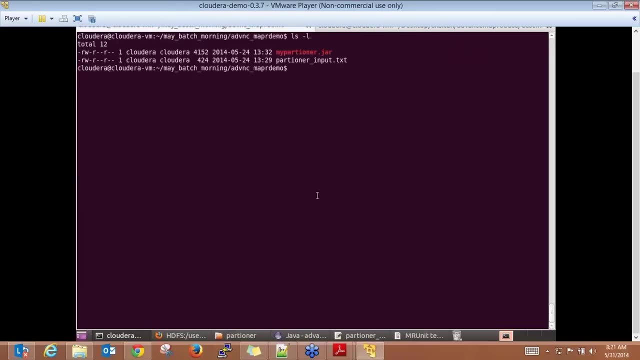 do that? What is the command, guys, to run this particular thing? Okay, so the command which you want to run it, you know, it's simple. All you have is, you know, the jar file you have and the input data set. that is already. 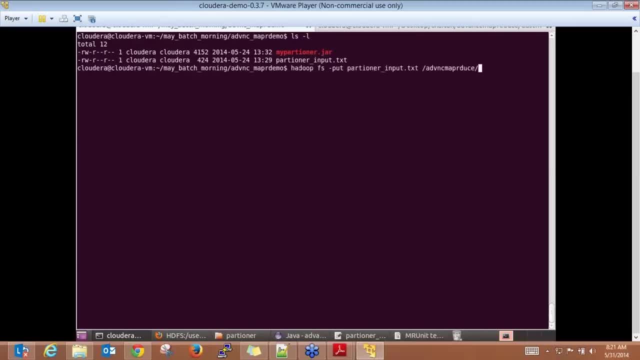 available. We have moved this data set, you know, into this particular location inside the Hadoop. So now, if you want to, you know, run this: it is Hadoop jar- and give this particular jar file name- So this is the jar file name- and give the input data file which you want to process. 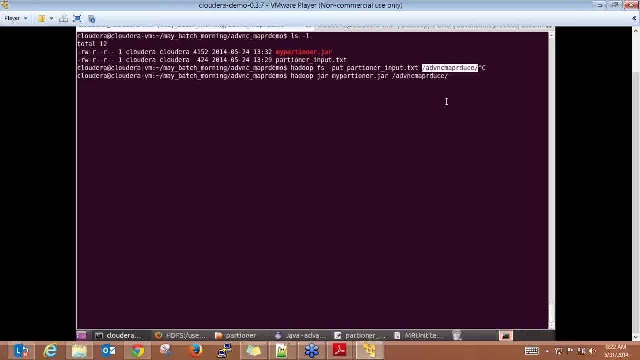 so it is like advanced MapReduce and inside that we have the partitioner one and it's going to consider all the data set and then output. we are going advanced, right, and then you are going to have this advanced MapReduce slash partitioner output. okay. 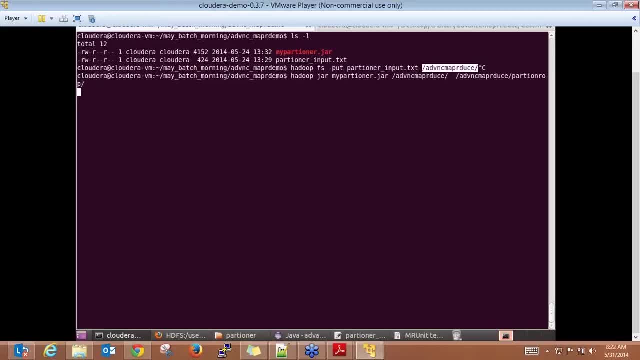 That's what the data we want to store. it okay. You hit enter, Okay, That's it Okay. So how many partitioner we are expecting here, guys? How many output file are we expecting here to come as part of this program? output of. 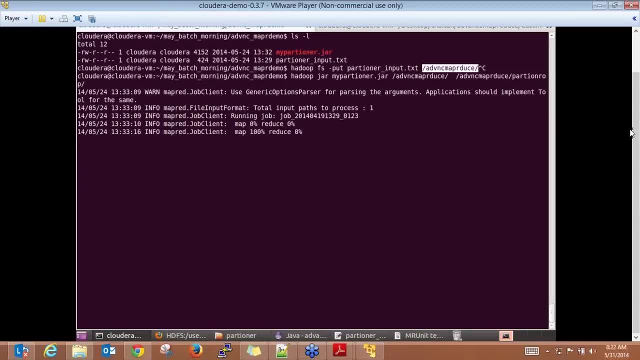 this program. So this is three, okay, How about other people? One, five, So how many? number of the reducer we set, those may number of the output file we are expecting, right, Okay? So Ashish Swagata, okay, I get it. 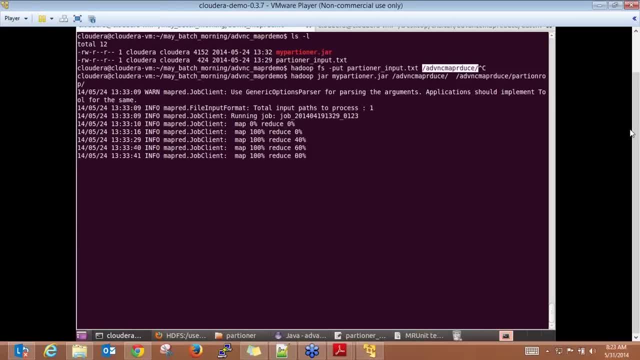 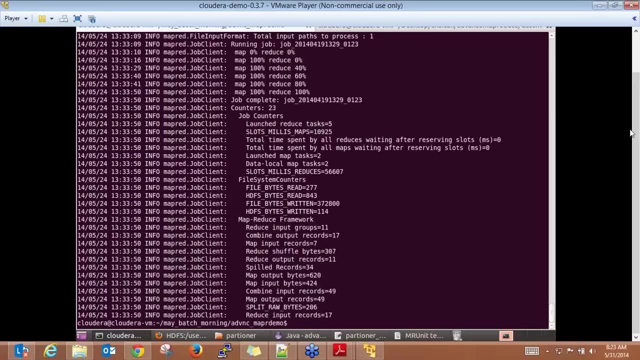 Okay, Devinder And Hitesh and Meg help me to understand, like: why do you see it will be either one, three kind of things, right? Why do you think it will be one or three? Okay, Satish says three into three copy in the distributed computing. 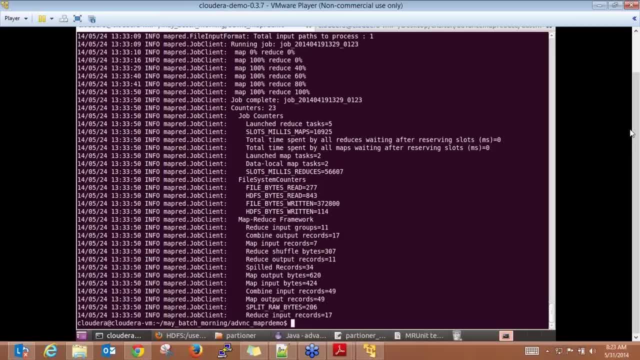 Okay, So that is Satish, like in the storage part. Okay, So my question was on the you know. okay, so first Satish, why first three? right, Okay, I got your the other thought process like you told that. okay, the three copies three. 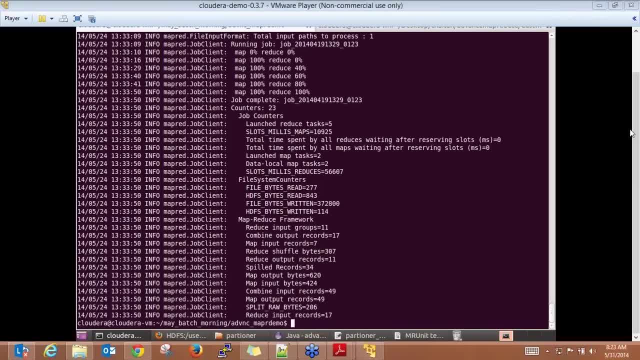 data set will be multiplied across three different nodes, so you will have those many copies, But how come you the first three, how you are determining that it will have only the three output? Yeah, So so, guys, when I'm talking the number of the reducer, it's not by default three. 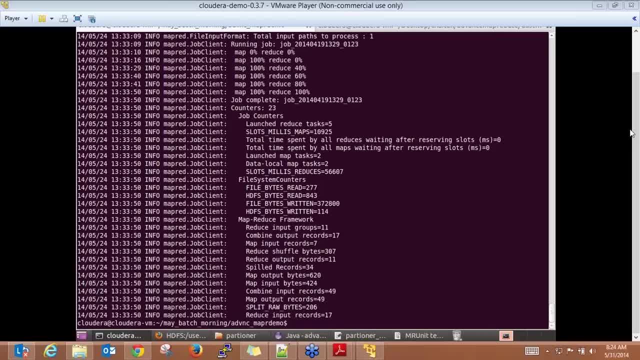 This is something you can configure it. By default, it is set as one. If you don't specify, there will be one single reducer, it will run right After that. you know the number of the output which you are going to get. it will be determined. 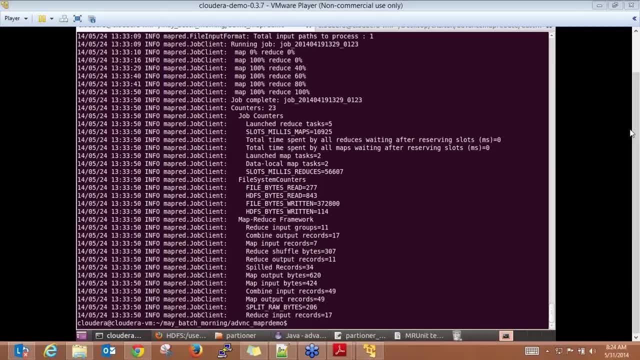 you know, based on the number of the reducer, you set it. Okay, Yeah, So it is five. Satish, Yes, you got it now. Yeah, And Hitesh. why do you think that it is going to be only one output file? 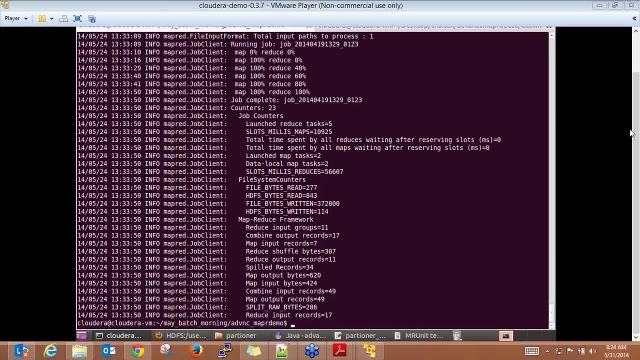 Okay, There will be only one for the total aggregated value. If we have ten reducers, we are going to have only one output file. Okay, So it is going to have the ten files. Yes, it is So. if you are having ten, then it is going to have the ten files. 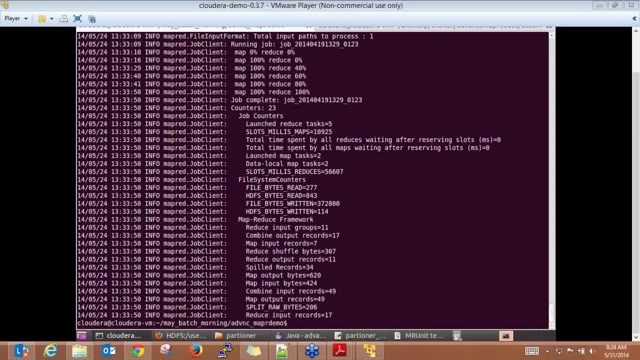 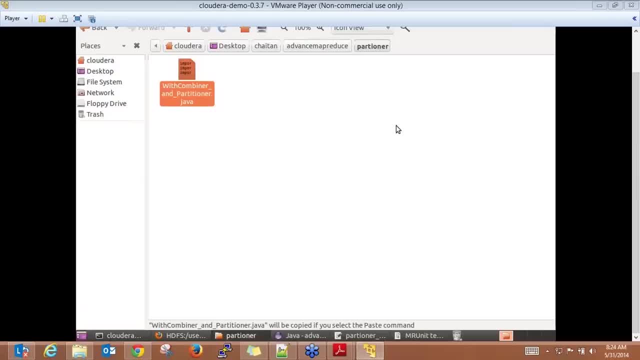 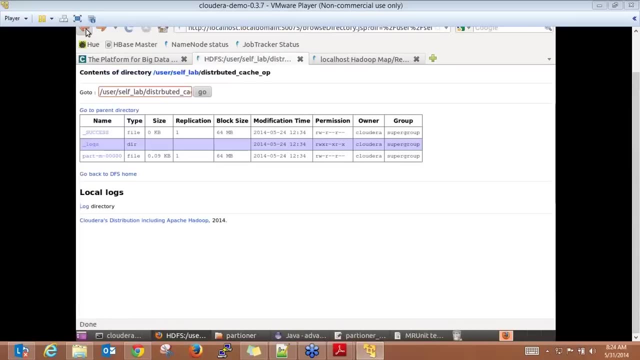 Yes, Okay, So it looks like the program ran successfully. Okay, Now let's go and see that. So where do you see this? You go to the name node here and you go back and you just try to list everything. 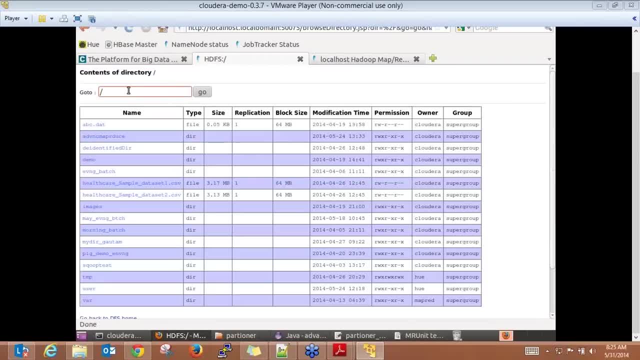 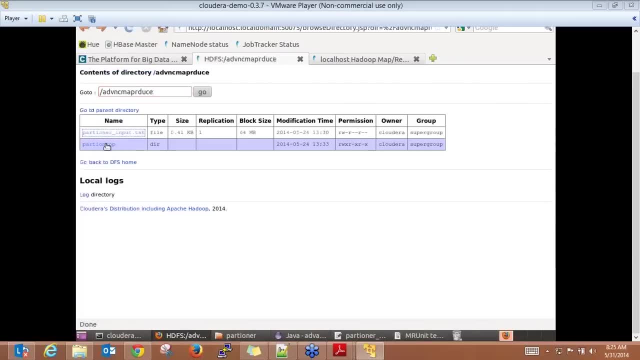 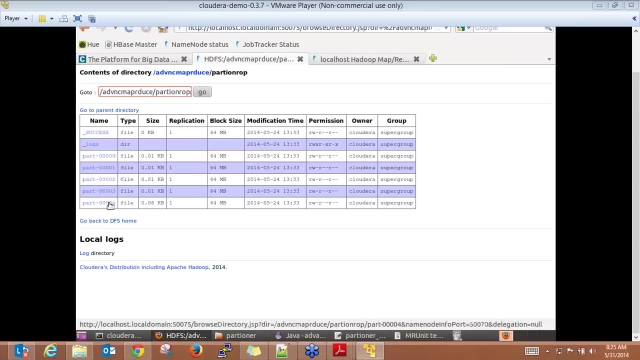 Okay, So we have this advanced MapReduce and then we input file we provided. This is the input file which we provided and this is the partition output. we have. How many files we got it here, guys? You see here: Zero, one, two, three, four. 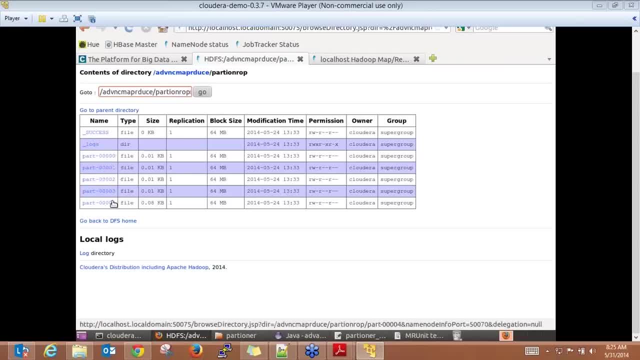 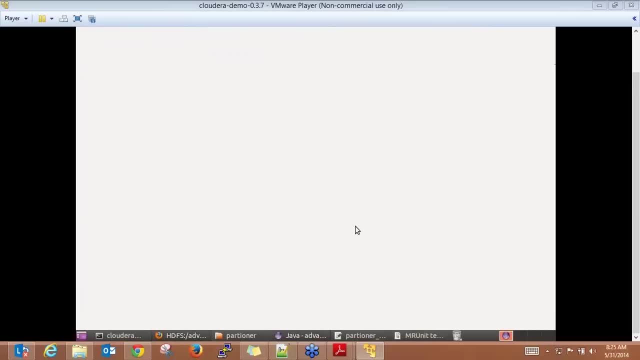 How many partition file. we have got it Four, Right. So that's what we wanted. We wanted to divide all this data into four. And what is the logic we have put here for the partition? The first part is the first. you know the reducer. it should process only the value. 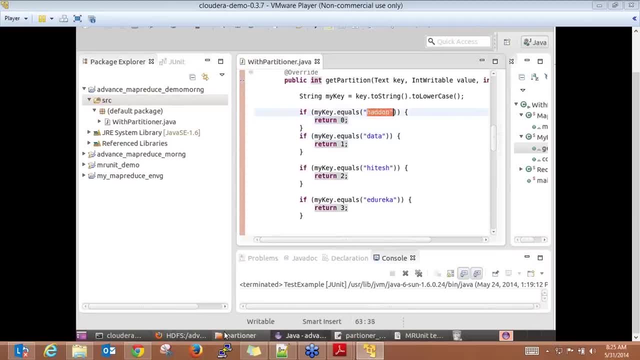 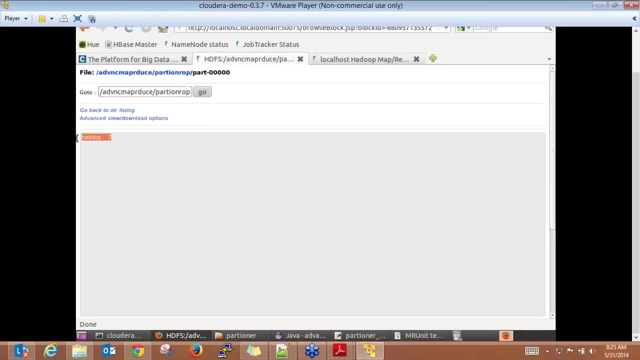 which are for this particular key called Hadoop. Okay, So let's see that. What is the output here? You see here This output file: we are getting only Hadoop, that it has come seven times. What is the second one we have? 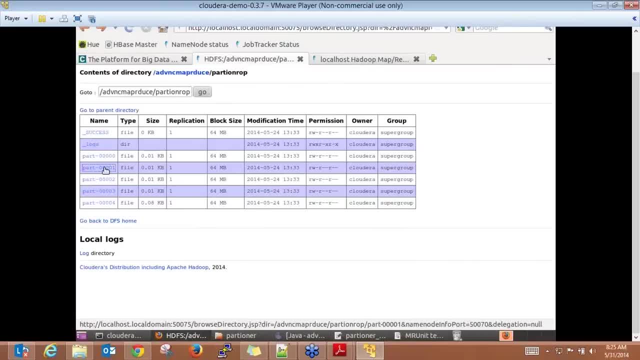 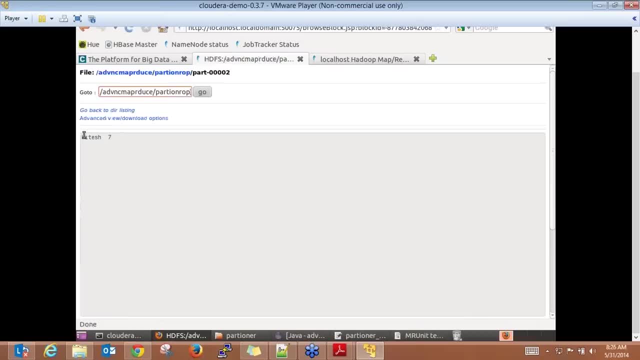 That is like data, Right. So it has just counted the data. The rest of the key it has just ignored. Similarly, if you come back here, The third one, it has just counted for how many times the Hitesh and that's the output. 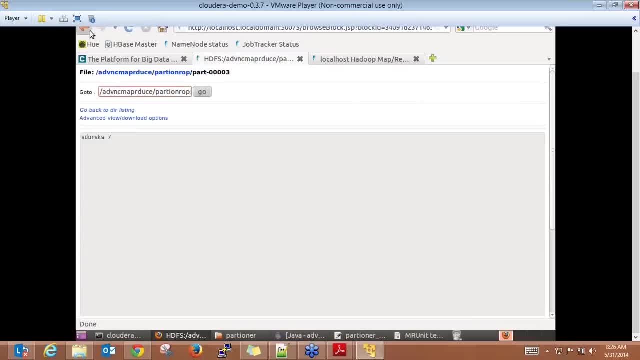 we have. The last one is for Eureka. Again, it has counted The rest of the things like all these. you know one, two, three, what we did for this data set. all those went to the default reducer. 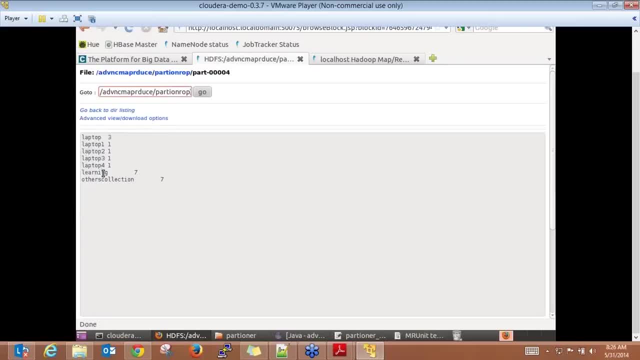 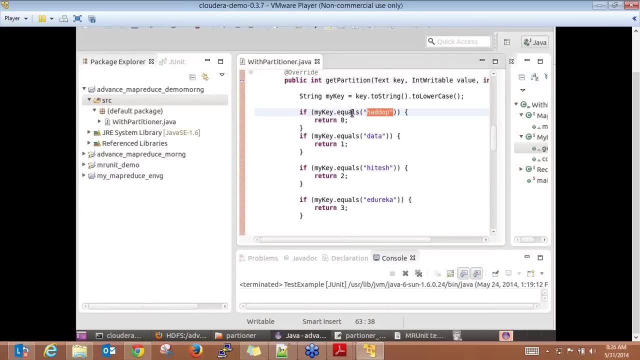 That is the fifth reducer which we have And you have like laptop, three times one, two. all those things are counted by the default reducer. So this way, what you are doing is by writing this particular logic, you are basically controlling how your output data is going to be moved from a mapper to which reducer. 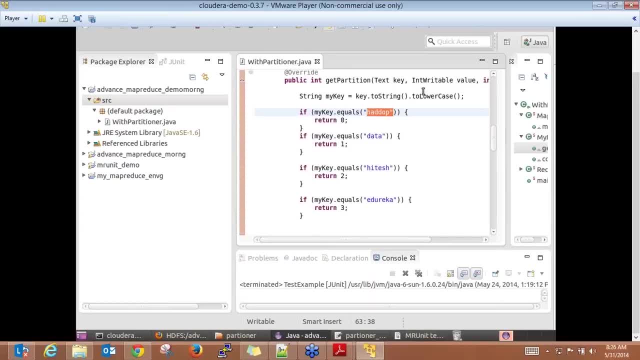 And, based on that, the aggregation will happen and your output will be stored in that particular reducer output file. Okay, So is this clear guys? Are you guys able to see that the partitioner, by using the partitioner, you are able to? 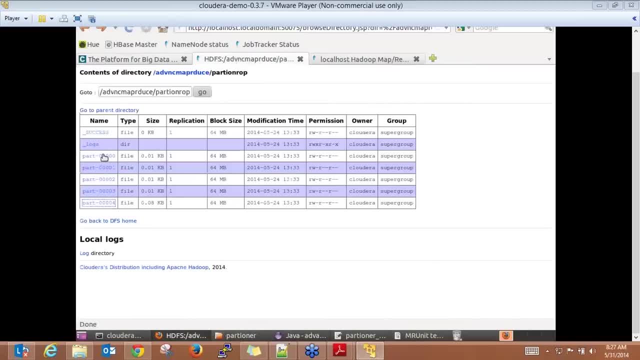 basically control how the output file is going to contain which particular. but now you think of your. this is one example you think of like: suppose, if you are computing multiple transactional data and you want to segregate that, okay, the company one you want to put. 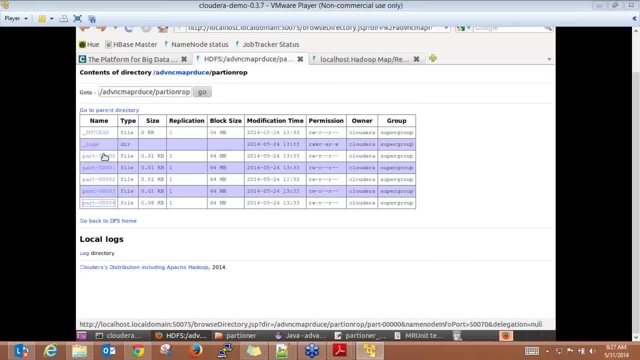 it one or you know, for a particular G or for a particular cluster. I want to put in all Now, all those things you have to put all only the filter and the key, and once you implement that you know filter as a partitioner, your all the data set will come together as one. 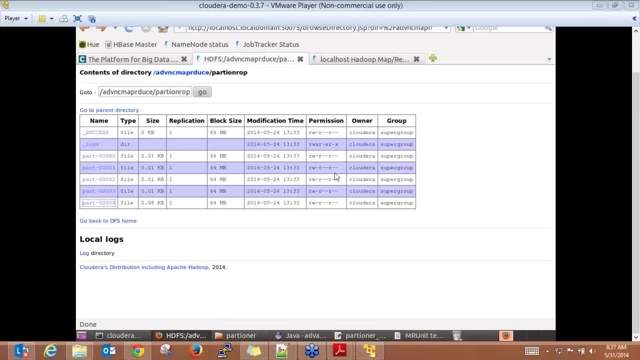 particular thing. Okay, Minus is clear. How about other people? Is everybody clear with this particular example guys, Can I get a go that? are you guys good with the partitioner and, in the overall logic, how to, how it works, how the file you will be able to control? 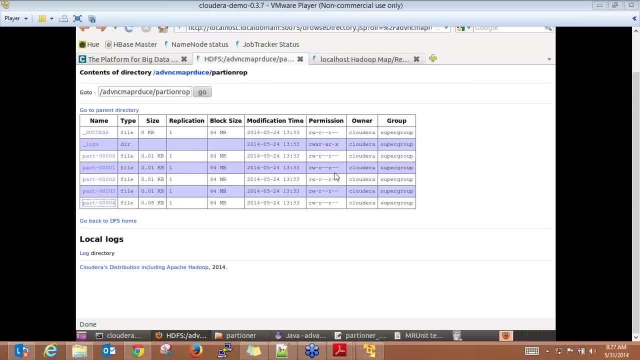 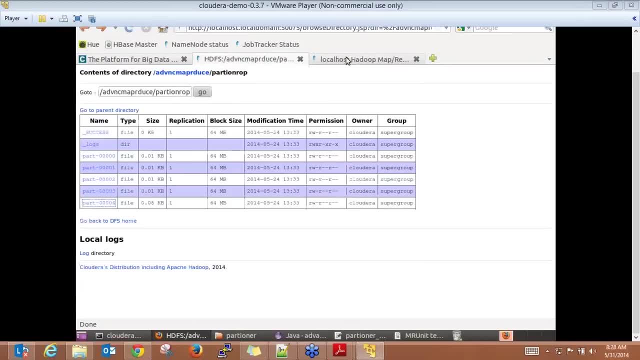 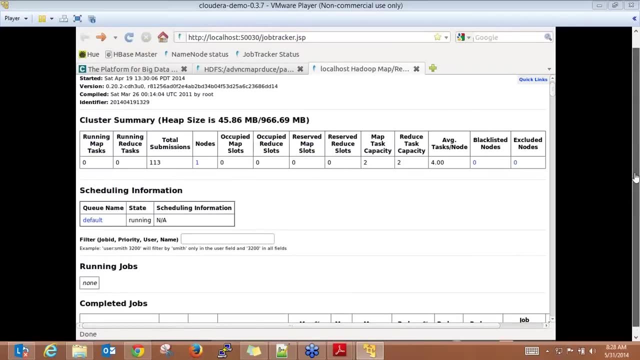 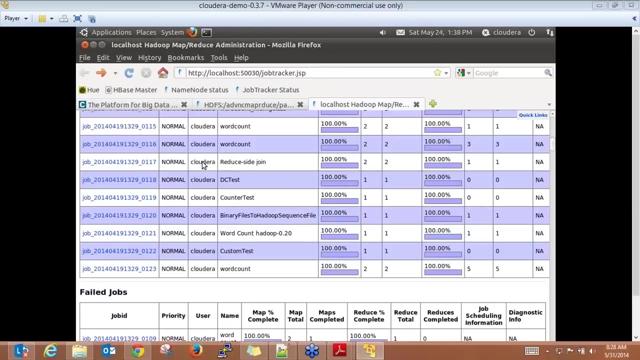 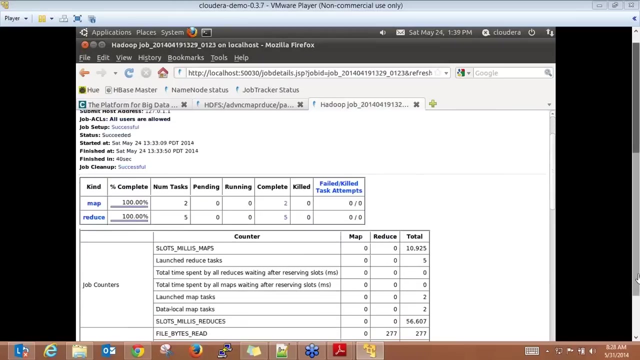 So now let's go to the job tracker here, guys, And let's see the job which I just know it to run. Okay, So, Okay, Okay, who had this question? let me, okay, I'm just so I'm going to your question, okay. 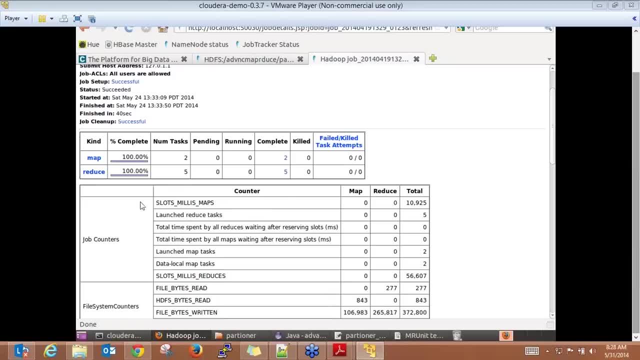 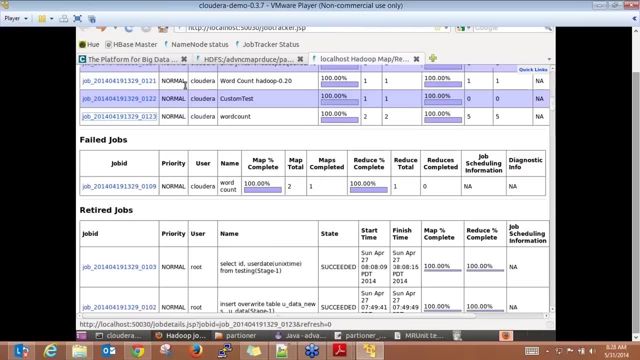 so so I had a question right. who had this question? hello, yeah, you, only right. so how the number of reduce are going to work right. so in a server, right when you go, if you come back here, you can see on this particular machine how many number of the map tasks and the reduce task is capacity is available. so the map task. 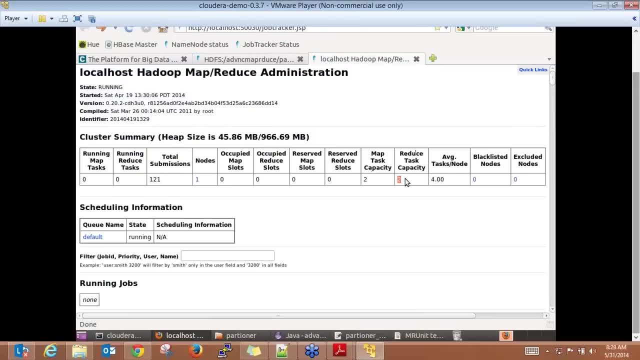 capacity is 2 and the reduce task capacity is 2, so what means in this particular no machine we can run the 2 reducer and the 2 mapper simultaneously. now what if? if I want to run 5 reducer, it doesn't mean that all the reducer 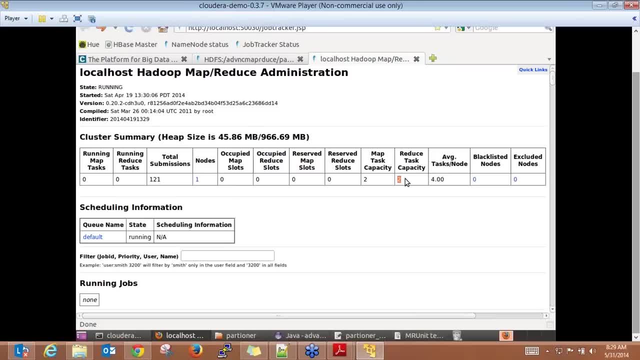 will not turn, it will run. but only thing is, since we have the two tasks capacity, only two can run at a same time. so rest of the three, it will be on the queue and once these two slots are complete, then the rest of the three will execute right. 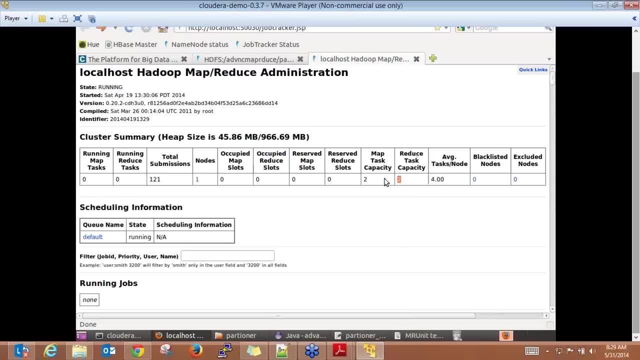 so that's the way the, the, you know it's going to work on this particular thing, right? so that's the way it's going to work on this particular thing, right? so that's the way it's going to work on this particular thing, right? so now suppose, 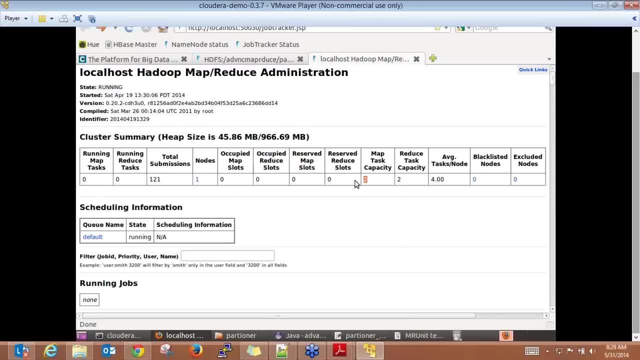 our data set is such a way that it know it need five mappers to process that. input it as a- so in that way smart weapon to really start simultaneously and the rest of the three it will start after that to slot becomes reliable and that's where the bigger cluster comes in the picture. so if you have more number, 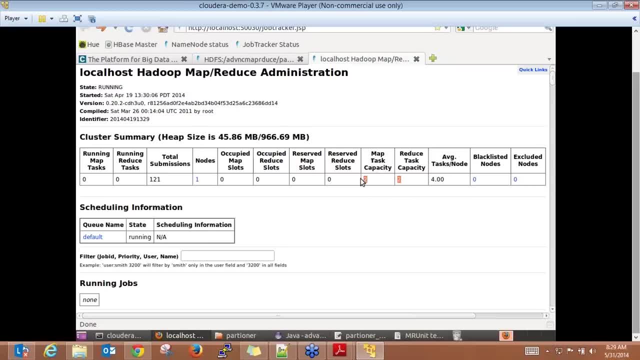 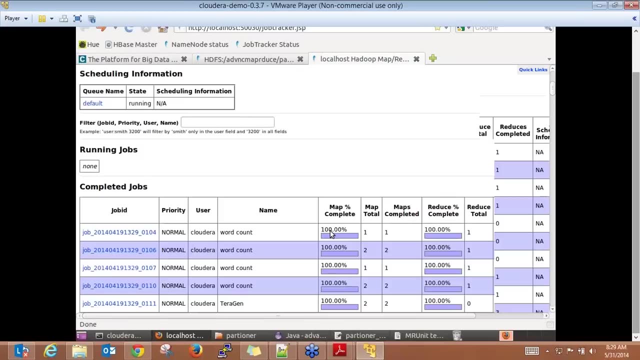 of the map task capacity. reduce task capacity. you can run more jobs in parallel. okay, so that's one part to answer your questions, Agatha, about the how the slots are there right now. come back to to the. So in this case you see how many number of the mapper we ran- 2- and how many reducer we. 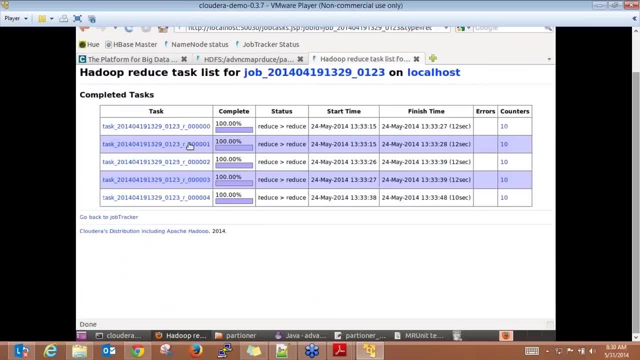 ran. We ran 5 reducer right. So each of the reducer it got like 1: 1 input data set based on the logic which we wrote and based on that logic it basically processed all this data and we got the output right. 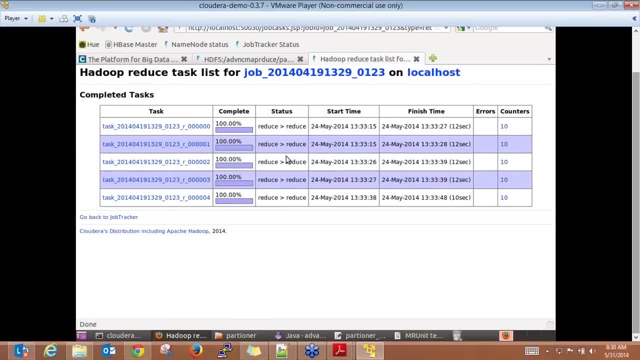 So this way, the 5 reducer we were able to run by using the 2 reduce slots which is there in the cluster. Does that answer your questions, Agatha, in terms of how things works on this particular machine? Okay, is there anywhere we can see the number of the task tracker involved? 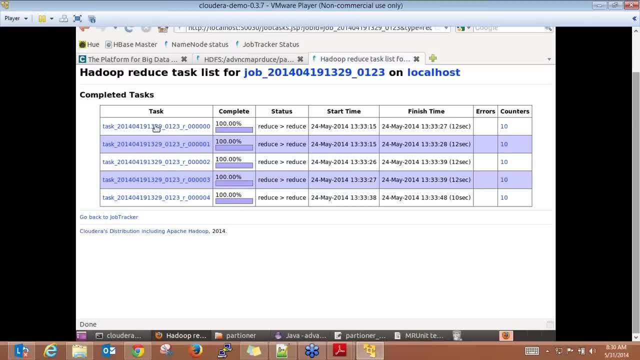 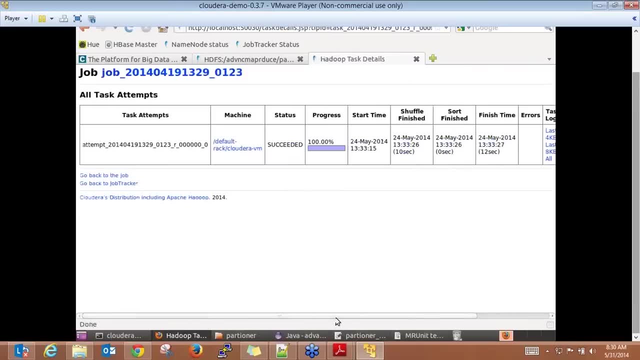 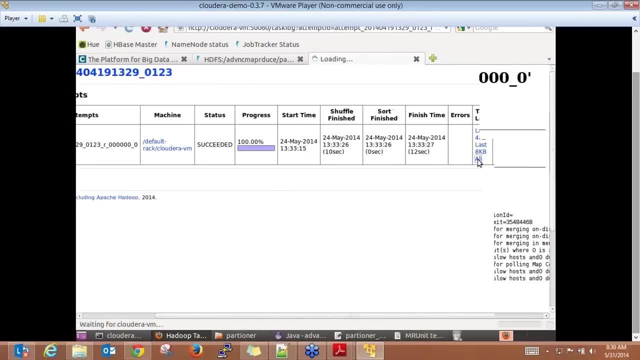 Yeah, you can see this here. So all those things are available in the job tracker. So you see here the task. yeah, so this task tracker, you can see if there is any output error message, You can see all this. all right, So you will be able to see all this standard out, standard out logs, everything you will. 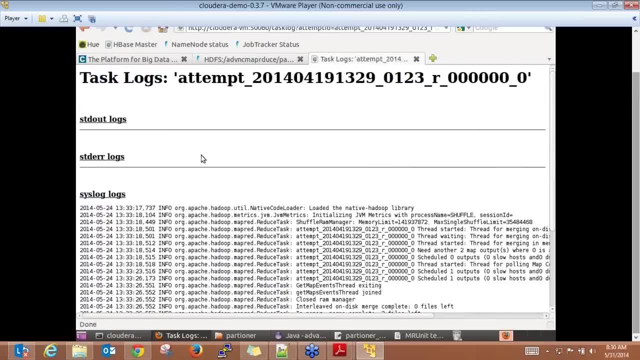 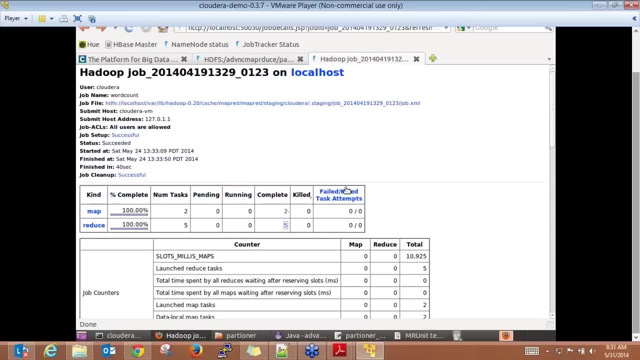 be able to see here, right? So when the job fails, guys, this will be the link which will come. so this is the job tracker. You will come and you will see here. when the job will fail, it will say that how many job has failed, failed and killed task and you will click that. and once you click that, you 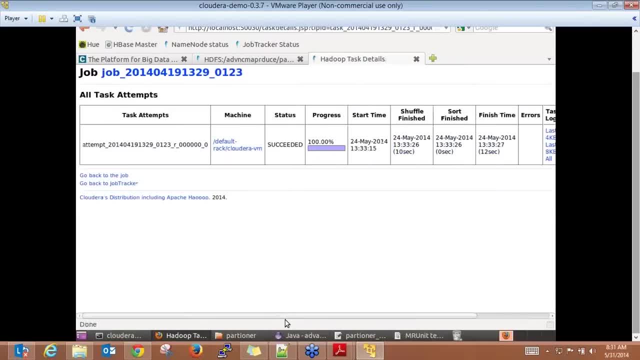 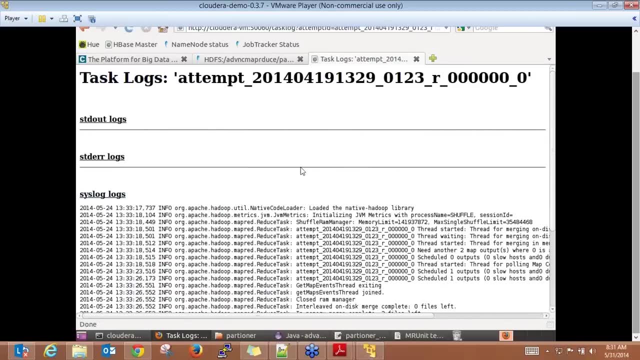 will basically go this particular thing- task tracker. You will click the task tracker and then you will go to the. you know the task logs and you will click the task log and see what are the error messages it is having. okay, In the output UI block size is 64 MB, but the data store is only few KBs. 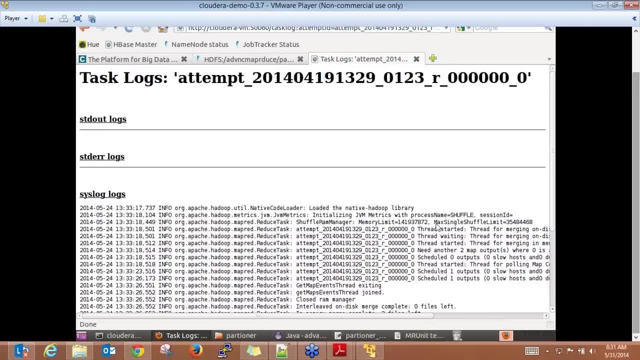 Yeah, so actual data, Vivek. it will be like few KB, but the block size is 64 MB. that's what it is showing, that okay, Okay. So So I think, apart from the Hitesh doubt, I'm not sure it's clear. 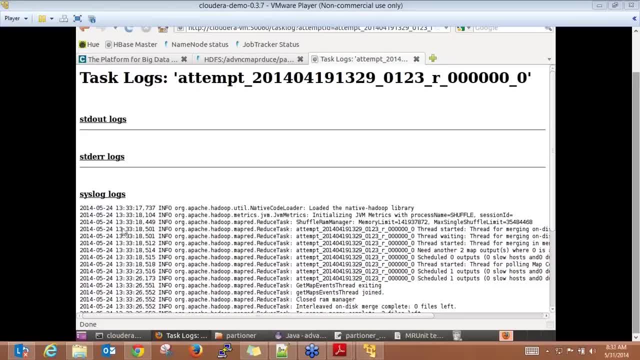 So Hitesh your doubt with having only one reducer. is it clear now that since we specified the number of reducer, 5, that's what we have: the total output file at the 5, not as a 1.. And okay, so that's all we have. okay. 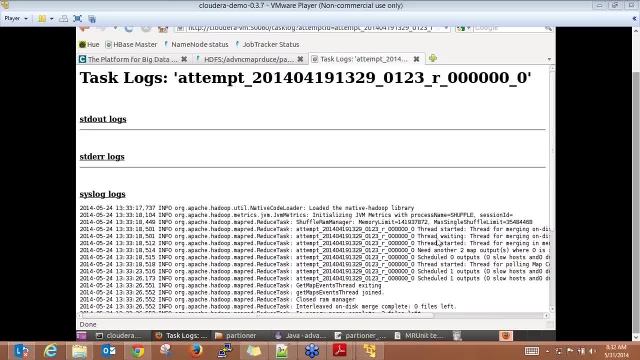 Yeah, and Hitesh. the number of the input split is equal to the number of the map task. if you limit the map task, are we not limiting the? We don't limit, Hitesh, the map task. so that's something you can limit. how many number of? 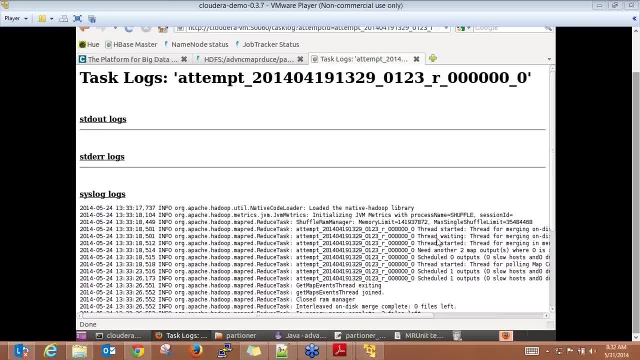 the reducer you want to run in the cluster, but the number of the mappers you cannot limit it. that will be basically decided by the framework in terms of how many blocks or how many split you have for your input data. So that's why that's way it is going to determine how many number of mapper it's going to run. 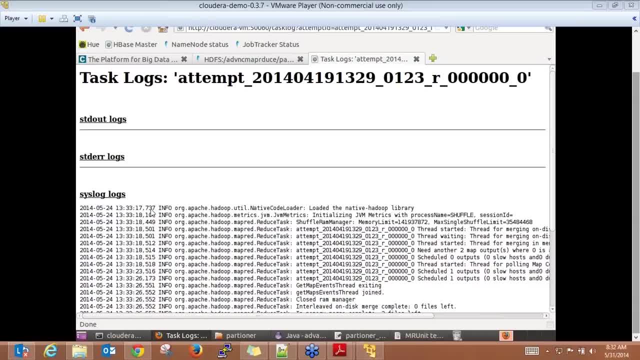 Okay, Okay, Okay. so let's go. Vivek says: what if the output is more than output is more than 64 or 128MB? So that file will get divided, Vivek, into the different blocks, and each of the blocks will get stored inside. 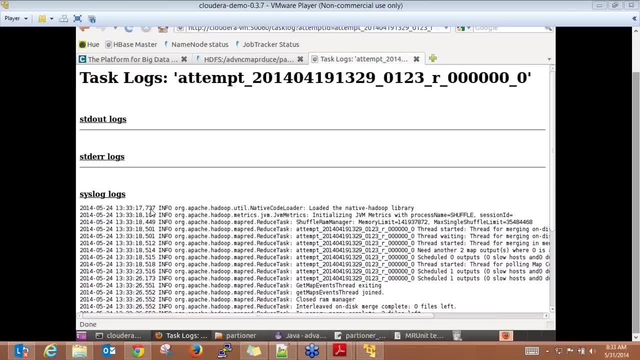 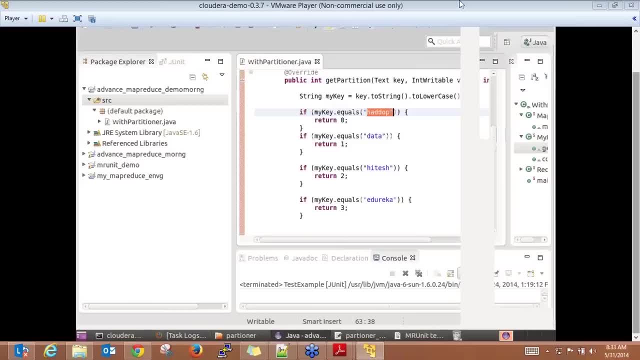 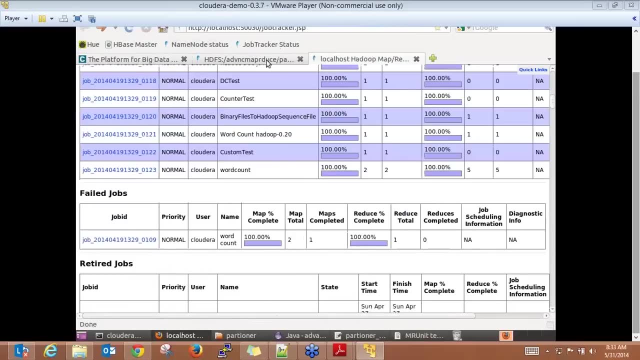 You know the different machines. but whole file you can refer is still by the single namespace, by using. you know this particular thing. Let me show you here, If I go back here. So part 0, right, So this file internally it can have, like you know, like currently. 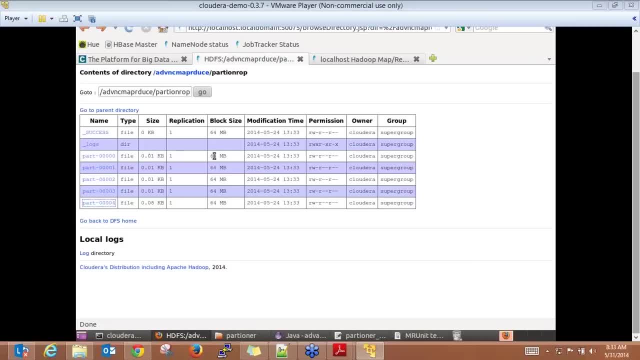 we have 0.01 KB kind of the size, Like, suppose if it becomes like 128 MB. So this file internally will have two different blocks which will make this file, but you as a- you know when you will access- you will access with the same file name. Internally we'll divide into: 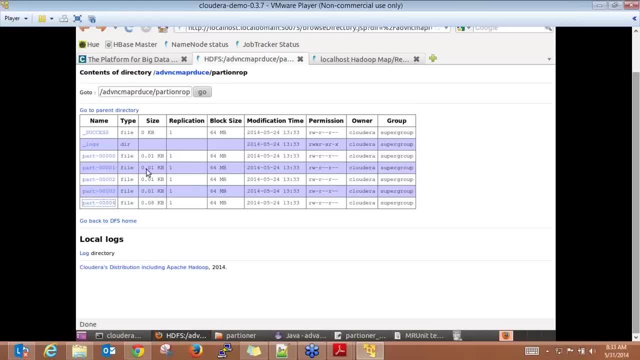 blocks and that's where it will be stored. Okay, but that will be something transparent to you Here. the block size you will see like 64 MB, but the actual size it may have like 128 MB or something like that. You will see it here but you will be able to access. 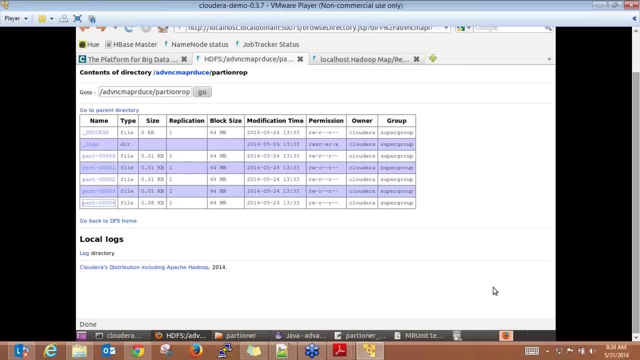 by using the same space. Okay, Can we specify number of my pass? No, you cannot. Okay, You got it, Vivek. Okay, Okay, cool, This is clear now. Okay, Is everybody clear by this concept? guys, Are you able to see the partitioner? everything? 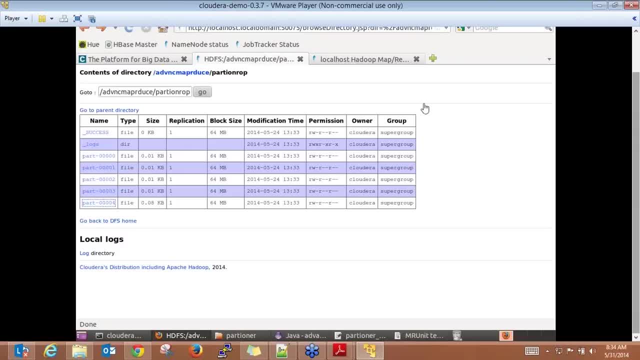 how it works. right. I know you have to practice it once, but you understood the whole flow, how you work and what the partitioner is doing. It's basically segregating your output into the way, whatever you want to put the logic. based on that logic, It's outputting.